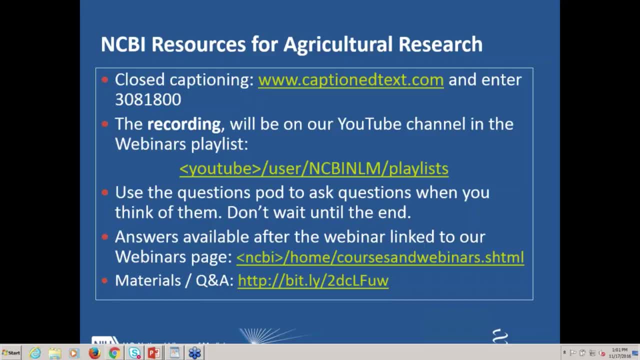 Matten, So they can answer some basic questions in there while we're going along And then at the end, if there's time, we can answer some more substantive questions. If we get questions, they're going to be available linked to our webinars page along with the link. 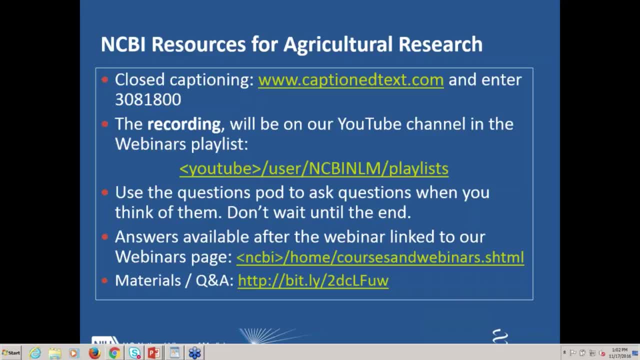 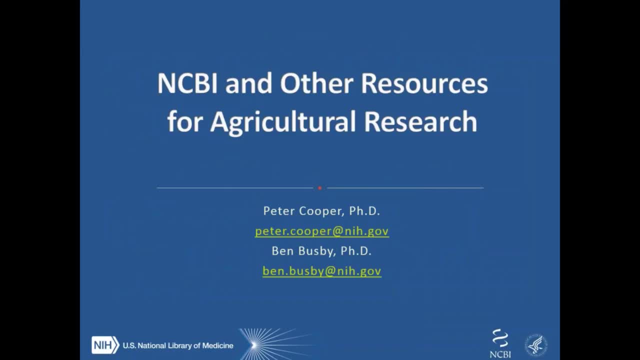 to the YouTube channel. The materials for this talk are on our FTP site and that compressed URL will lead you to that FTP site. So there are two people presenting there. We're in sort of not in any particular order except chronological. I'm going to go first. I'm 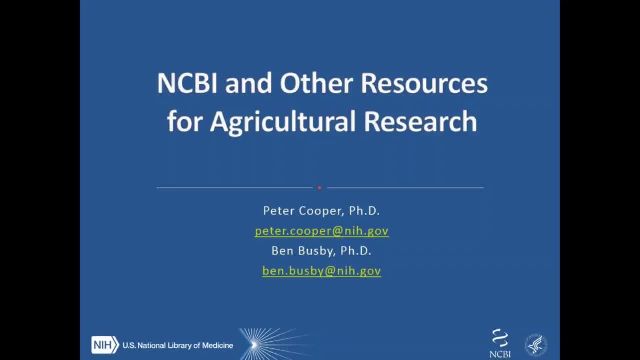 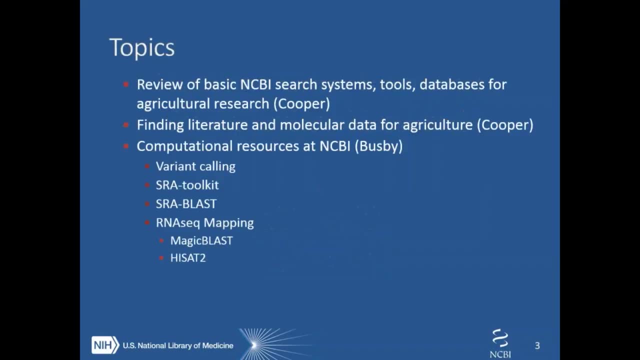 Peter Cooper, I'm with the education group here at NCBI And then Ben's going to talk. He is the genomic researcher, He's the outreach coordinator at NCBI, And so basically, what we're going to do is talk about the basic search systems at NCBI, tools and databases that are for everything but 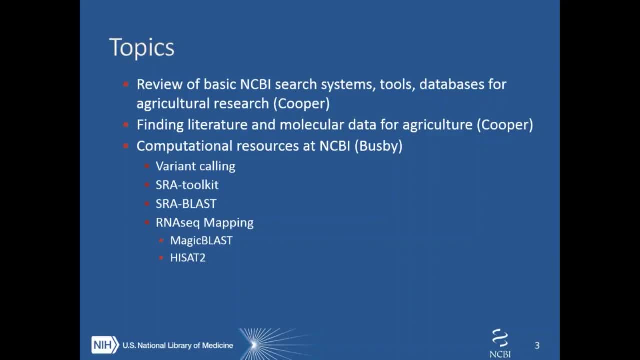 we're going to focus on agriculturally relevant organisms And then I'm going to do a demo on the web using some examples from cow and using an example from a plant, linking across a bunch of the different NCBI databases. Then Ben is going to take over and he's going 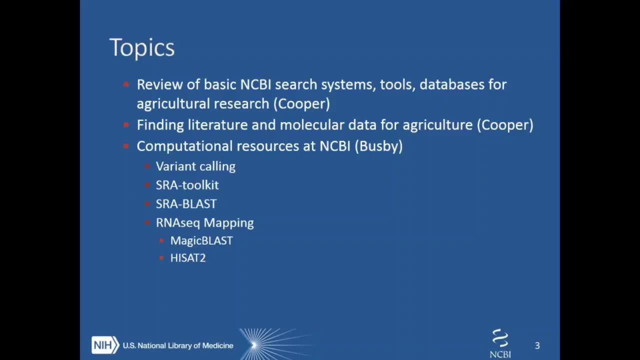 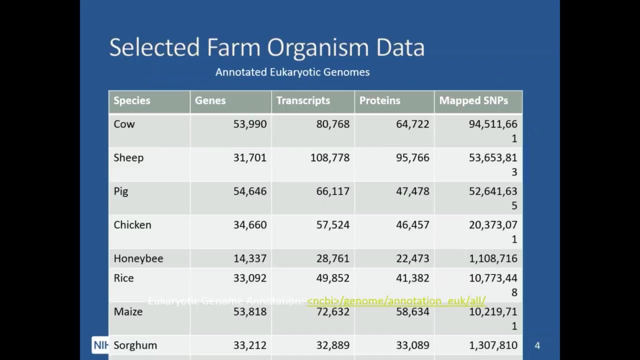 to talk about more bioinformatics types of research, And then I'm going to go ahead and show you a little bit more about the resources that are available. So we're going to look at the themes that he's going to talk about. So just before we begin, I wanted to show you a slide, which didn't format very well when 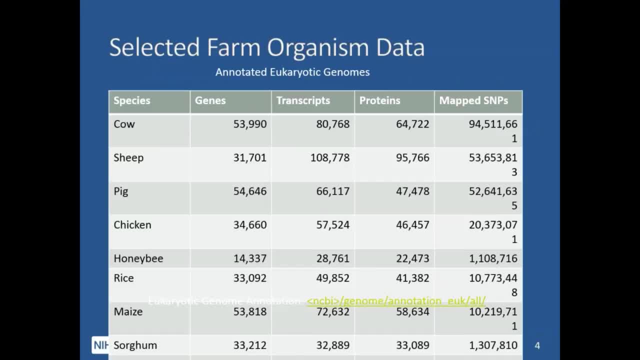 I crossed the platforms here Essentially just to make you aware that we have a lot of data available for organisms that are not strictly human. These are some agriculturally important organisms: Cow, sheep, pig, chicken, honeybee rice and so forth. And then I'm 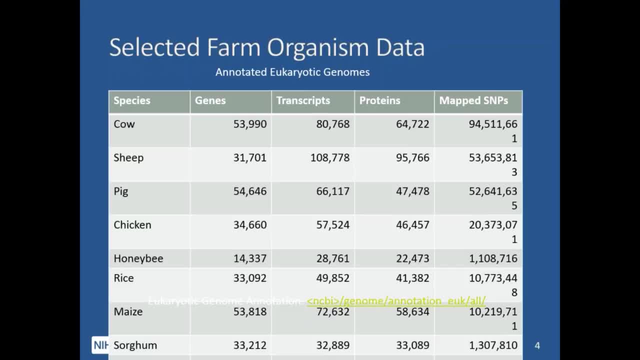 going to go ahead and talk about some of the other items that are available, So I'm going. maize, sorghum: we have completely annotated genomes for these organisms. we have genes, transcripts, proteins and map snips available for each one of these. this is just a selected set. 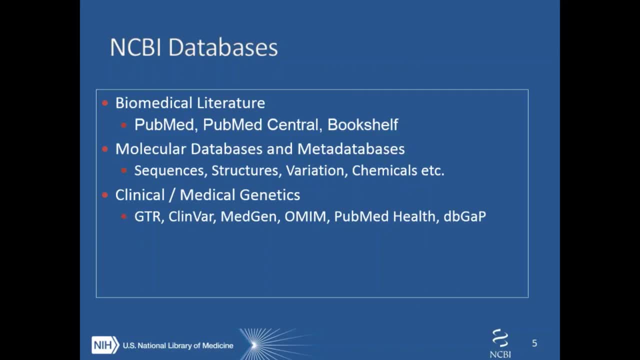 there are others where we also have a lot of data, and so when we're looking at data at ncbi, it's useful, i think, to think about three different sets for aspects of the data. there's biomedical literature. that's our pubmed resource. there's also the full text pubmed central and our full text. 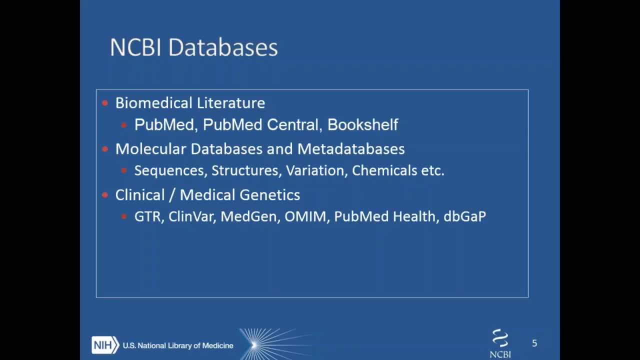 online bookshelf, then their molecular databases, which are the ones that i'm going to focus on today. they have things like sequences and structures and variation, and even chemicals, if you want, and then the last set are things that have to do with clinical and medical genetics, and 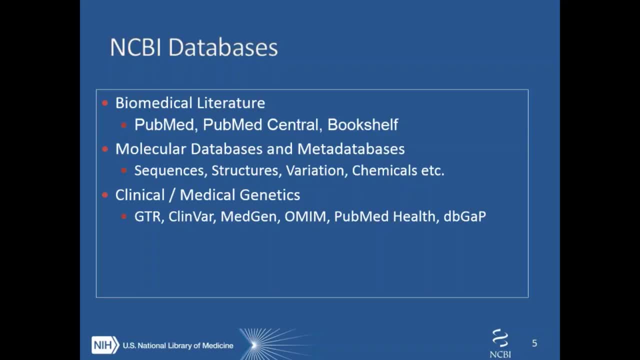 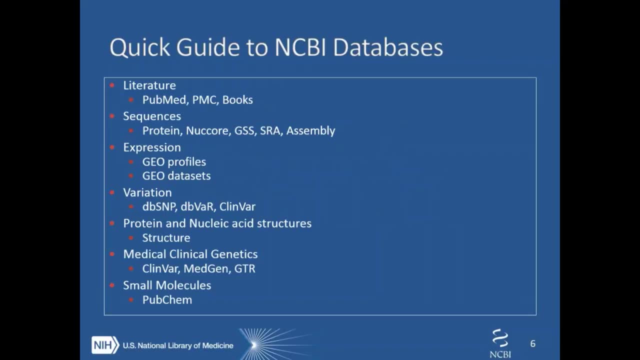 those are focused exclusively on human health and disease, not on animals or plants. if we want to break them down a little bit more, you can sort of break them down into these categories: literature sequences, expression variation, protein nucleic acid structure and then the clinical genetics things that we talked about a minute ago. we're going to visit. 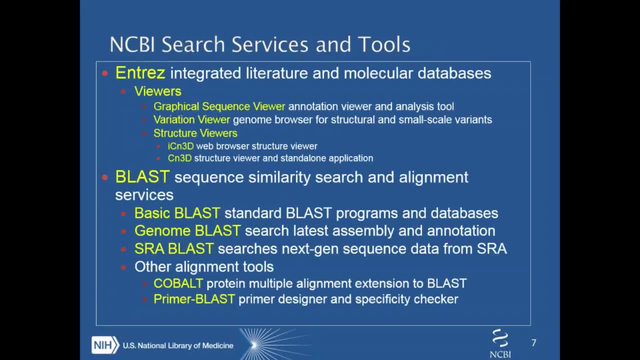 a lot of these molecular databases today. so the way we're going to do that is we're going to use some search services and tools. there are two main ones. there's entre, which is the general tech search system. that also includes these databases. that will let you see records associated. 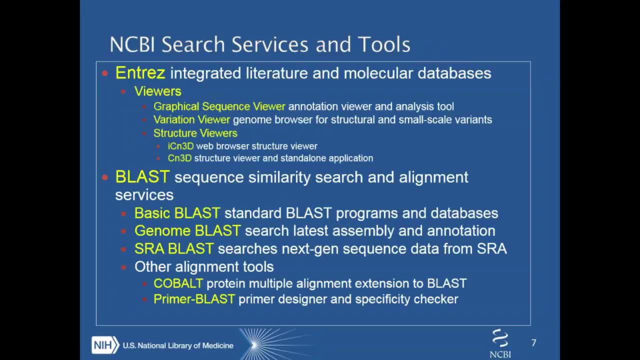 with that are some viewers: the graphical sequence viewer. we're going to use that today to look at some genomic sequences. there is a variation viewer that's really set up for mouse and mouse and human right now structure viewers. there is a old-fashioned one you can download called cn3d. 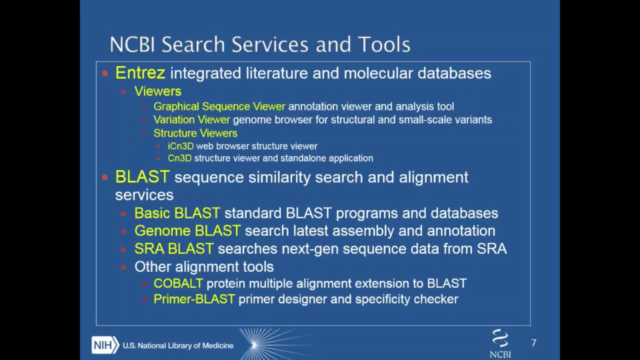 and today i'm going to show a structure. i'm going to use icn3d, which is a web-based application, so it runs right in your browser. you don't need to download anything. so entre is a tech search system. service blast is the other way of getting into. 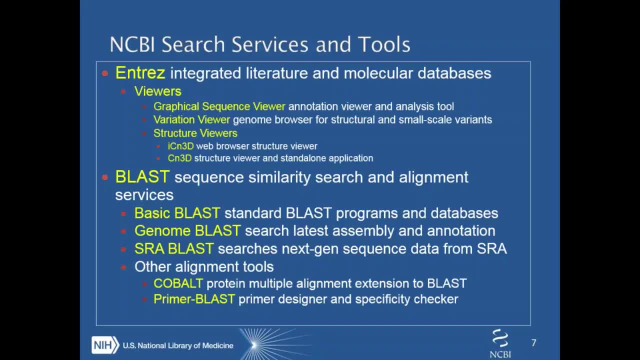 our databases and that's using sequence similarity search. there's a number of different kinds of blast. today, in my portion of the talk, we're going to talk about basic blast. We're going to use basic BLAST. Really, we're not going to talk a whole lot about how it works to find homologs. 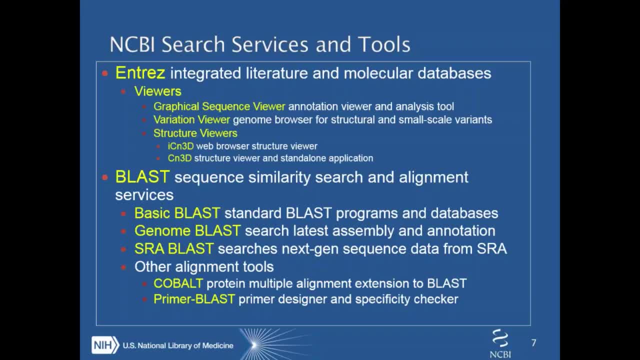 Ben's going to probably do some talking about SRA BLAST, which is looking at next-gen sequencing data, And the other alignment tool that I'm going to show you today is Primer BLAST, which is a very useful tool for designing primers for DNA sequences. 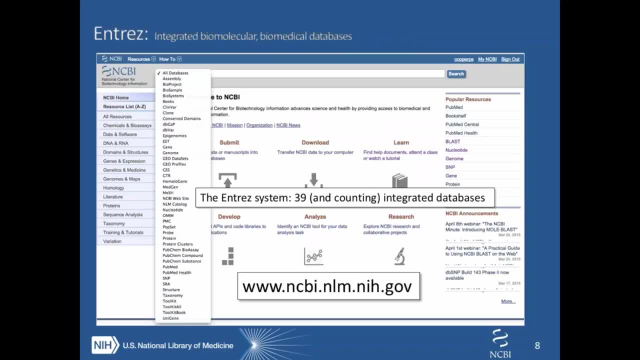 and I'm going to show you that with a genomic sequence. So the Andre system is available from our homepage. You can search 39 databases there. These databases are integrated in the sense that they're connected to each other. If you find a record in one, you can link to records in other databases, and I'll show you that today. 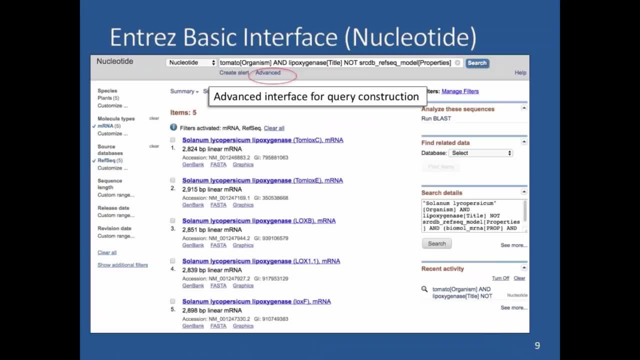 There's a basic interface and here's the basic interface for nucleotide, which is a complex Boolean-type query. I could construct a query like that through the advanced interface. I'm going to show you that in just a minute, just to show you a little bit of the structure of the webpages. 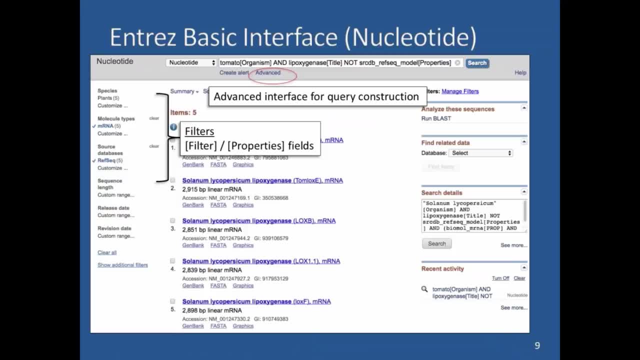 There can be filters on the left-hand side that will let you filter by different parameters. You can also see the properties of the particular records you're looking at. For example, here you've got sequence length, publication date, modification date. There's also a thing that we've called the discovery column, which is present on the search results. 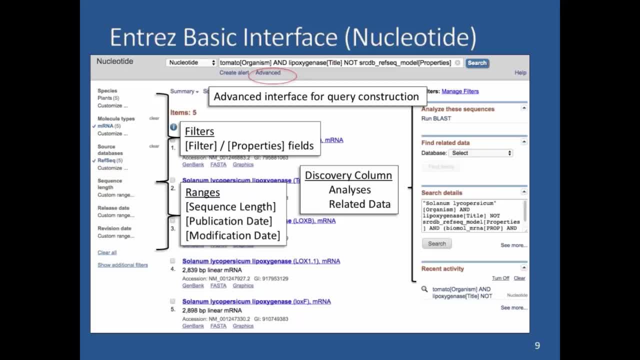 and also present on the records. that lets you get access to analyses and related data. So here is a complex Boolean query that you can construct using the next interface and I'm going to show you which are the advanced interfaces. And here I'm showing you the advanced interface from BioWare. 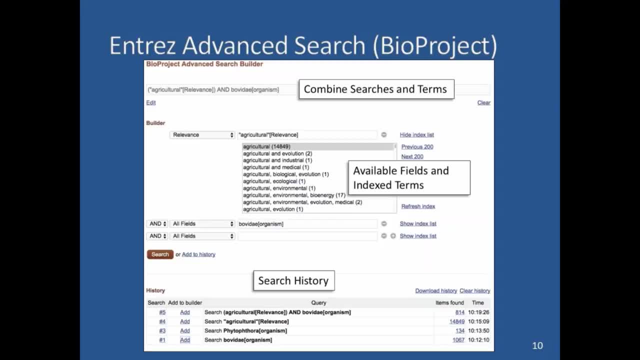 In BioProject. all these advanced interfaces work the same way for the different Entrez databases. I just wanted to show you this particular field search here in BioProject and that's agricultural relevance, which is a way of getting projects that have that kind of relevance assigned to them by their submitters. 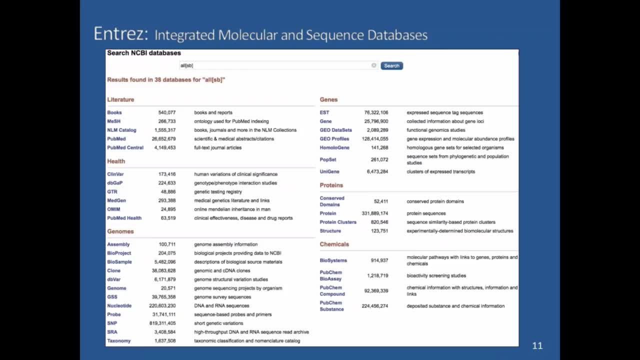 That's a useful term if you're looking for things like that. Here's the Entrez system in a way that you can search all the databases at once, And the question that you often come across when you're doing this is: where do you start with all these different databases? 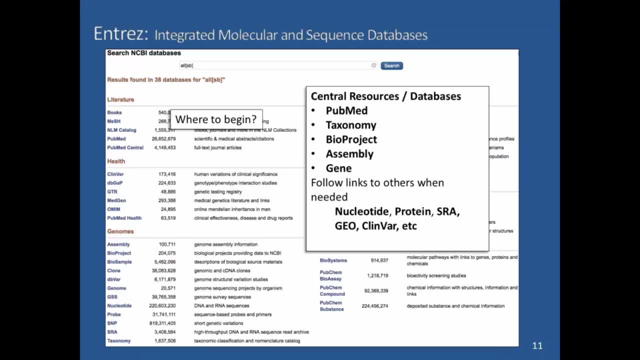 I just want to point out that there are some sources, There are some central resources that really are the best places to start and you can link out to the other ones to get the data you want. So PubMed, our taxonomy database, BioProject, Assembly and Gene. 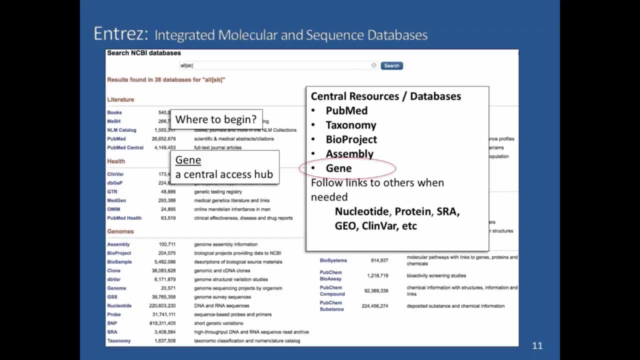 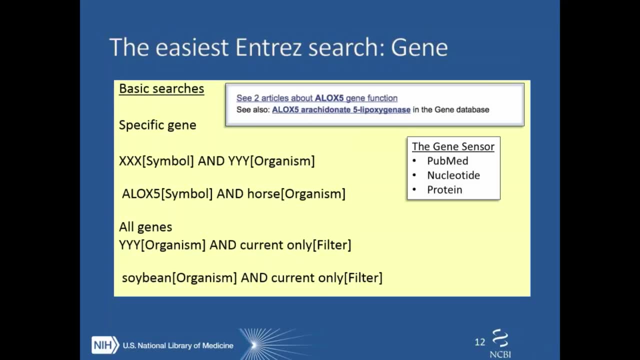 And for my examples, we're going to start in Gene and link out to some other kinds of data. Gene is useful for lots of different reasons. One of the things that's really good about it is it's very simple to search. You can search for a specific gene with just a very simple query with the symbol and the organism. 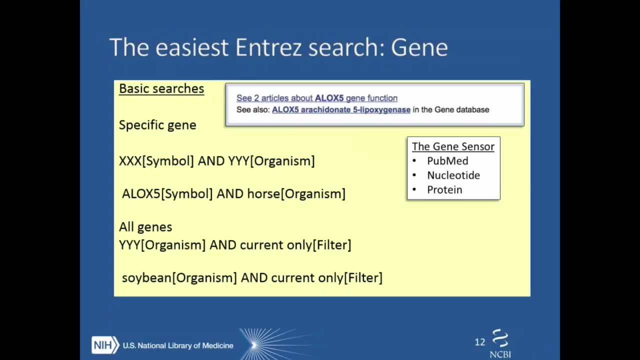 for example, there's a way of finding 5-lipoxygenase for horse, Or you can get all the genes for a particular organism just by making sure you have the current only filter. That's on by default in the web anyway. And then at the top of this slide there's this screenshot of something that we call the gene sensor. 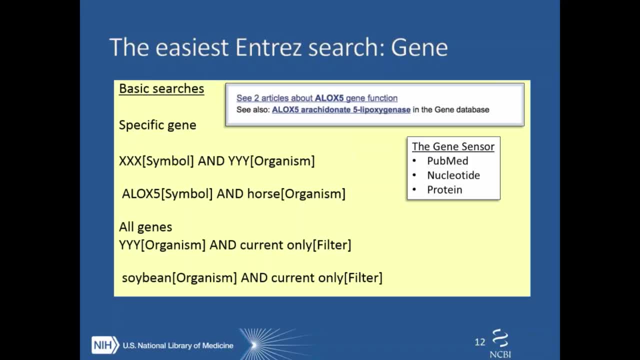 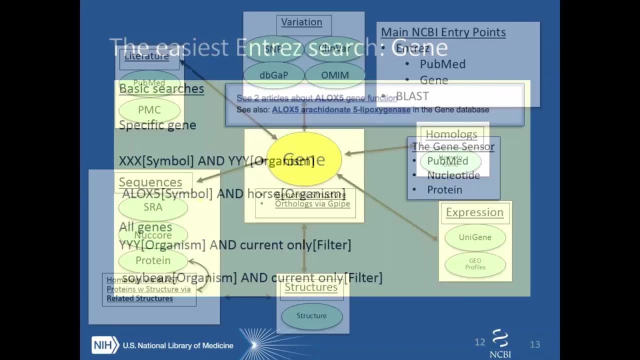 which is much more active for things like human, but you can also specify an organism like horse in this case. You can get some direct access to the gene record and also PubMed articles that are attached to that gene record, And I'll use that as a way to get into the database today. 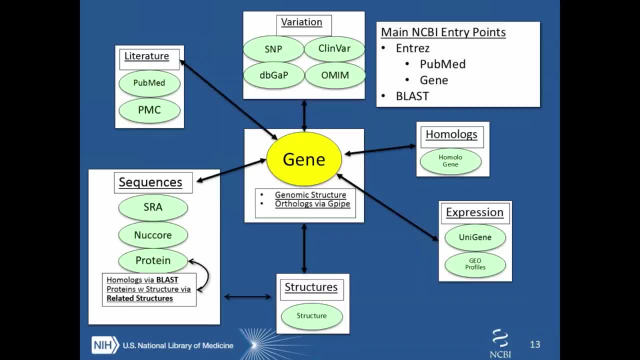 So this is sort of a diagram of the Entrez system. that is kind of complicated but it shows you Gene as sort of the central hub, And starting there makes things a lot easier if you're interested in particular genes and their products or things associated with genes. 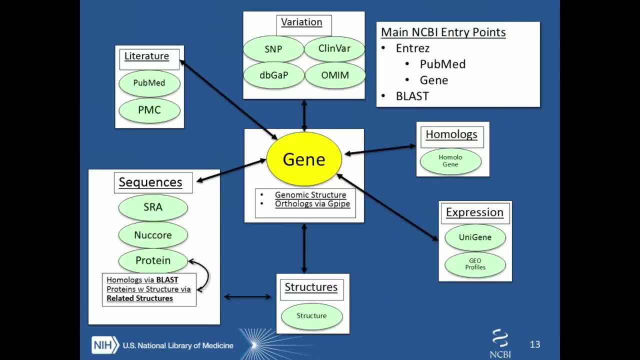 And so you can link out, as it shows here, to these other databases. You can find sequences, literature, variation, homologs on other species, expression, information and structure. Okay, so what I want to do now is do some quick live demos. 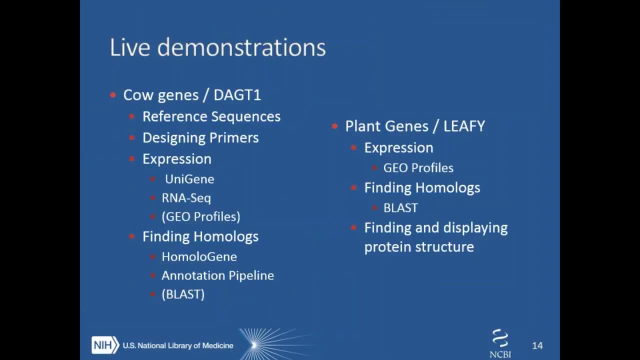 We're going to look at a gene from cow, DG81.. We'll find some reference sequences for that. We'll design primers for an exon of that gene. We'll look at some expression resources: unigene and RNA-seq data. 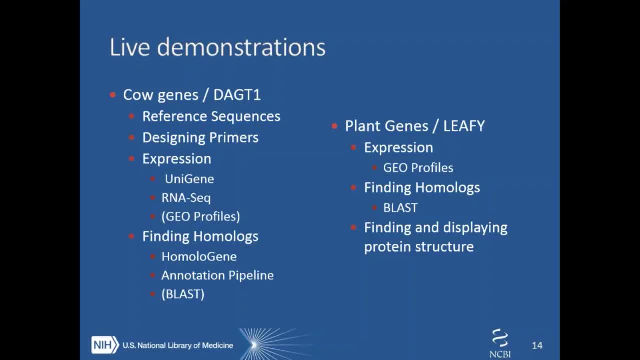 And Ben's going to talk more about RNA-seq in his portion of the talk. Geopropyls is listed there. It's a commonly used expression resource but we won't be using it for that gene. I'm going to use it for an Arabidopsis gene in the second part of the demonstration that I want to do. 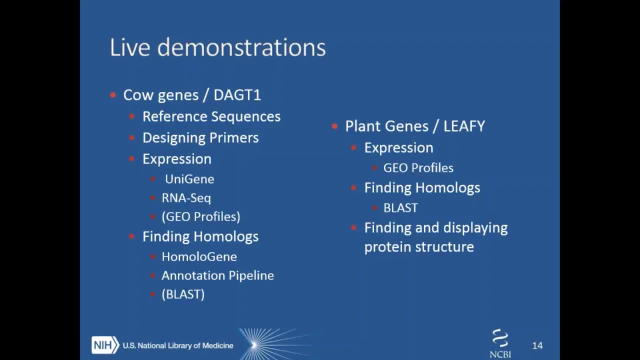 We'll find some homologs using homologene in the annotation pipeline And of course we could do that using BLAST. Again, I'm going to save that for the plant genes. So on the second part of my demo, I'm going to look at the leafy gene, which is a transcription factor in Arabidopsis. 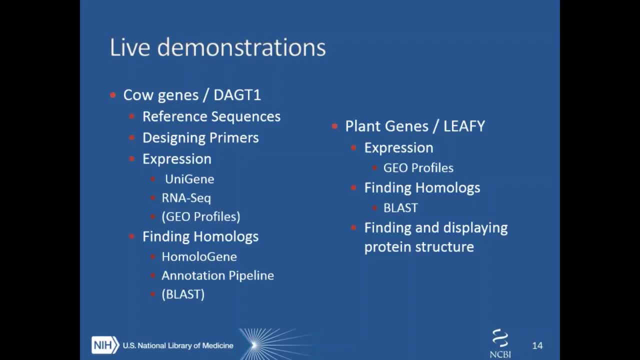 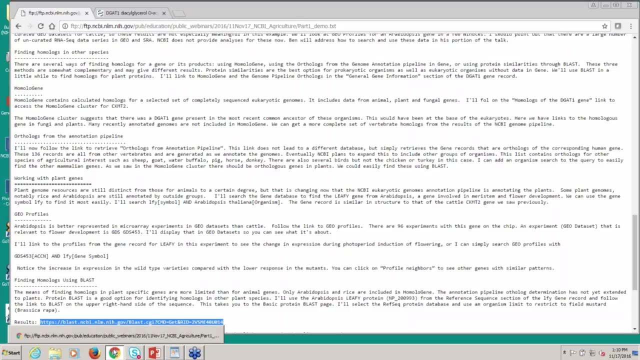 We'll look at geopropyls, We'll also find homologs using BLAST And finally we'll display a structure of that particular protein product. So I want to stop here and exit the slideshow, And I'm going to launch a web browser here. 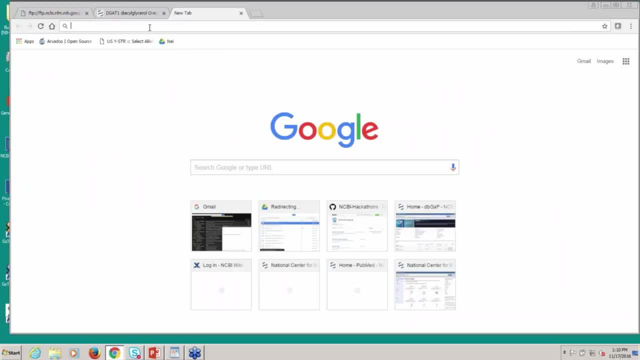 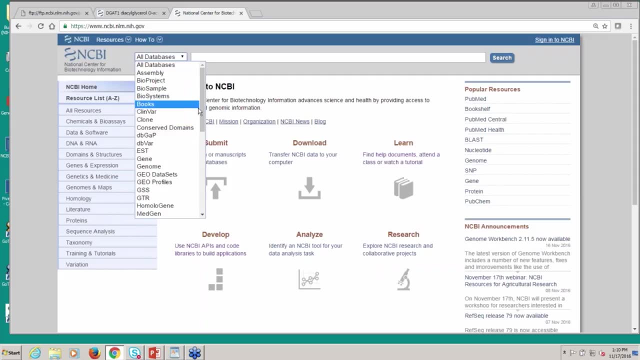 And I'm going to go to a new tab and I'm just going to go to NCBI And what I'm going to do here is I'm going to go to the PubMed database And I'm going to search for a particular gene: PAGT1. 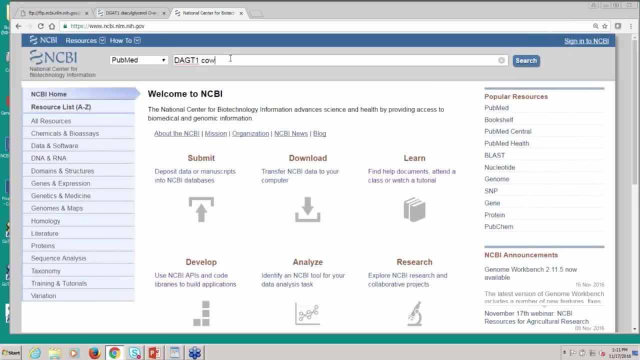 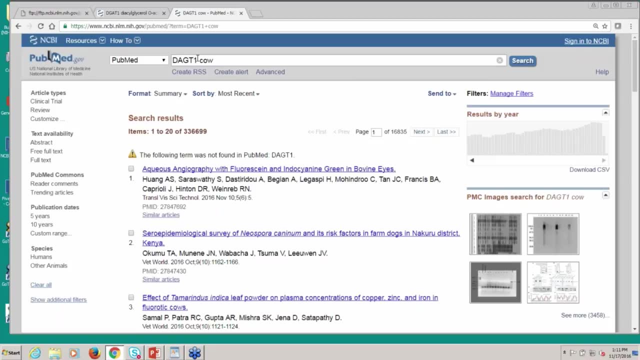 And I'm going to type the name of an organism. after that, The name I'm going to type is cow. Yes, and I keep doing this to myself. I think I'm getting dyslexic. DGAT1.. Ah, that worked a little bit better. 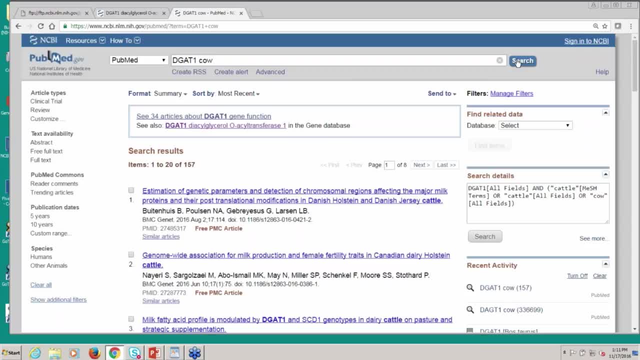 So that's a gene name, And so the gene sensor, which is that box that you're seeing at the top, recognize that as a gene name And it gave me access to the gene database. That's the second line in that box. 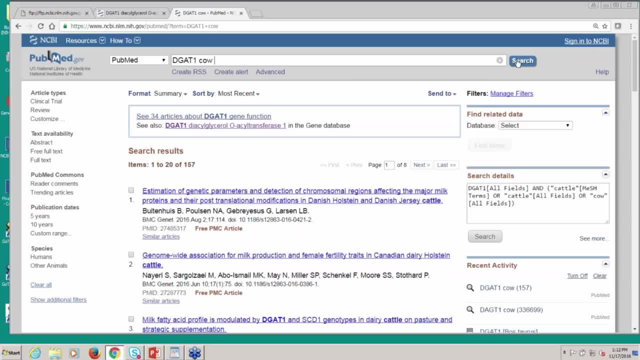 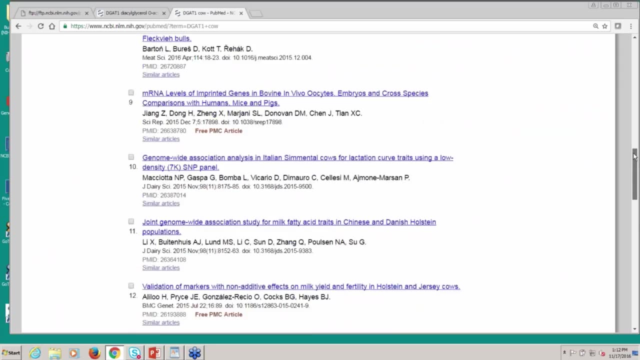 The top line gives me a selected set of articles about the DGAT gene function that are linked to that gene record, And if we just scroll down through these a little bit here, you'll notice that there are several of them that talk about a particular polymorphism. 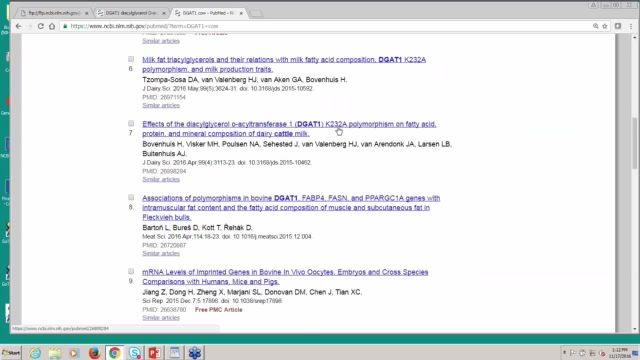 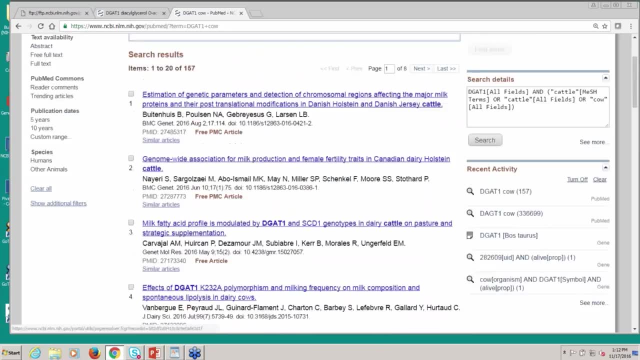 which is a lysine 232 alanine polymorphism, And we'll come back to that in a few minutes. We're going to look at that particular thing in the gene record, So what I can do now is go to the top of the gene sensor. 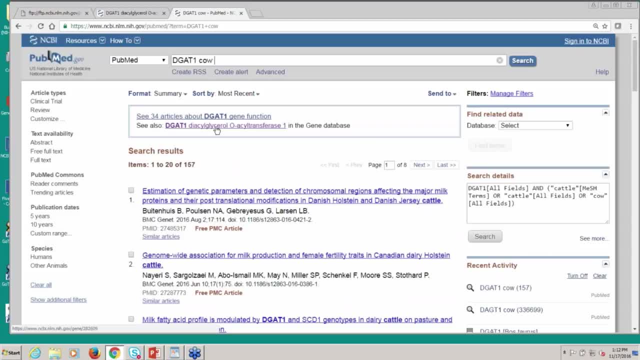 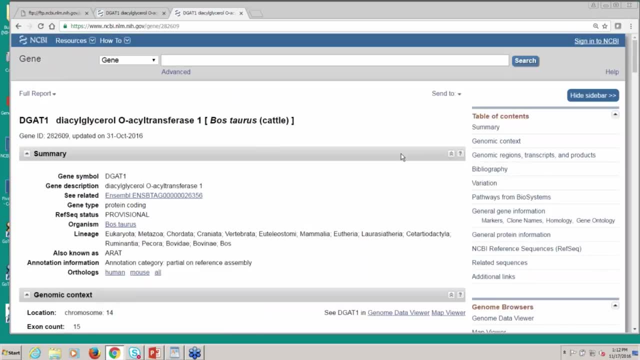 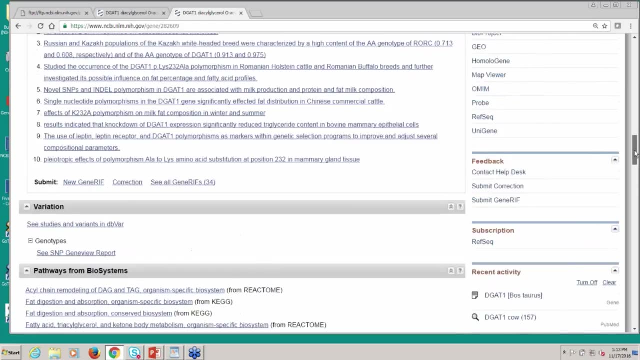 and I can click through to the gene record for cow or this diacylglycerol oacyltransferase gene in the gene database. So this is a gene record. It's a typical-looking one for sort of a non-model organism like cow. 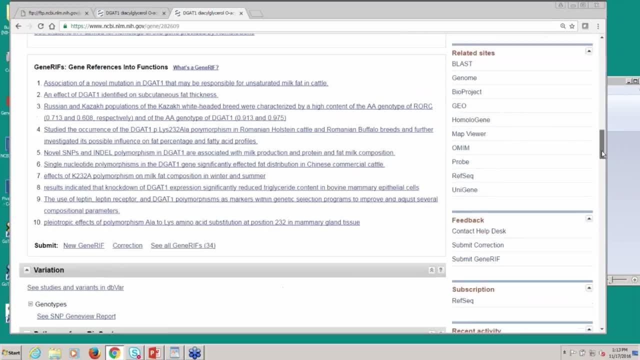 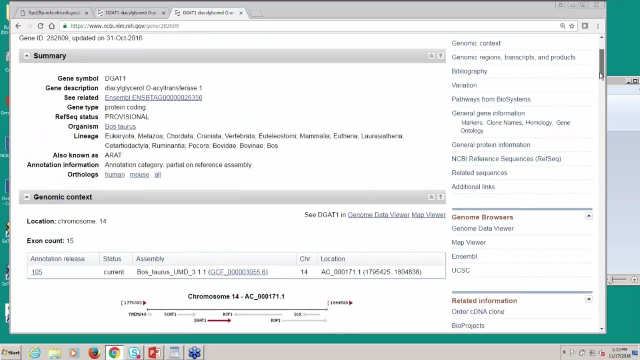 Human one would be more extensive, But this still has a lot of information on it. You can scroll through here and you can see there are lots of things here. We're going to focus on a few aspects of this. We're going to look at sequences. 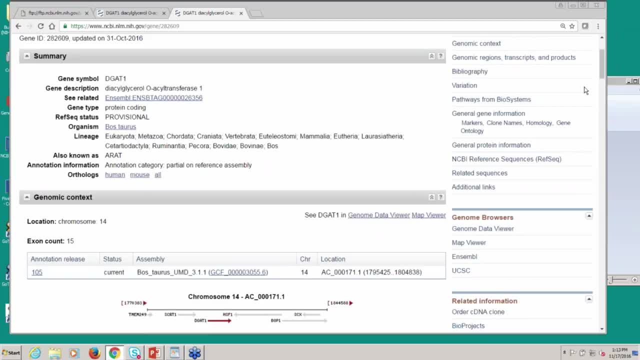 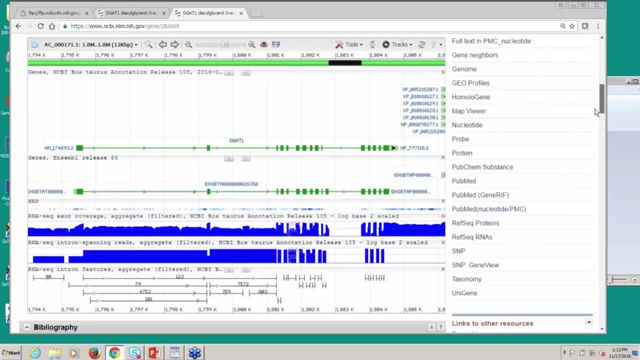 We'll take a look at some expression information, some variation. We'll mess around a little bit with the graphical sequence viewer, which is that object that's embedded in the center of the gene record here that has lots of details about this region of the cow genome. 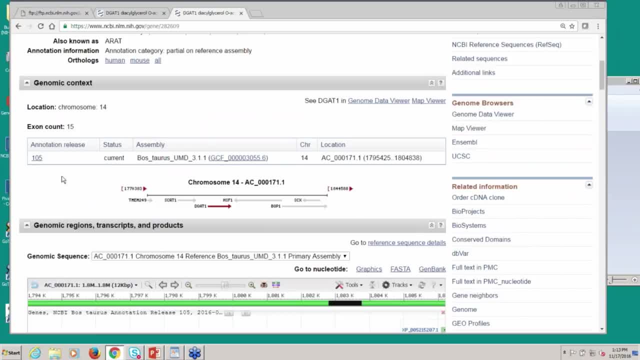 You can see we're looking at chromosome 14.. The annotation release here gives you the current annotation on the cow genome. It goes to our eukaryotic genome annotation page and this gives you information about the assembly and that's where you would go to download this if you wanted to get this key data. 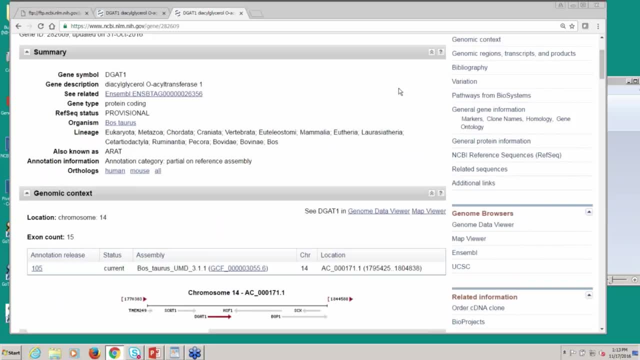 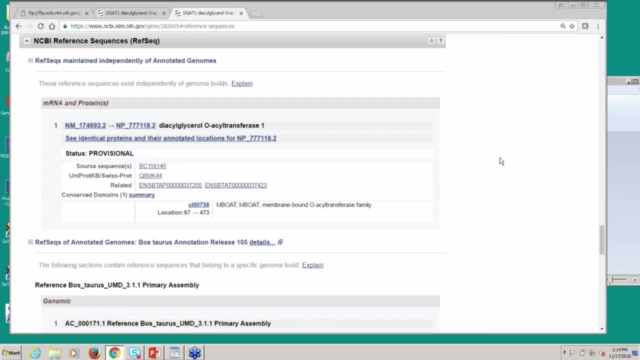 So the first thing I want to do is to just show you some of the sequences that are here, and I'm going to use this shortcut here to jump down to the reference sequences section. There are two kinds of sequences, typically in one of these eukaryotic genome pages. 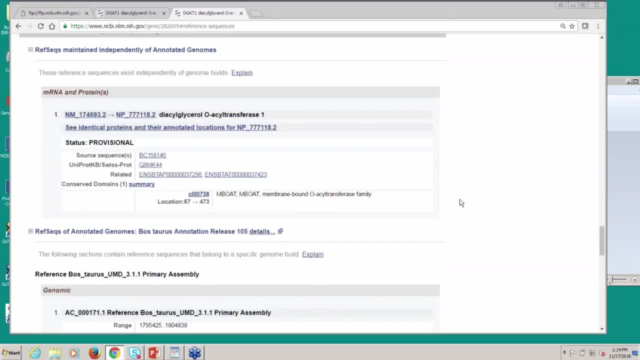 There are those that are so-called maintained, independently of the annotated genomes. These are based on sequences that we have in our primary sequence database called GenBank. In this case, we have a single transcript aligned to the genome and its corresponding protein translation. In a few minutes we'll talk about the gene model sequences that are based on the RNA-seq data. 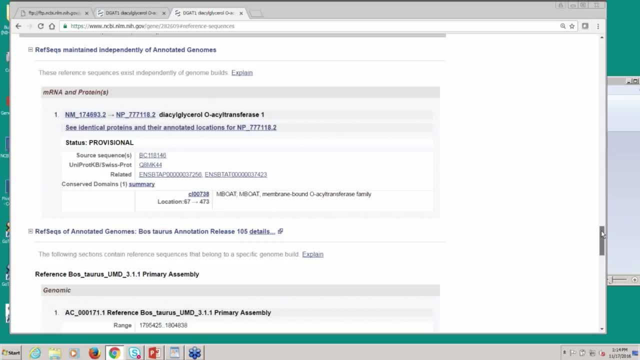 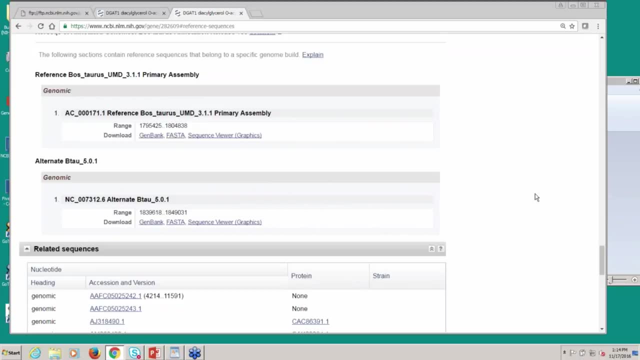 There are none present in this particular record, but there are in some nearby genes. There are two assemblies here. They both use the same underlying data- The University of Maryland 3.11 assembly to annotate, and so that's our so-called reference genome. 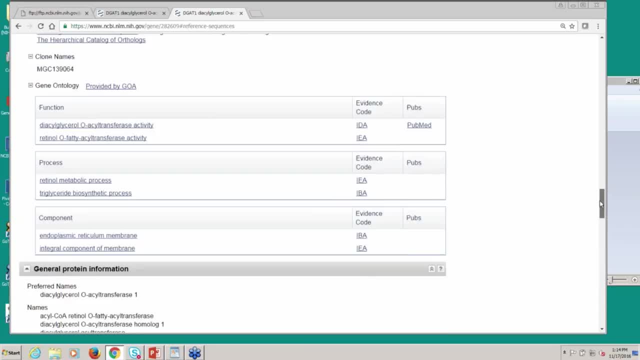 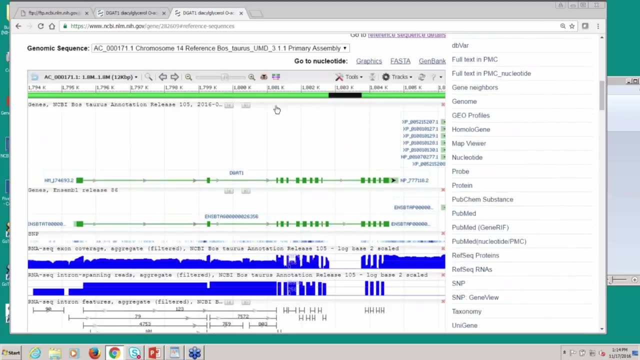 So to focus on these sequences and their annotations, I'm going to go to the center here and look at the graphical sequence viewer. At the top is a line representing the genome sequence. You'll notice this black region here. That's because that's missing data. 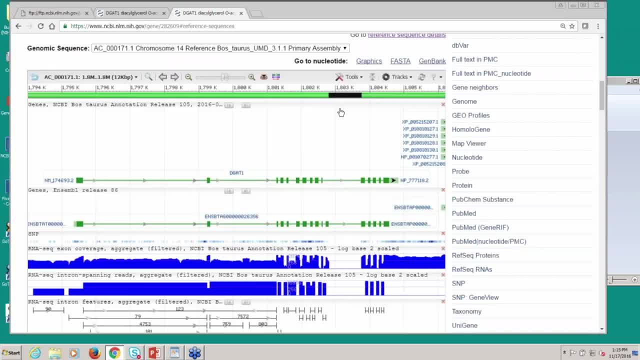 So there's some missing data right there in this region of the cow genome. Here's our annotation of the cow genome, based on alignment of that genome. We have the messenger RNA sequence. We have the ensemble transcript aligned. here too, We have some variations. 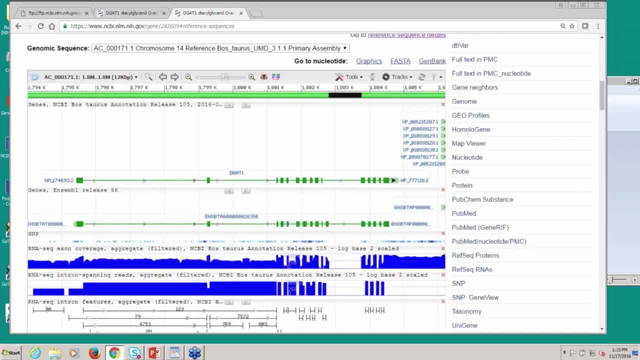 We have these RNA-seq tracks which show you the alignment of RNA-seq data. that's coming from our SRA database. We use these extensively in our annotation of the genome. We can change the way this looks a little bit if we want to. 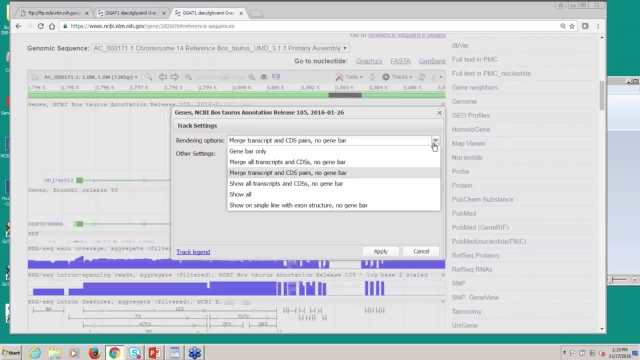 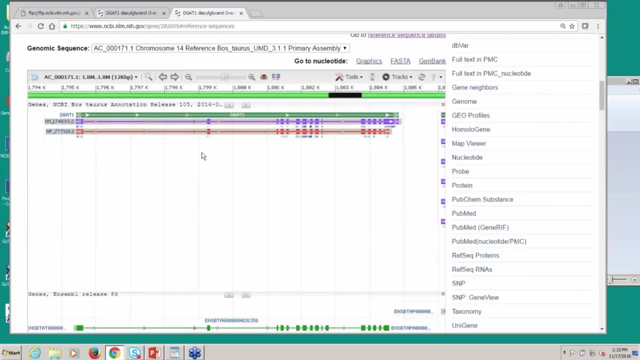 I'm going to click on the top of the gene track and I'm going to change this so that we're seeing everything. I'm also going to project the SNPs onto this. So now I can see the corresponding transcript and the protein translation of that transcript. 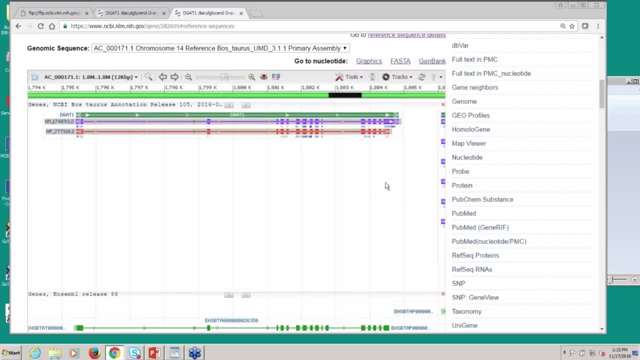 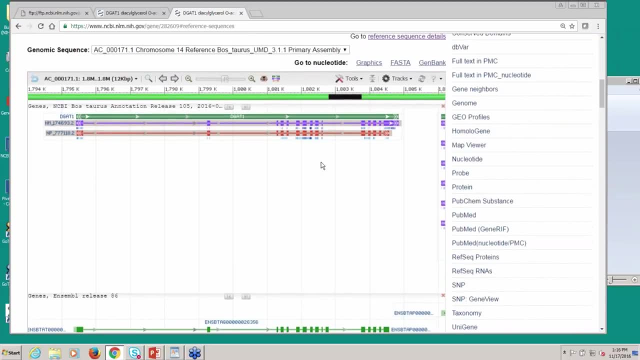 You'll notice that it's incomplete at the 5 prime end and the 3 prime end. One of the things that we're going to do is we're going to use a feature of this to find that particular variant that we saw in PubMed. 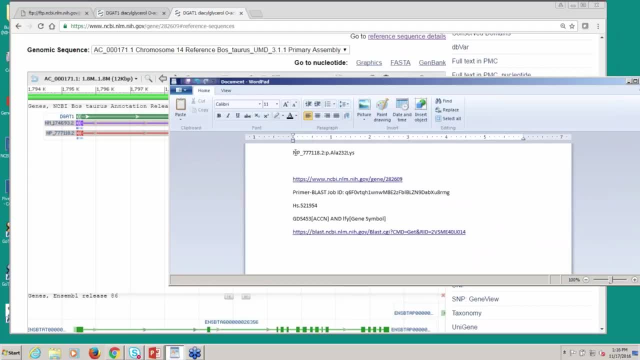 And I've got a little scratch pad here where I've written this down as what's called a Human Genome Variation Society notation, And I can actually find this protein position- This is alanine- at position 232 of this protein sequence, which is our REPSI protein, in the graphical sequence viewer. 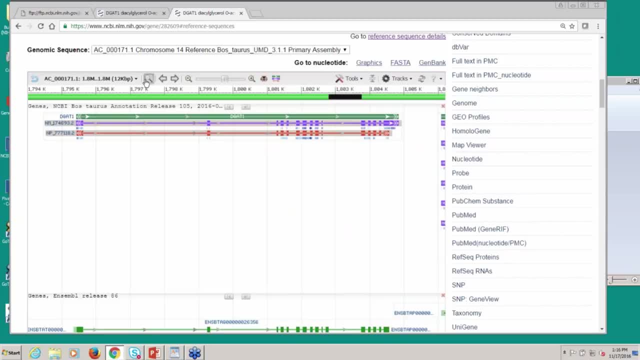 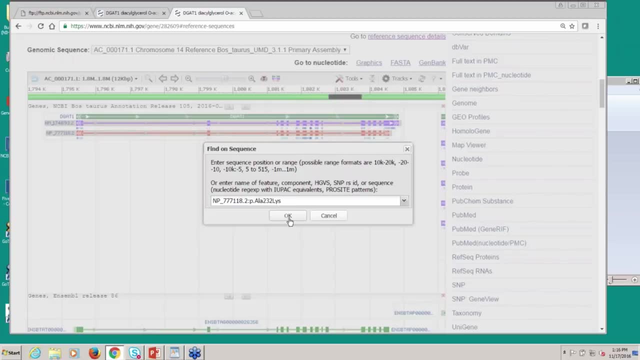 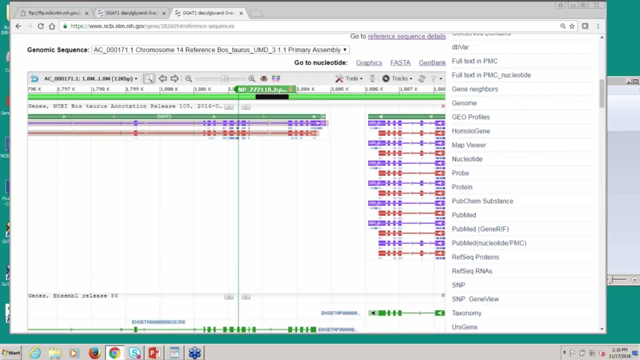 So I'm just going to copy that to my clipboard and I'm going to search for it. I clicked on that magnifying glass to activate the search feature And voila, it has now landed on the genome at a particular place, And we're going to use this particular piece of information to do some things. 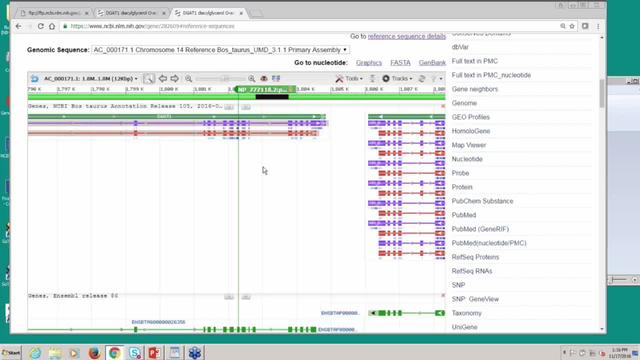 For example, this is a variant that affects- if you read some of those articles, this variant affects the quality and the quantity of the milk produced by these cows. So it's an interesting variation from an animal husbandry point of view and from a dairy farming point of view. 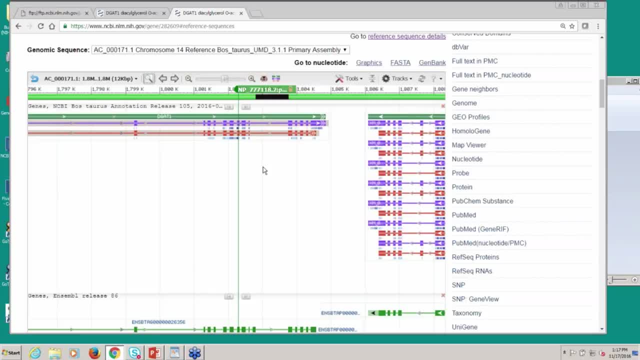 So it would be interesting, for example, to assay this The way you might do that is by PCR. So what I want to do is we're going to take this particular exon. You can see that that's an exon. I'm going to zoom in a little bit. 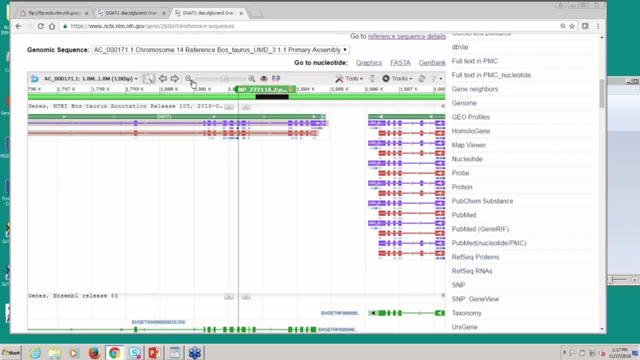 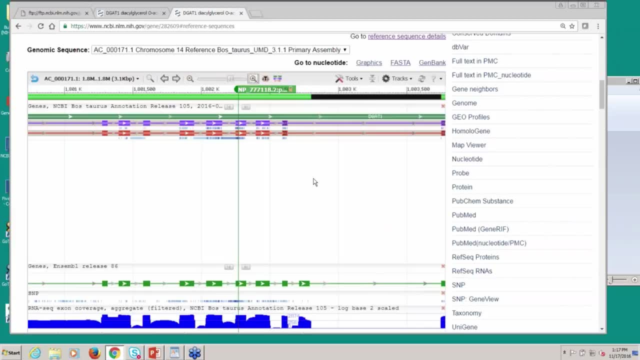 Do that And if you count the exons of this gene, it happens to be number eight from the five prime end. So what I want to do is show you a way to design primers for that particular exon. What I'm going to do is I'm going to go into a different window over here. 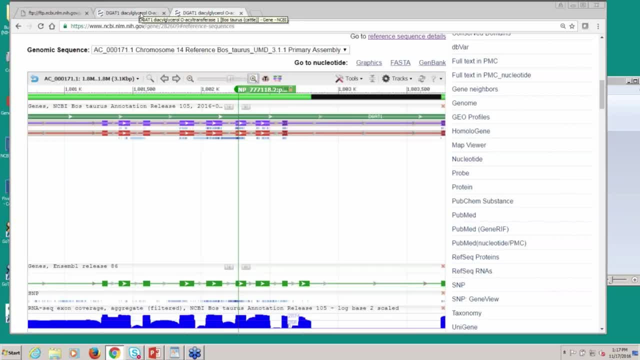 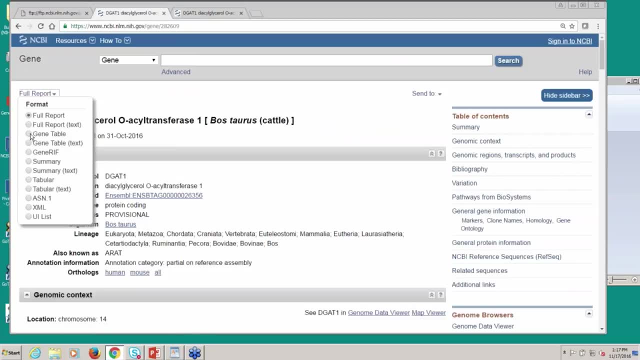 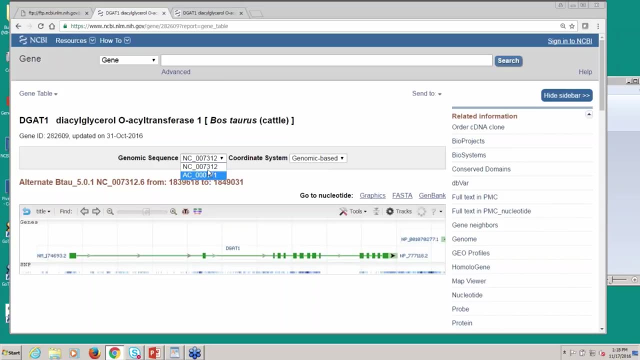 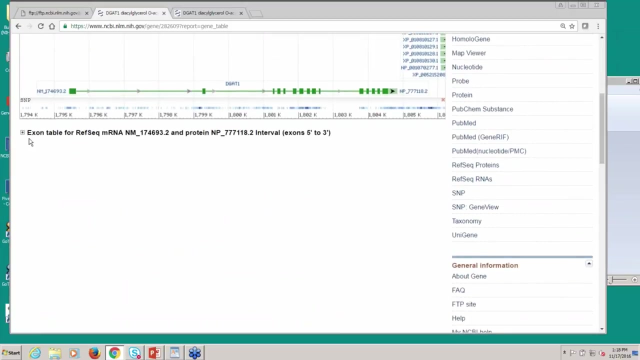 and the same gene, but just so I don't lose my marker that's in this particular view here. So here's the same gene and I'm going to change the report here from full report to gene table. So this gives me a blow-by-blow description. 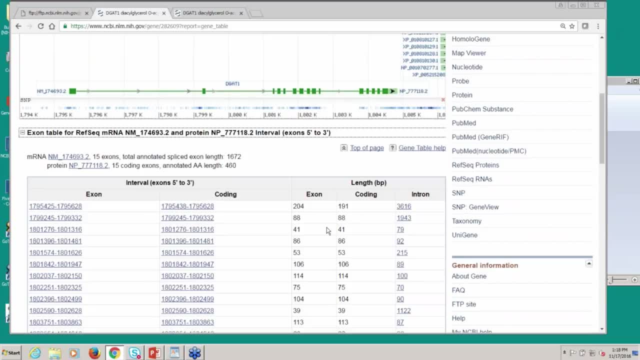 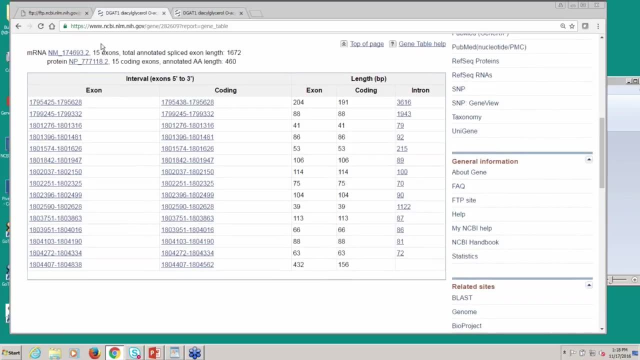 if I expand this exon table of the exon intron structure of the gene And any of these links will let me load that. So if I count one, two, three, four, five, six, seven, eight, this is the exon that I want. 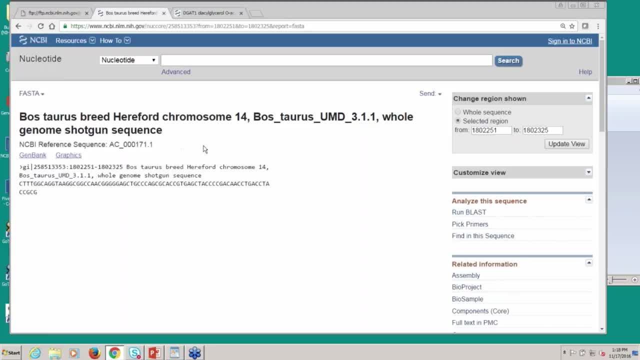 So I'm now leaving gene and I'm going to the nucleotide database. I can take this piece of DNA and I can load it into Primer Blast. If I follow this link here that says pick primers, that's what that will do for me. 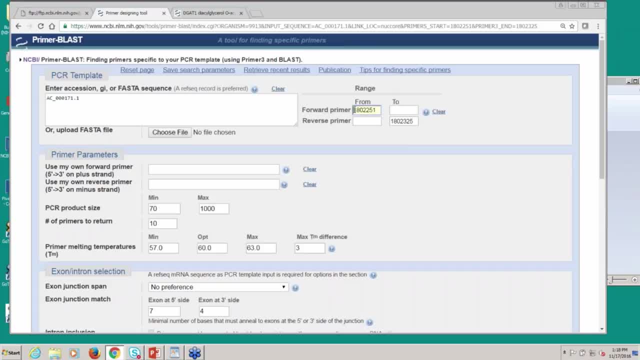 So what I can do is adjust the coordinates here to get a little bit of the upstream sequence if I want, So 100 bases upstream of this. Likewise, I want to go beyond the end of this, So I can adjust the end of this region too. 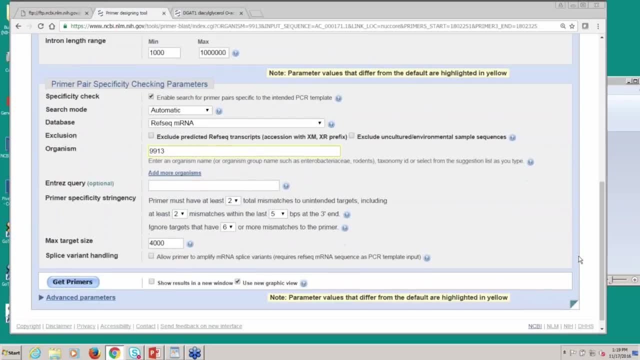 And then I just want to go down here to pick the background database. So it's going to basically design primers that are specific to this particular piece of genomic DNA. So I want to change my database here to the reference assembly. So this will search the cow reference assembly. 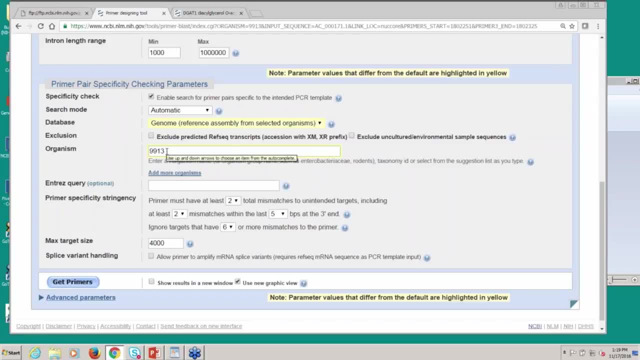 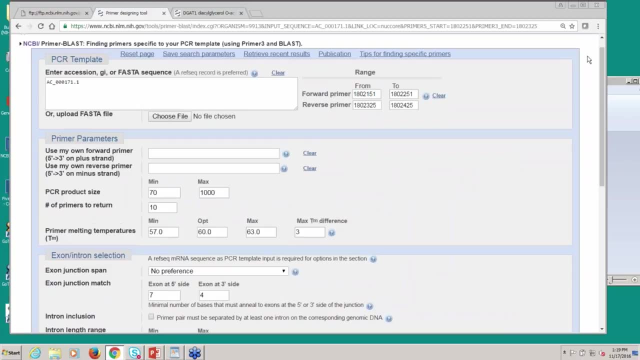 and that's what this organism identifier here is, and it will give me specific primers. Now, it takes a minute or two to run that, so I'm actually going to load my results through this little tab here, this little link here. 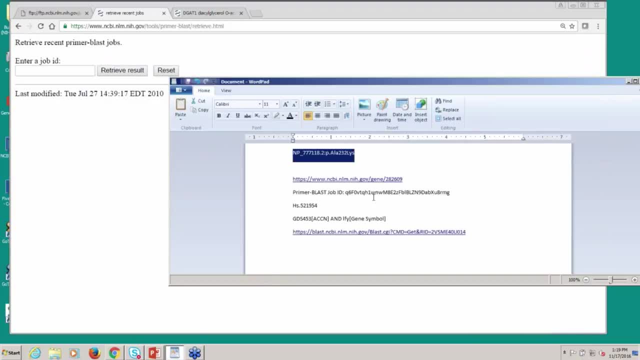 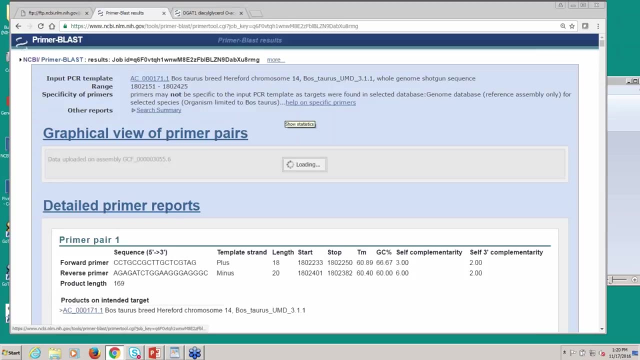 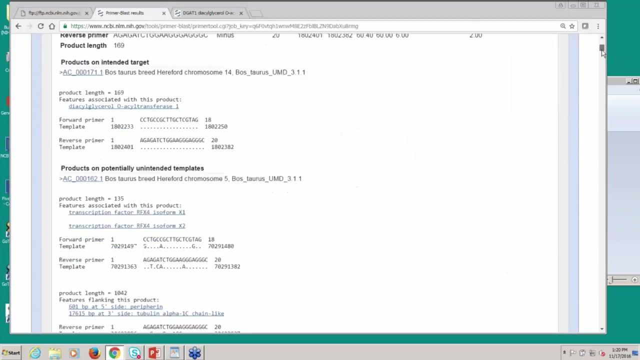 I've saved these results from this morning. It warns me that my primers may not be specific and you can take a look and see what that is all about. You can see that there are other places that these match in the genome, but they've got a number of mismatches. 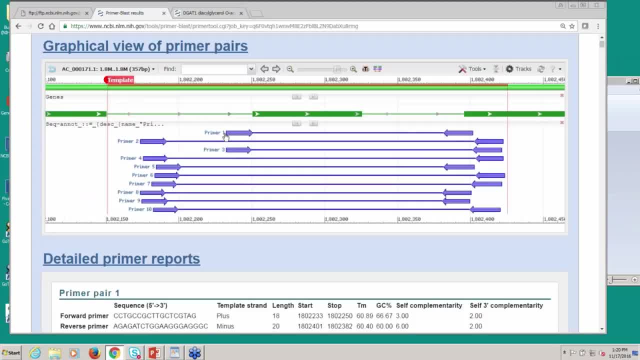 So if I'm fairly stringent about this, this should work just fine. Notice, I have a number of options for primer pairs that I could use to amplify this particular exon from the cow genome if I was trying to assay a particular cow whether they carried this particular polymorphism or not. 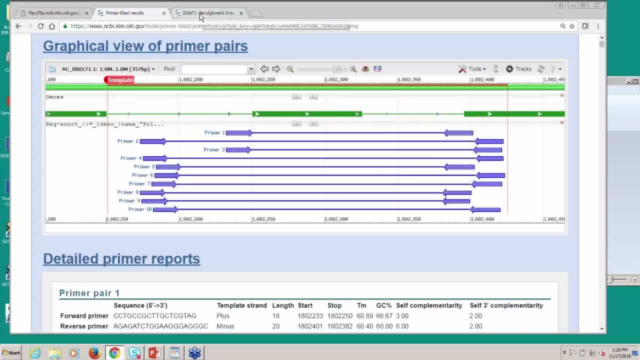 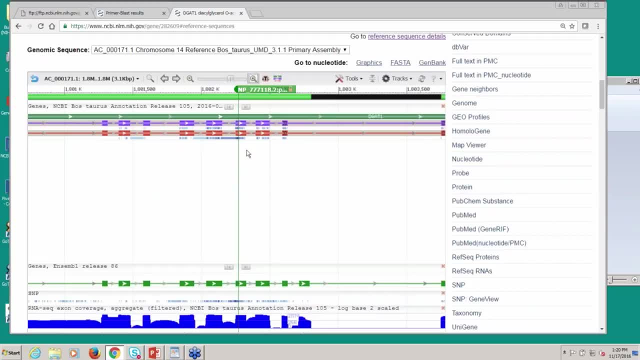 I could do that. So let's go back over here to the gene again, And so now what I want to do is let's take a little bit more close look at that particular position in the genome. If I can go back to my marker, 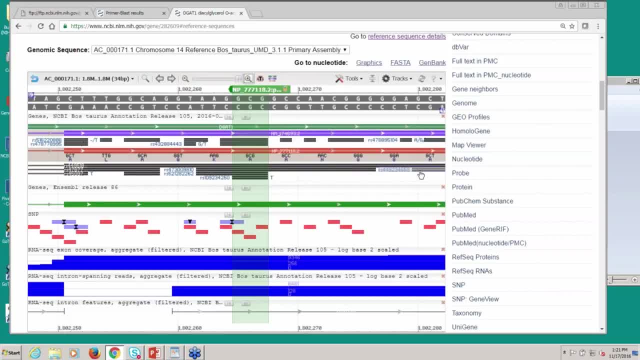 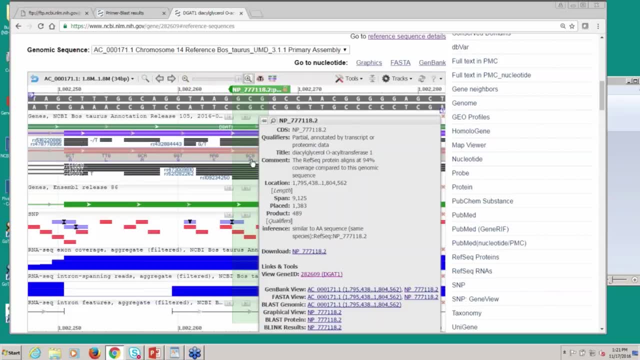 I can zoom to the sequence at the marker, And now I'm zoomed in quite far and I can see the alanine codon that's there in the reference genome. Notice that it's mapped onto the protein here. One thing to notice about this: 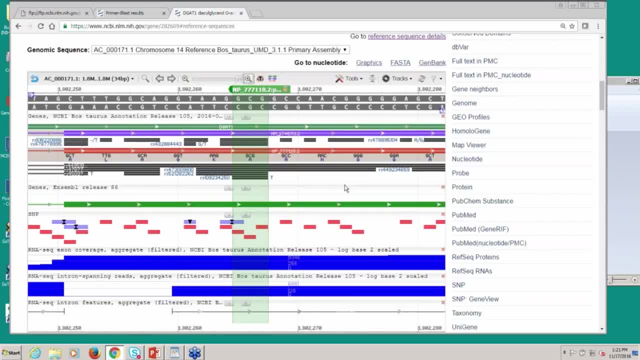 is that we don't have this particular variant in the database. We do have one here that changes the alanine to a threonine, but we don't have the one that changes the alanine to a lysine. dbSNP: our database variations. 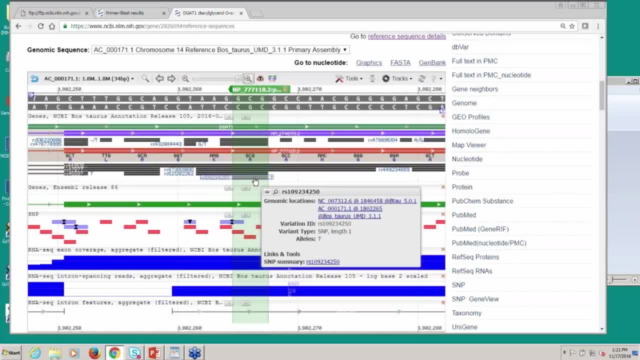 is a submission-driven variation database. We have a lot of cow SNPs- We have about 94 million of them at this point- but we don't have this particular one. Okay, so we could from here, of course, link into the SNP database. 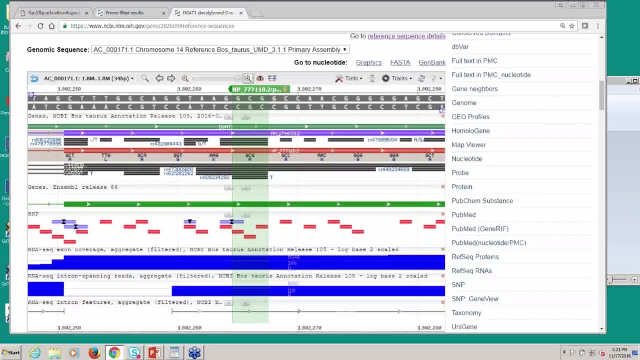 through the refSNP ID. I'm not going to bother to show you that right now, but you could go there and learn more about what SNPs we have for this particular record by following the links here to SNP or to gene view, which gives you some more. 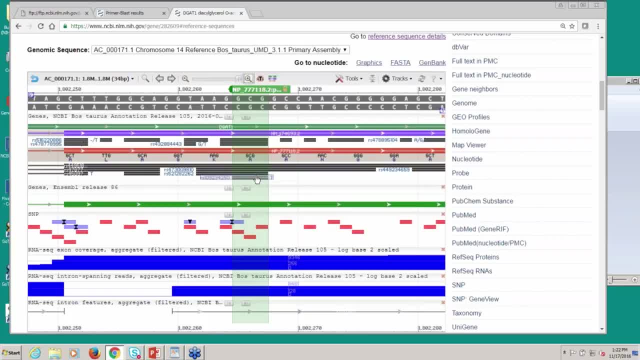 detailed information about how these SNPs map onto the protein, And that information is shown here. It tells you that it's going to change that alanine to threonine by mouse over this particular graphic object here. Okay, So the next thing I want to address. 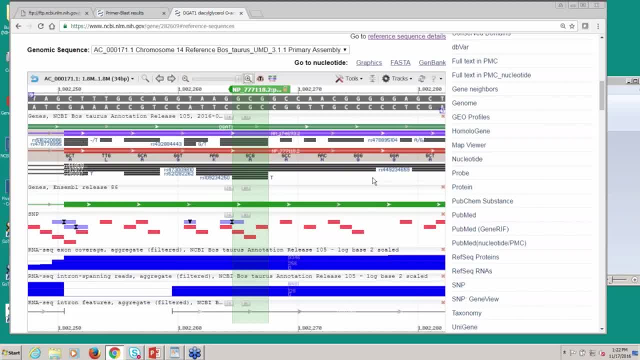 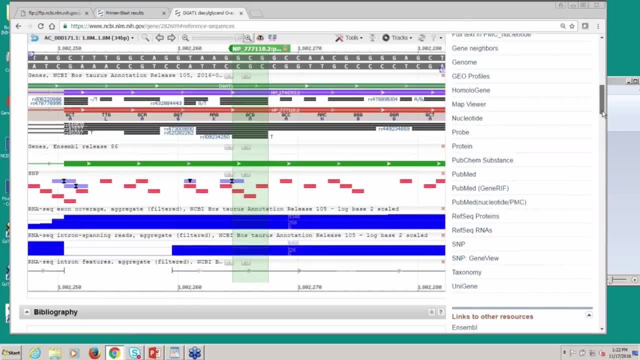 a little bit is sequence variation. There are a couple of different resources linked here that tell you about sequence variation that are in other databases. One of them is Unigene, One of them is GeoProfiles, which are based on microarray data. 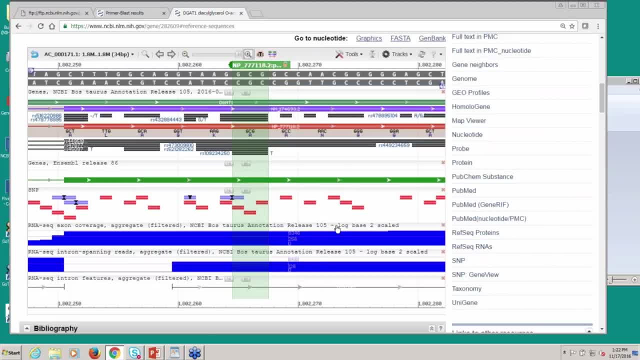 And then the other one is actually right here in the graphical sequence viewer, which is the alignments of these RNA-seq data. So we can see here. let me just go ahead and I'm just going to click on the gene here and click on that little magnifying glass. 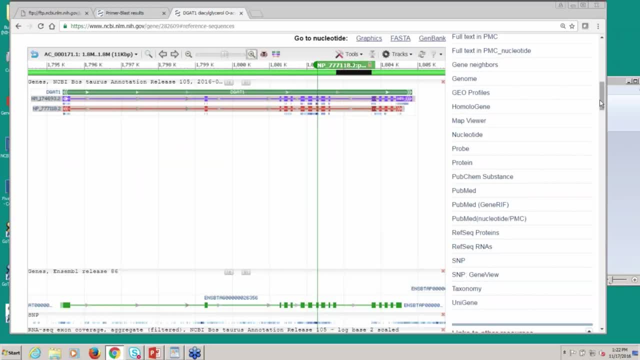 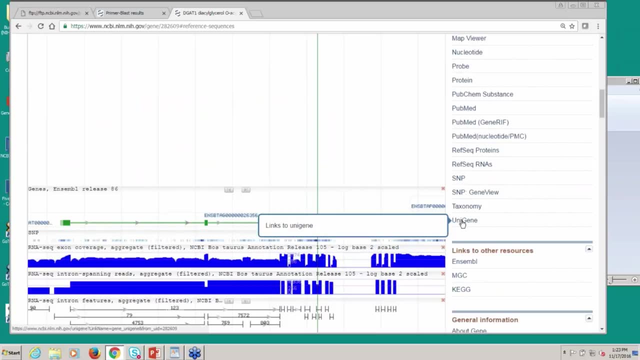 and it will zoom me back out to where I want to be. So the first one I want to visit is an old-fashioned database. It's no longer being developed, It's Unigene, but it's still useful for a lot of organisms. 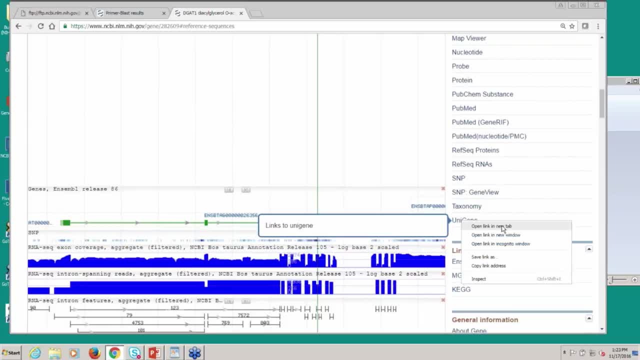 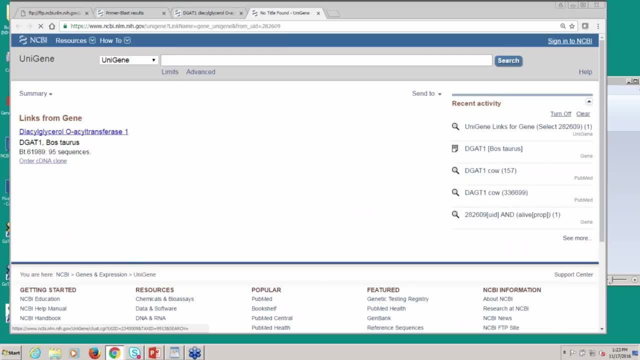 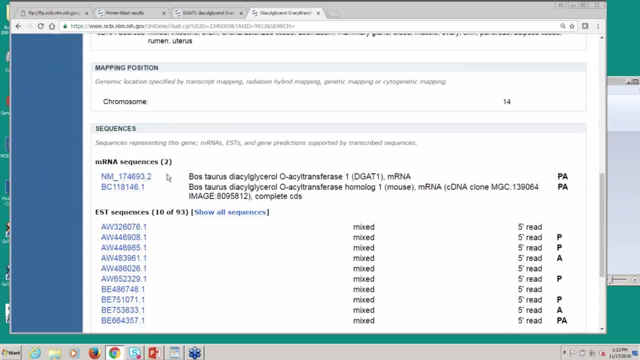 even cow in this particular case. So I'm going to open that in a new tab to show you what happens. This is a cluster based on old-fashioned EST sequences which are first passed single-read sequences from CDNA libraries from various tissues. We have two. 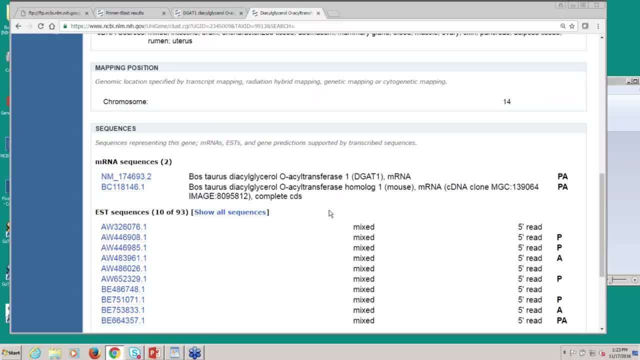 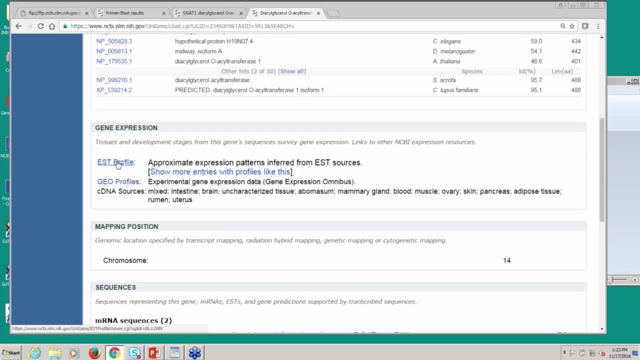 traditional types of sequences in here plus 93 EST sequences. You can basically count the sequences that are coming from particular libraries to get an EST profile out of this. I can show you one right here. It's not a whole lot of sequences for the cow gene. 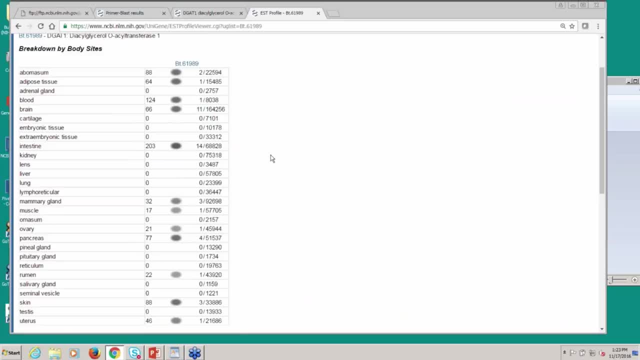 and there's not a tremendous amount of CDNA libraries in terms of numbers compared to, say, human, but you can get the impression that this gene is expressed in lots of different tissues. Particular seems to be highly expressed in the intestine, If you want to see the corresponding gene. 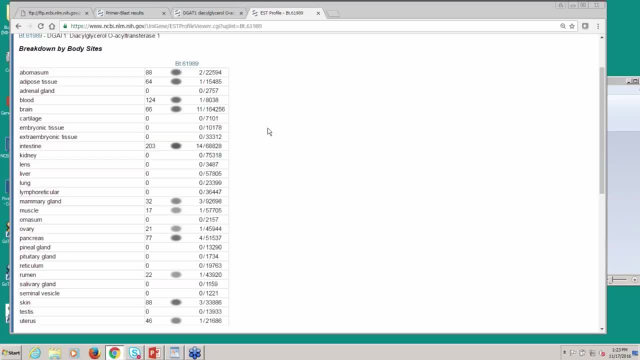 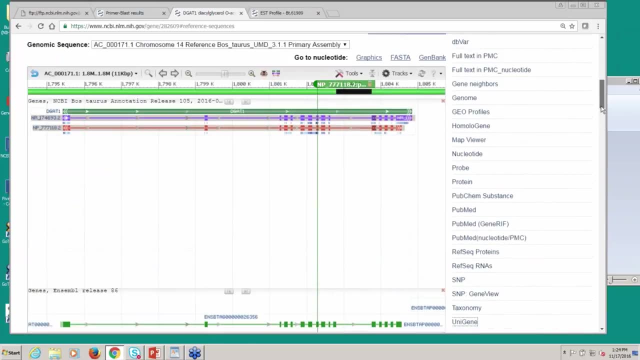 in human. you can do that in Unigene. You can see that there are a lot more CDNA libraries available. The other source of information would be geoprofiles, but there's not a whole lot of curated profiles for cow. Ben's going to talk a little bit later on. 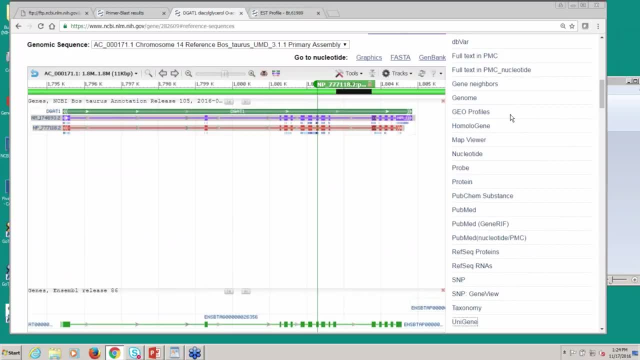 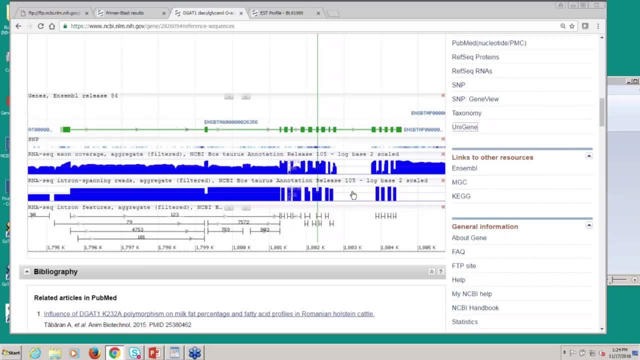 about RNA-seq data, which is a source of expression information that you can analyze yourself. We have aligned some of that to the cow genome. You can see that down here. These are the aggregates here. If I wanted to add something else. 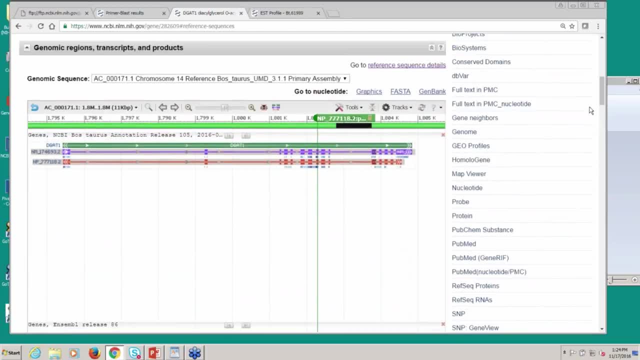 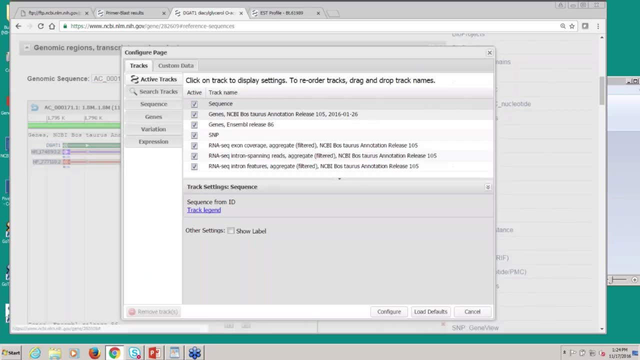 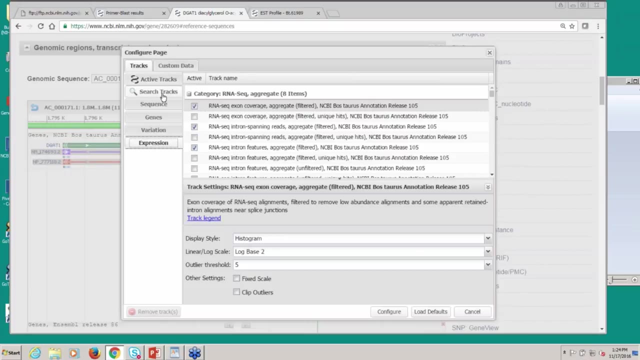 other tissues. I can do that by going up here to the tracks menu. I'll click on that. I'll click on configure tracks. Notice that there are expression tracks available. What's up there now is the aggregate. These are the search tracks. 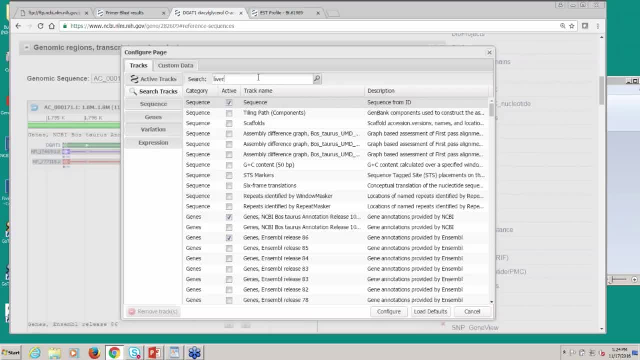 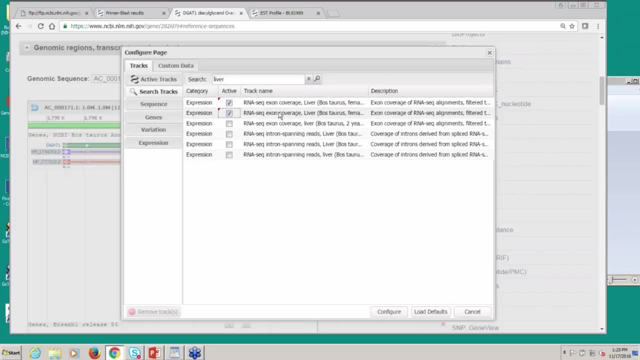 Suppose I wanted to add, for example, a track from liver. I'm just going to search for liver. There are some liver tracks there I could search. These are the exon coverage, which is basically the alignment. The intron spanning reads are very useful. 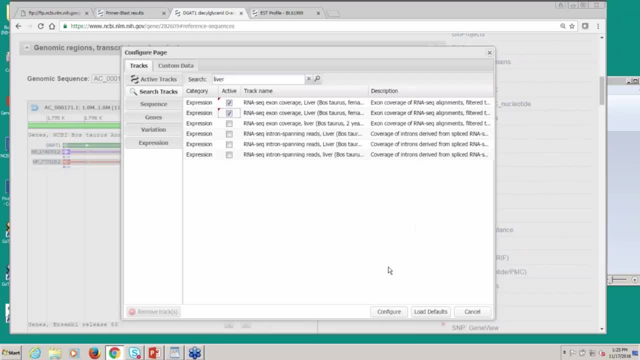 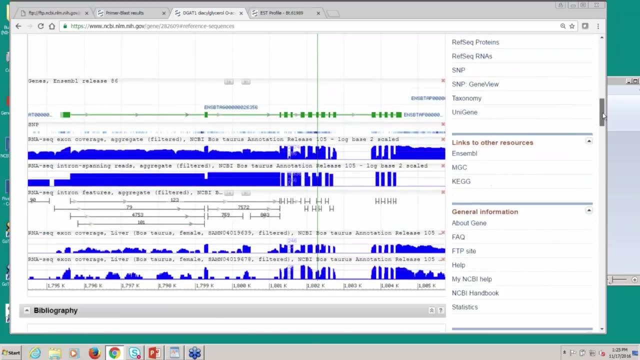 for trying to figure out what the various splice variants are. Let me just go ahead and add the liver track here. You can add more if you want to, to see what the various expression profiles are like. This is what liver looks like. two different samples. 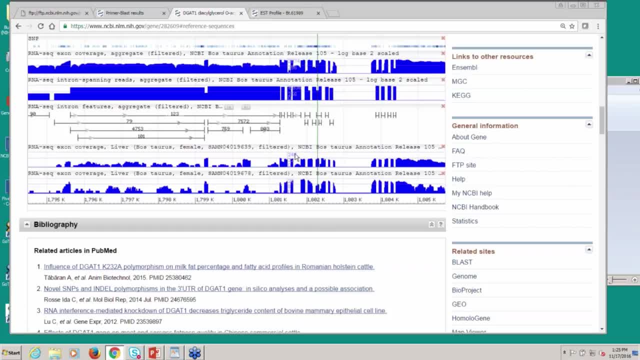 You can compare expression in sort of a rough way here by just looking at the heights of these peaks. Notice that they give you a scale here. I could put another tissue up there and see, for example, if I expected higher level expression. Notice that at this point. 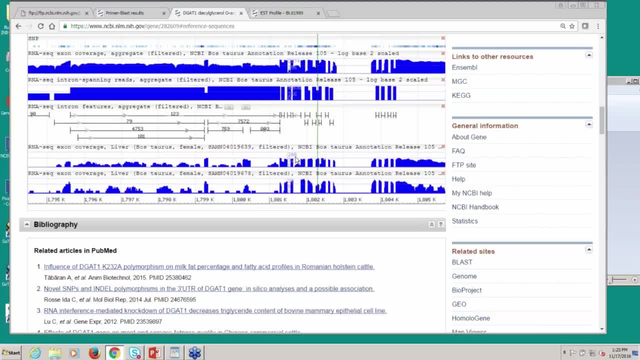 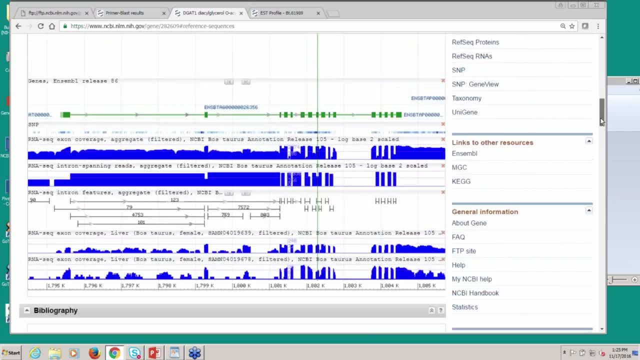 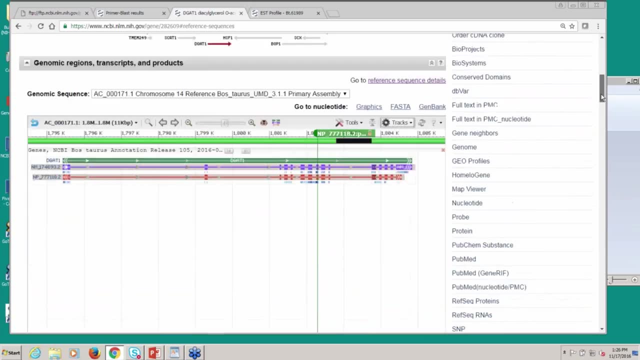 these are log two based scales here. Remember that the high peaks are much, much higher than the low peaks. Another task that people are faced with a lot of times when they're in this kind of situation is to try to find a homolog in another species. 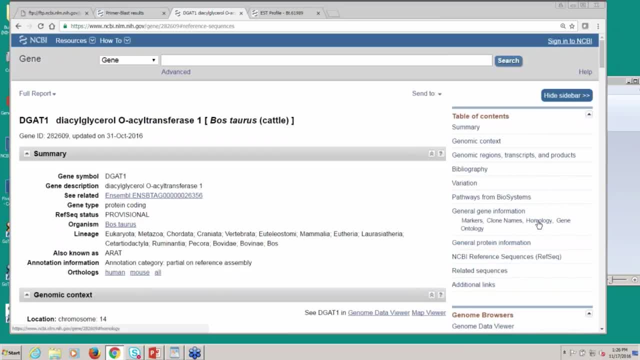 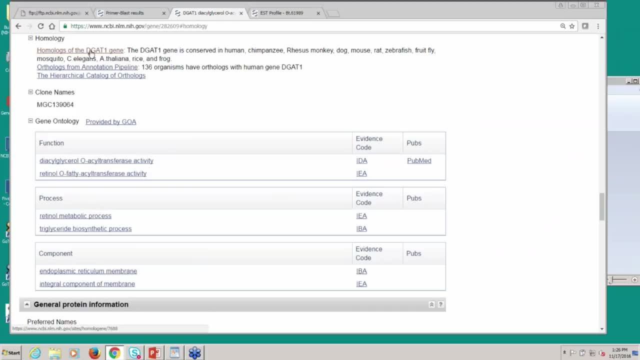 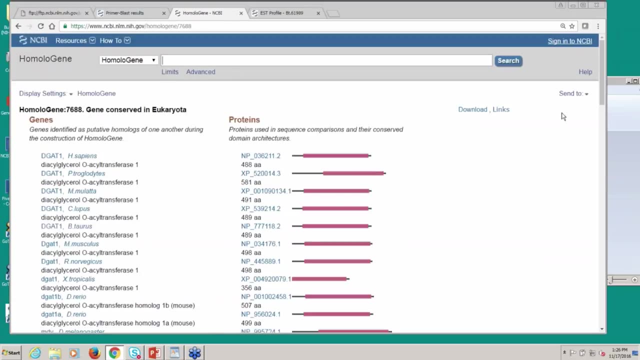 If you go to the top of the gene record. there is a link here to homology. There are basically two ways here of doing it. I could look at the old fashioned database which we call homologene. Let me do that first. This gives me: 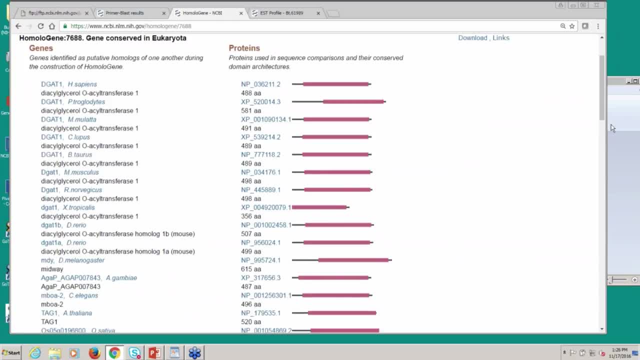 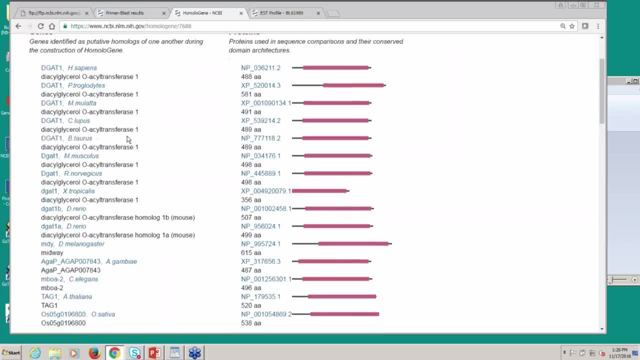 a set of sort of representative organisms. These are based on completely sequenced eukaryotic genomes. This database is frozen at this point. It does give me a way of getting, for example, from cow back up to human. I could do that already in another way. 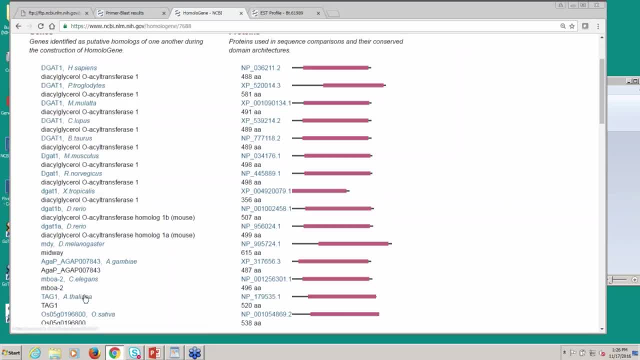 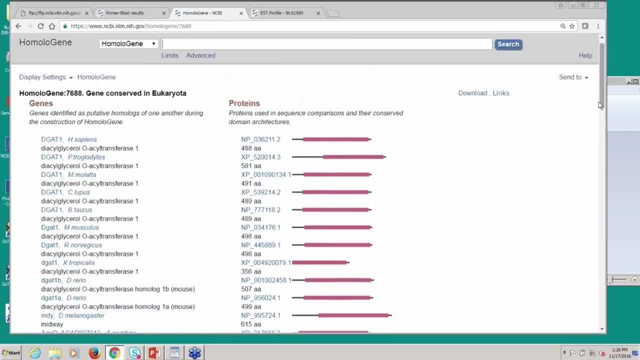 I'll show you that in a second. It also gives me a little bit broader coverage. I can get to, for example, some plant genomes. here There is a homolog and a rabidopsis. Basically homologene tells you about. 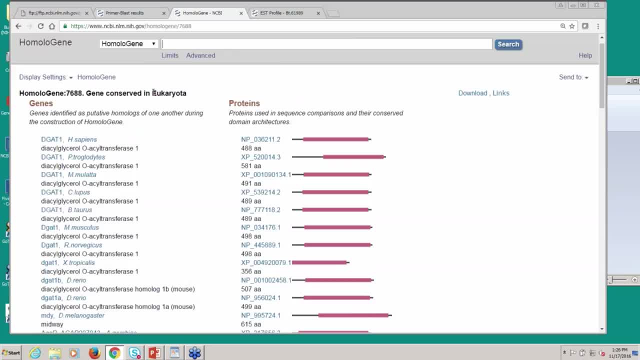 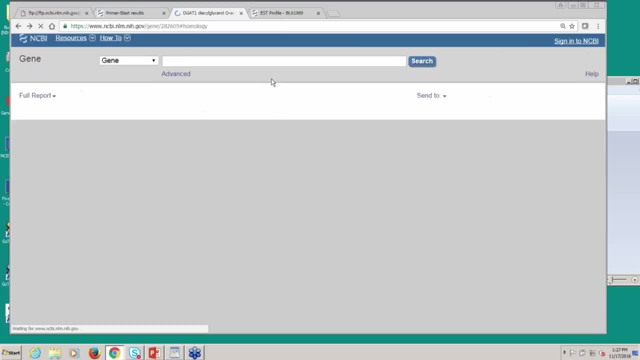 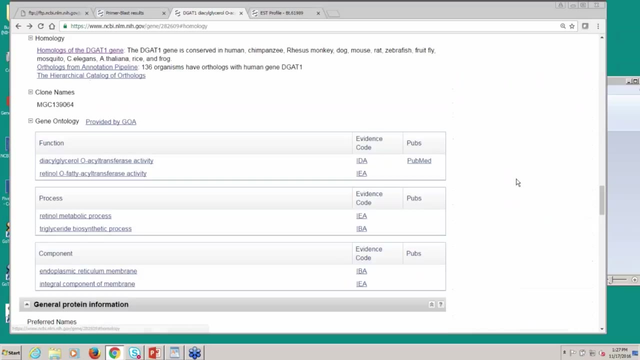 the most recent common ancestor of all these organisms. We expect to find this gene in pretty much all eukaryotes. The other way of finding homologs here, which is particularly useful if you are working with vertebrates, is to use the orthologs. 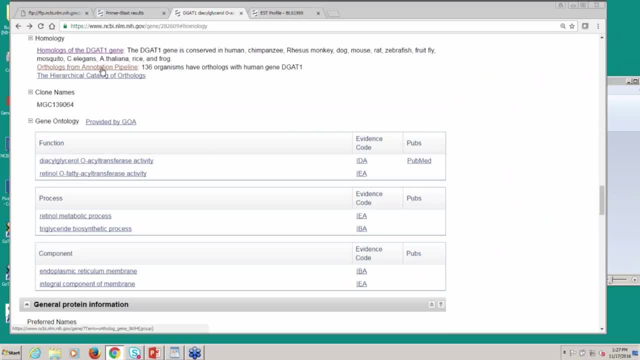 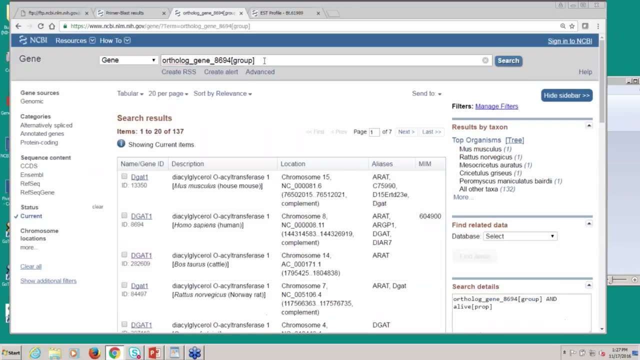 that we have found. when we annotate the genomes, You can see that it says 136 organisms have orthologs with this. This is actually a search that is based on a gene that is orthologous with the human gene. I can add any kind of 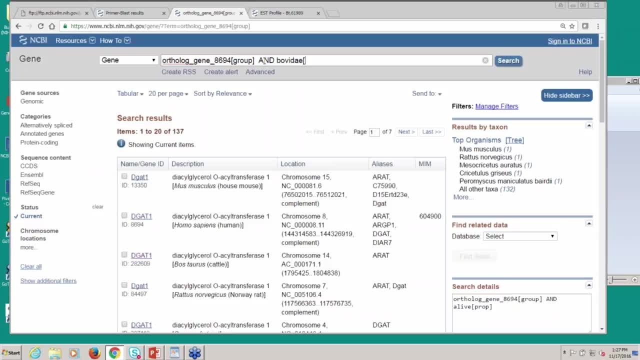 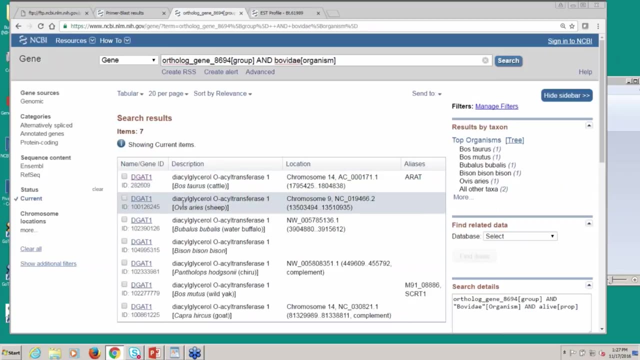 organism search to this if I want to find the corresponding matches. I'm just going to put an organism search on the end of this to find those in the family Bovidae. I can find the sheep and the goat and other members of the genus. 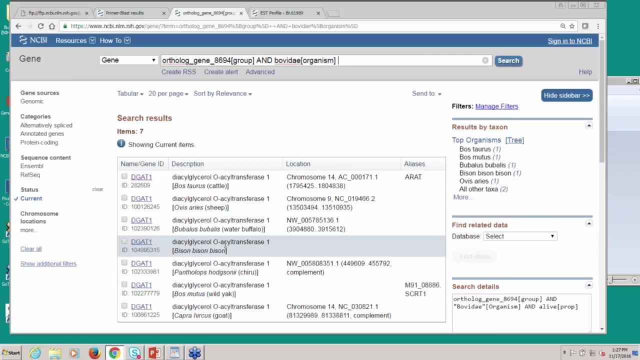 boss, Here is a wild yak. There is also bison here. You can do the same thing, if you want to, for other organisms of interest. The last example that I want to do- I'm going to do it fairly quickly- is to switch over to a plant gene. 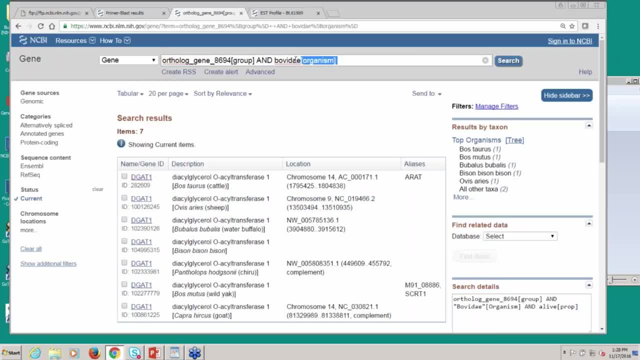 That will give me a chance to show you a geoprofile, Also how to find a homolog using BLAST, which we could do, of course, with the gene that we are working with now, but I'll show you this with the plant gene, The gene that I'm going to work with. 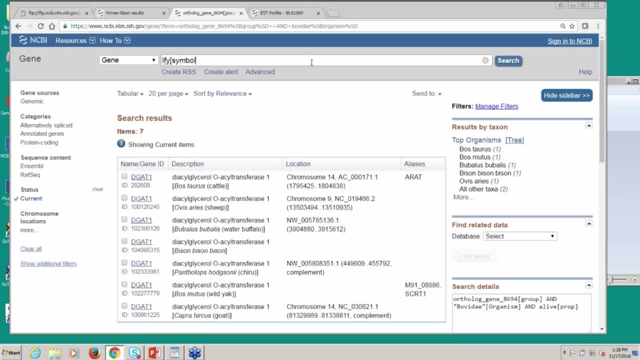 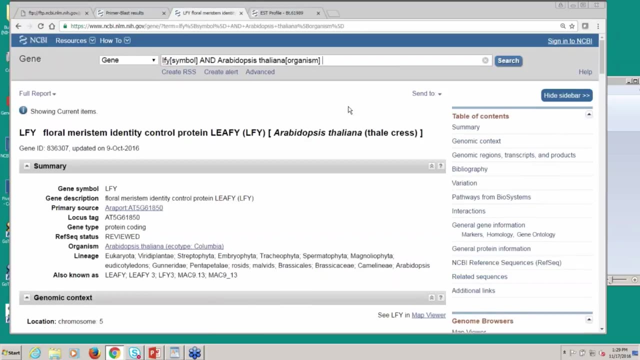 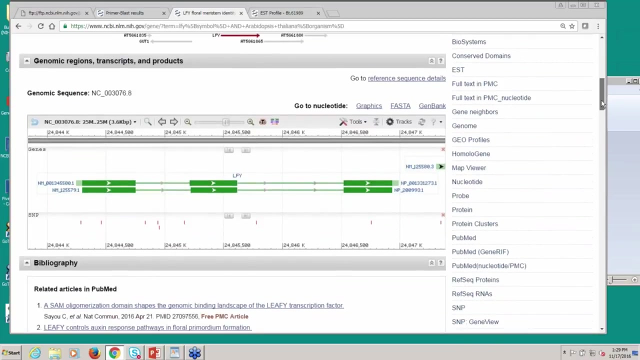 is leafy, which is a transcription factor. I'm going to show you a very useful kind of gene search here, which is this symbol combined with the name of an organism. This looks very similar to the record we saw for cow. This is a gene from Arabidopsis. 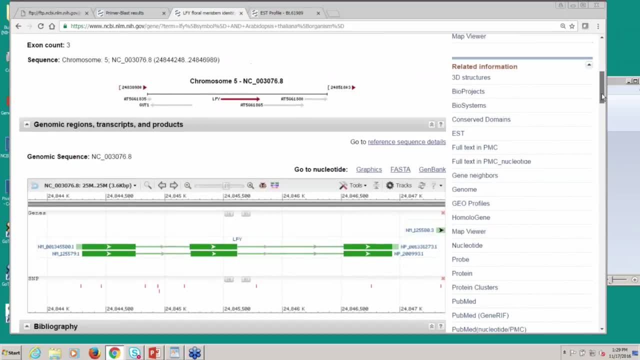 We have access to reference sequences and so on and so forth- What you can do with cow to get very good information. there are a lot more geoprofiles for Arabidopsis, a widely used experimental organism. I can just go here and see what one of these expression profiles look like. 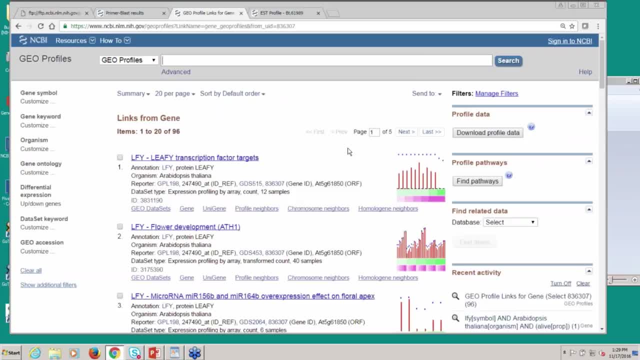 These basically are looking at the genes that are on a particular gene chip to see the expression level. So you're basically taking a slice across that microarray for a particular gene that's got maybe more than one probe in that microarray. What you can do 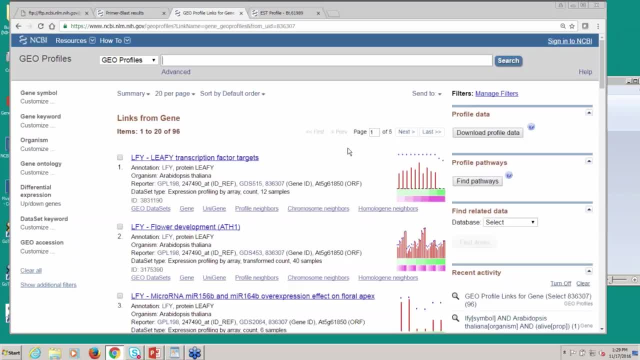 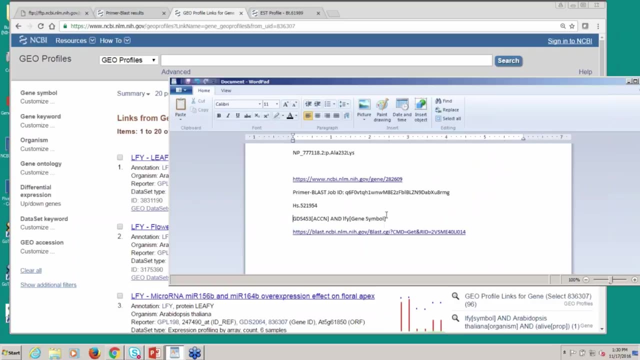 is to associate it with a particular geodataset, which is one of these curated experiments. So I'm just going to go ahead and use the one that later on, if you have some time, you might want to take a look at GDS453, which is basically looking at 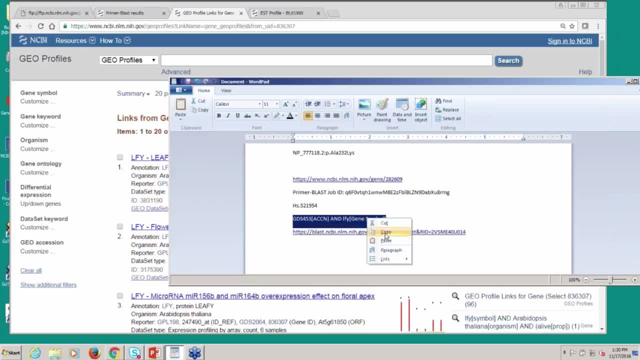 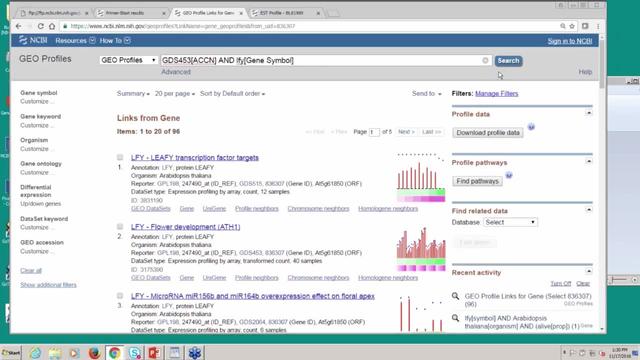 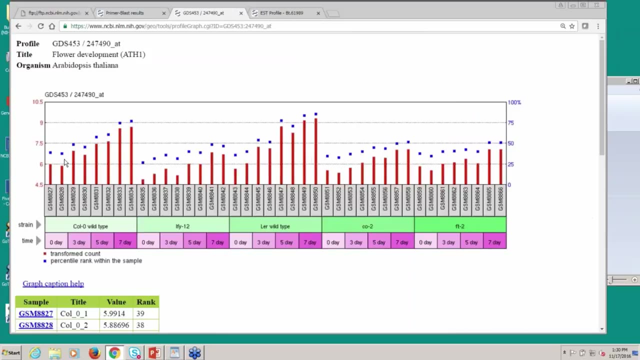 mutant strains of Arabidopsis that have mutations in some of the genes involved in flower development. So I can just run this kind of a search in geoprofiles to get that directly And this shows you a geoprofile and it shows you that the wild types. 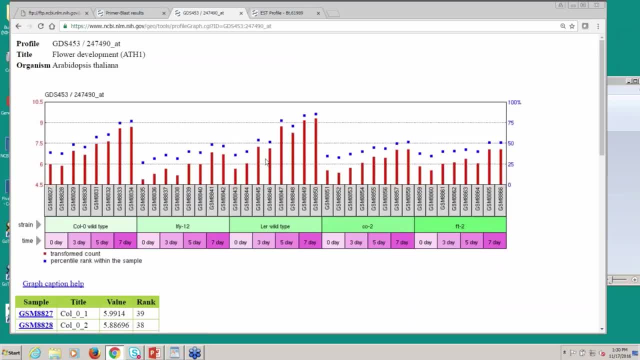 have much more increased expression of this leafy gene, which is involved in flower development, over the day trials that they did here. These are the mutant ones that have mutations in genes related to flower development. Last thing I want to do, or there are two things. 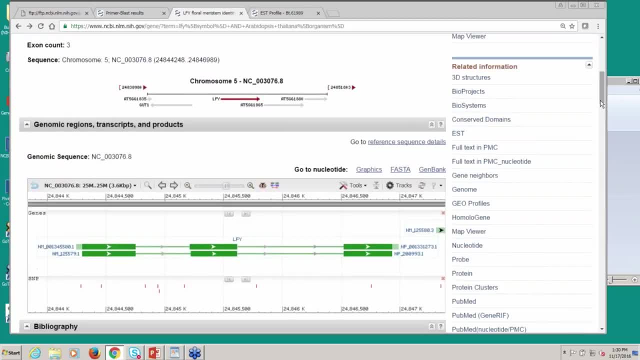 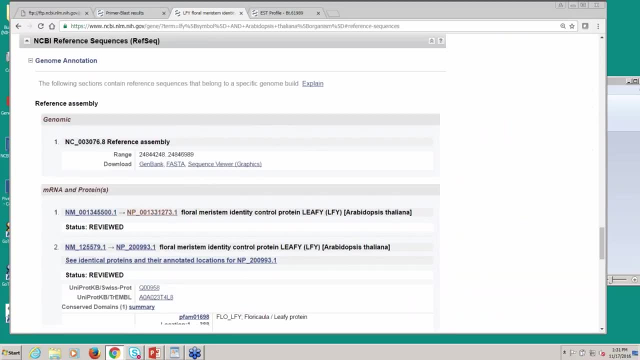 I want to do with BLAST, and that's to go ahead and show you how to find homologs using BLAST. What I'm going to do is go down here to the reference sequence section of the record and I'm going to retrieve the protein record. 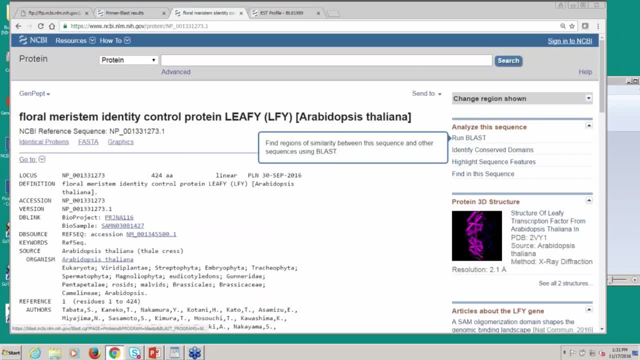 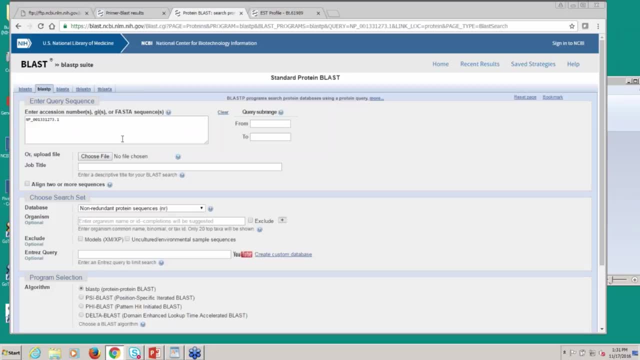 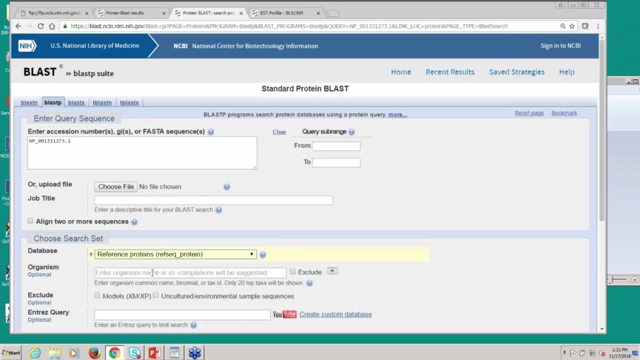 This is the leafy gene product here. I'm going to run BLAST with that. So what I can do with BLAST to find the corresponding gene in another species, which is what my goal really is here- is I'm going to pick our reference sequences here. 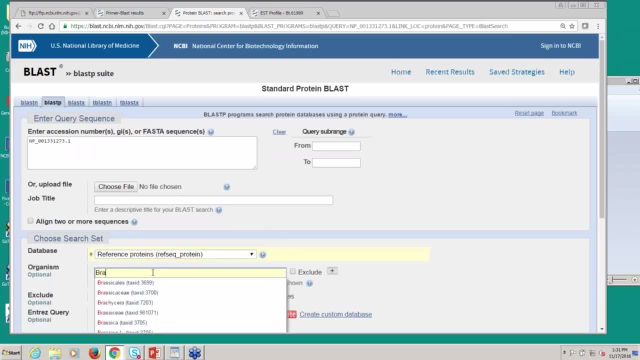 and I'm going to use field mustard to do this. So I'm going to try to find the corresponding gene in Brassica napa. Not Brassica napa. I'm going to find it in Brassica rapa And I can run this search directly. 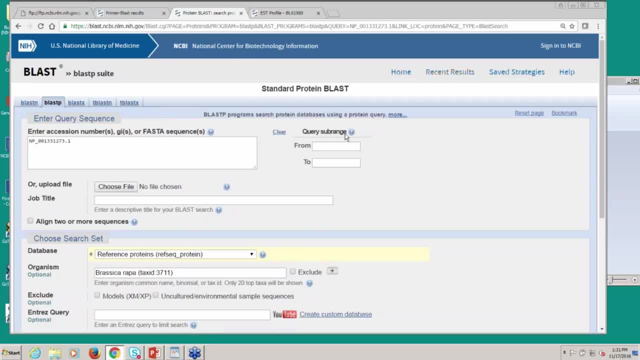 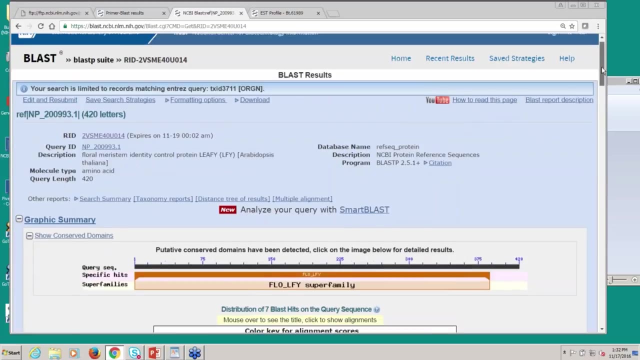 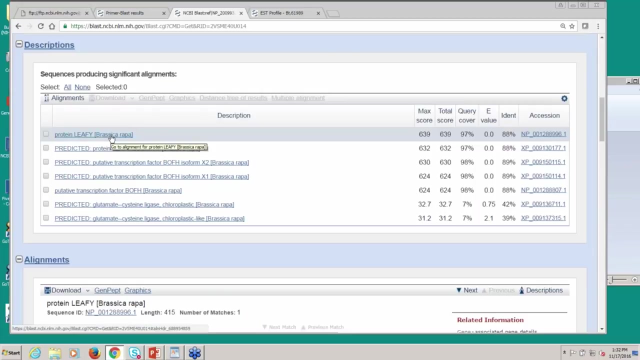 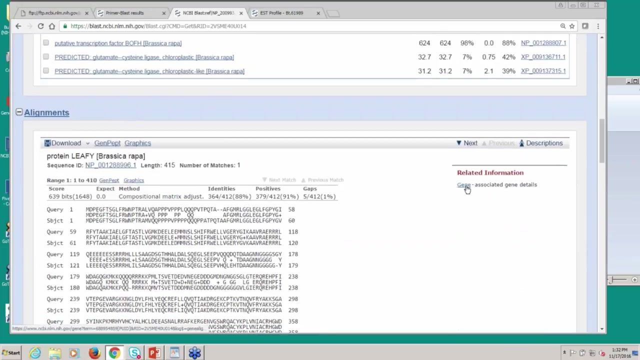 to save time, I'm going to go ahead and load the results, and I've saved those here, And so here are the corresponding match in Brassica rapa And from the BLAST results I have a quick link back to the corresponding gene record. 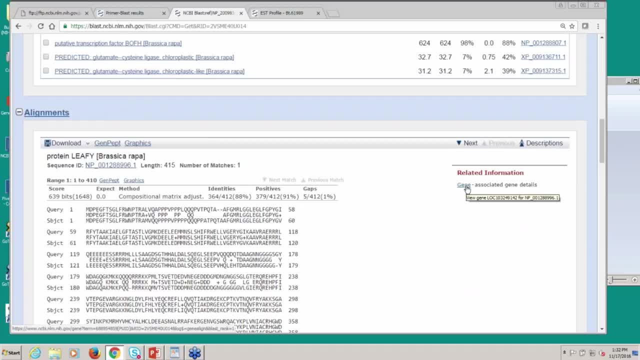 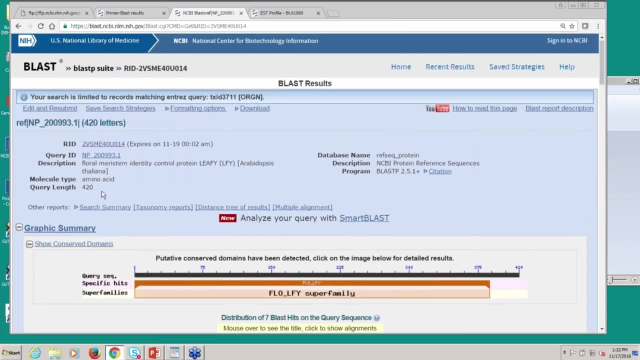 in the gene database. So that's how you would find the plant genes, because we don't have some kind of annotation pipeline for plants doing these kinds of things. The last thing I want to do here is just to show you how to find a structure for. 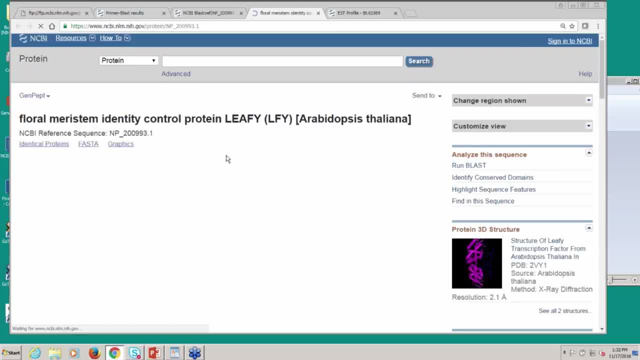 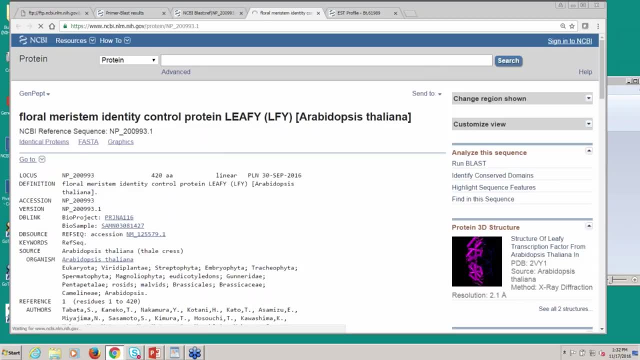 a particular protein. You can do this directly from the leafy gene or you can do it from the protein record. You can see there's a shortcut here to the protein 3D structure. I'll take the first one here If I want to. 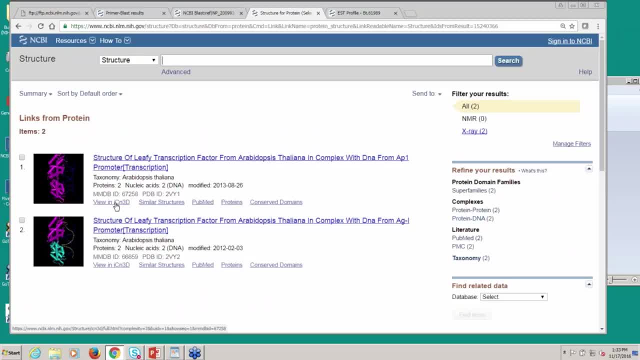 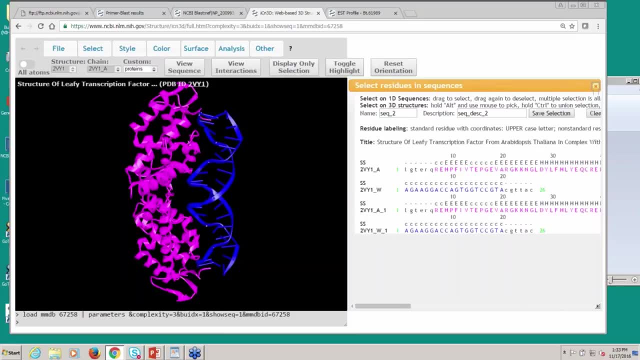 I can just directly view this structure in ICN3D. I'm going to go ahead and do that, And so this is a transcription factor and it binds to DNA, And so you can see that this is a structure that has a crystal structure. 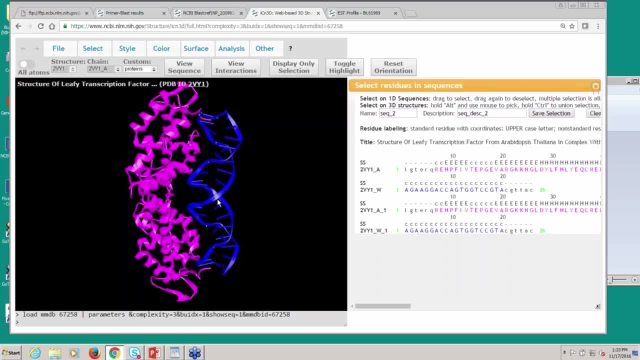 The protein over here is shown as a ribbon diagram And this is sort of a cartoon of the DNA structure And you can change the way these things look, So I could, for example, color the protein by charge. So now the blue residues. 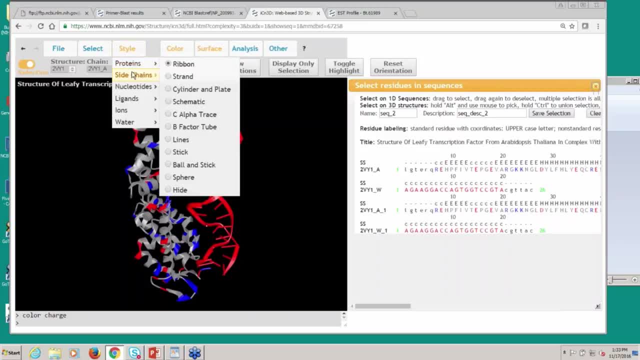 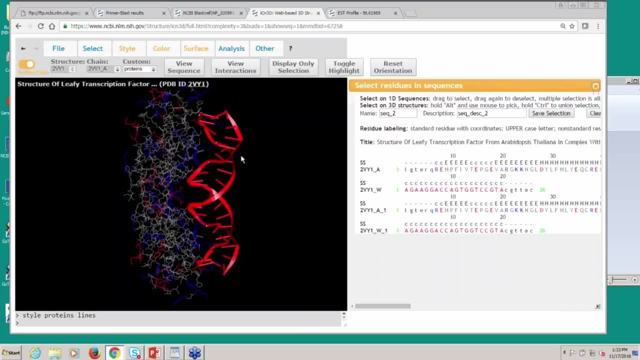 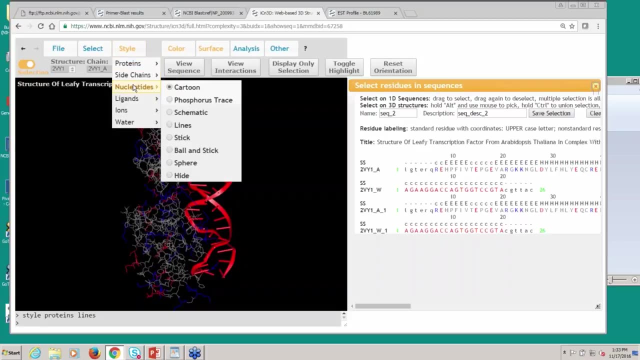 are negatively charged. I can put side chains on them if I want to. I change this to lines And then, if I want to change the way the nucleic acid structure looks, you change that to sphere And I can zoom in to take a look at this. 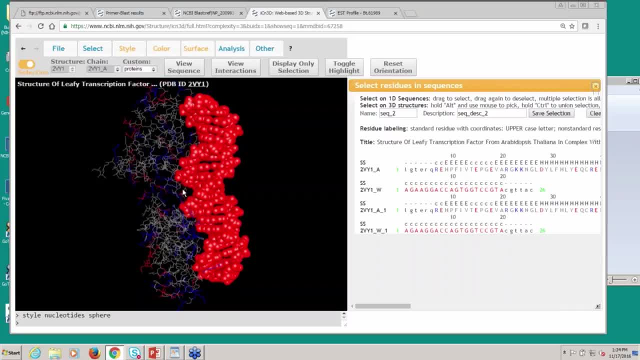 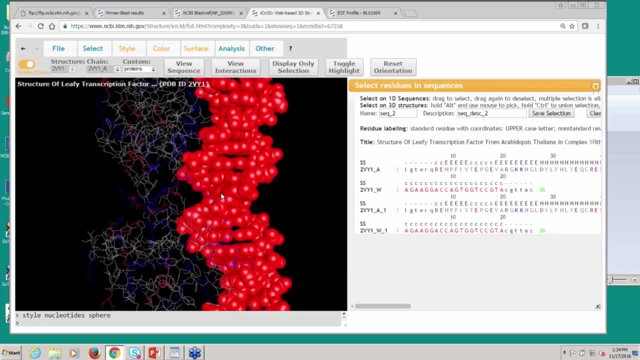 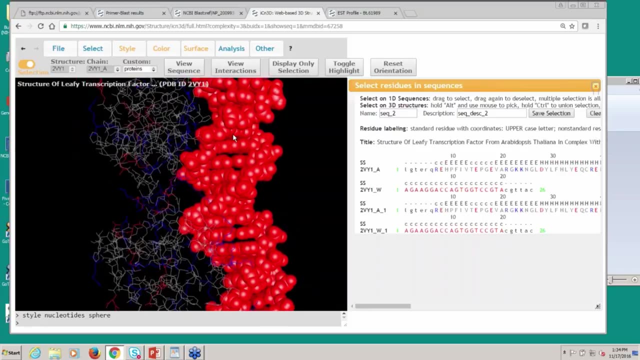 One of the things you might notice that's quite obvious when you look at this is that those negatively charged- I'm sorry, the positively charged- amino acids, the blue basic amino acids, are the ones that are interacting there with this overall negatively charged DNA structure. that's bound to it. 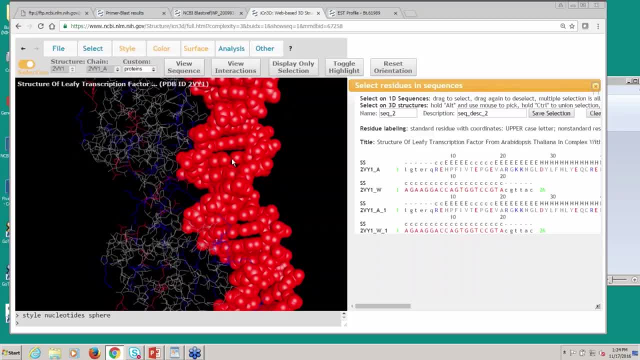 Okay, so that was a quick. what we're going to do is we're going to go ahead and take a look at this. Okay, so that was a quick whirlwind tour of some of our resources, And what I want to do now is to turn this over to Ben. 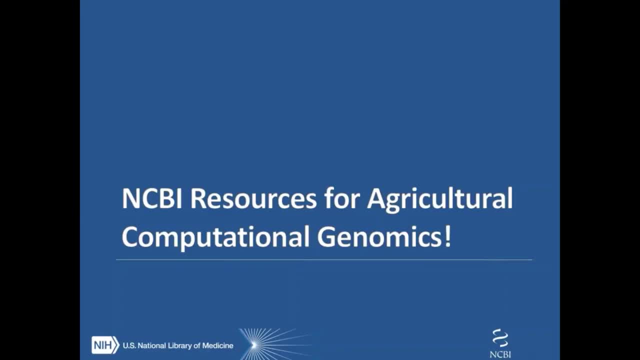 Hi everybody. I hope you enjoyed Peter's portion of the talk. For the next 15 minutes or so I'm going to talk about resources for really doing computational genomics on agriculture. Most of the resources I'm going to talk about are command line. 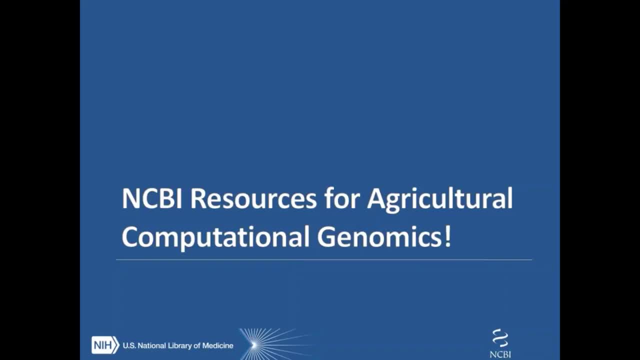 or Linux based. If you are not familiar with Linux and would like to be, there are many fantastic online resources. We have some videos on learning Linux, Or you could turn to say something like Software Carpentry, which, in my personal opinion, is a fantastic way. 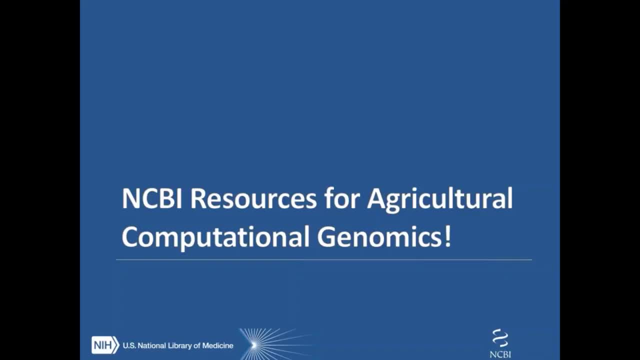 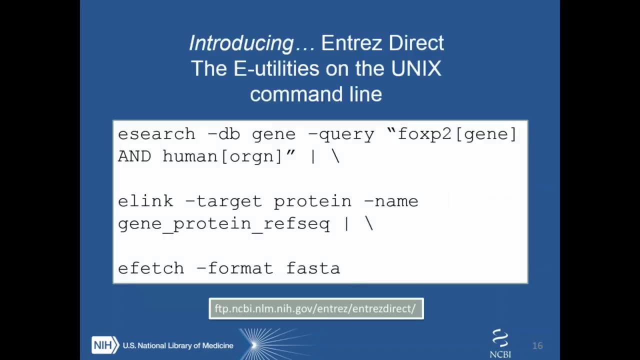 to learn Linux, Alright. so the first thing I'm going to show you is an API that we've adapted for the command line called EDirect. So many of you are probably familiar with the E-Utilities API, where, in a Perl or Python. 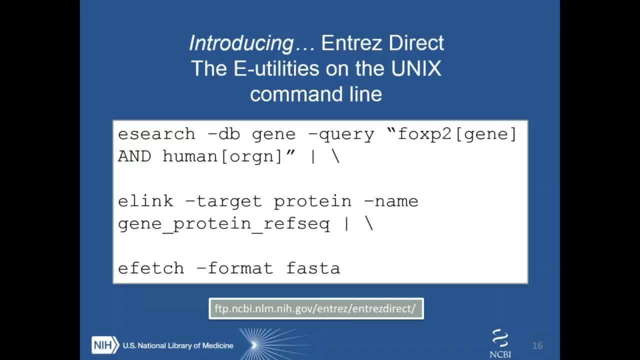 script. you could script up URLs and find out about lots of things, But now you can do that directly on the command line. And if you Google NCBI EDirect, there's a very useful document that will show you how to download a Perl script. 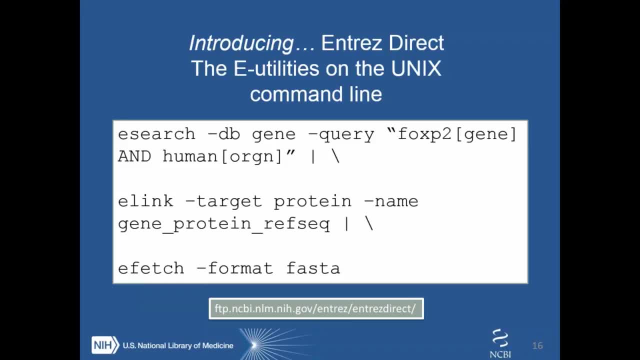 And when you configure that Perl script in your Linux environment, then you'll be able to use EDirect on the command line. So this is an example. granted, this example is for human. but say you wanted all protein FASTAs for the human? FOXP2. 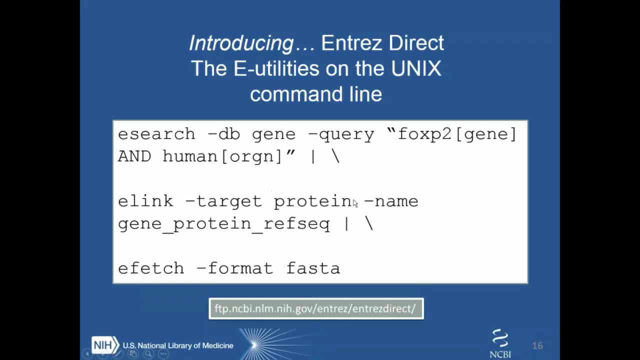 gene, you would have it actually go through there. Now, one thing many people ask me for- whether they're in the metagenomics community and they're interested in plant or animal microbiomes or from other types of communities- is- they say, Ben, I would like to get all. 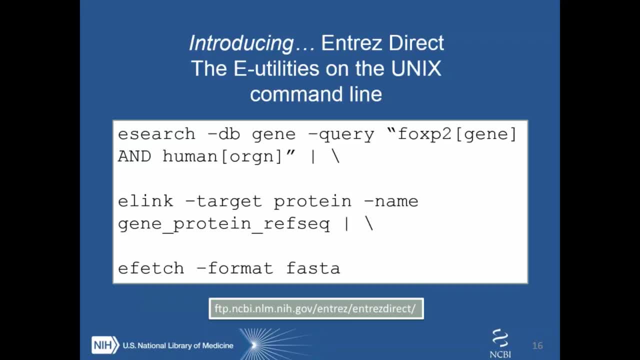 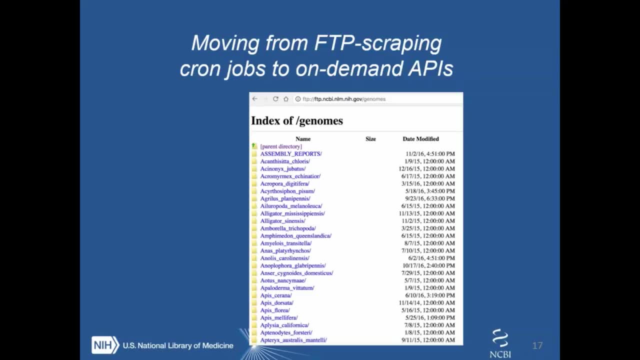 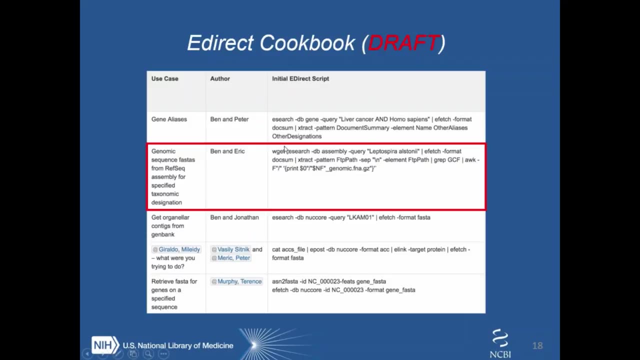 the FASTA sequences for a given taxonomy, And one way you could do that would be to go to the Genomes FTP site, but that's a bit complicated. But another way you could do that is by using this short command here, which basically: 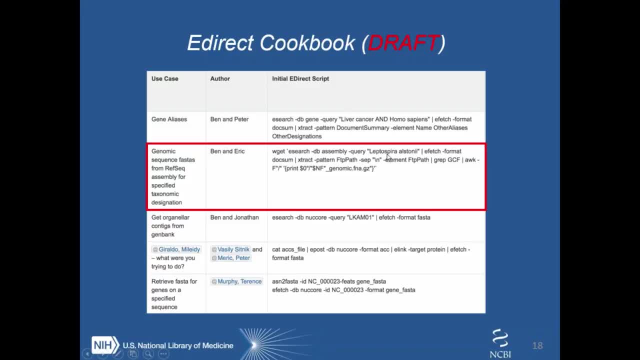 leverages EDirect and I can send this to anybody who's interested What this does and these slides will be available in just a couple of days. this leverages EDirect to go ahead and get all of the FASTAs for any particular. 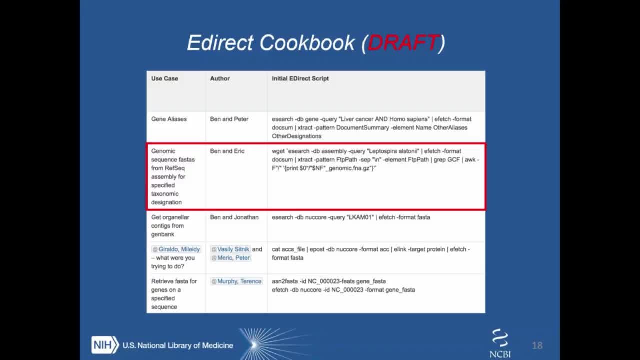 sort of genus and species you're interested in And, of course, you can swap this bacteria in quotation marks for any particular genus and or species that you're interested in. We have a whole bunch of these EDirect commands and we're going to be putting a cookbook. 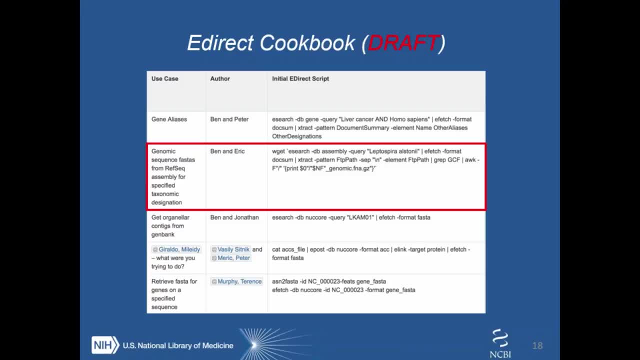 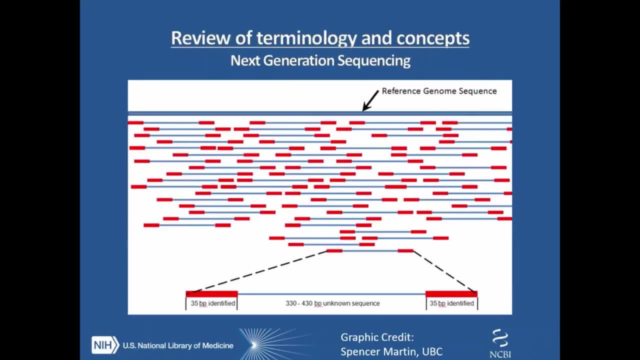 most likely out on GitHub, so that can be a community resource. So watch NCBI news for that. That's something I'm particularly very excited about. Alright, so what I'm going to talk about for most of the rest of the webinar is: 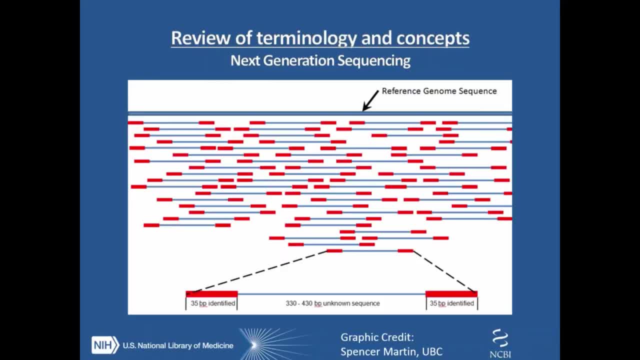 next generation sequencing. So I hope many of you have access to next generation sequencing and I'm sure many of you are probably using it to answer questions. What we're typically doing with next generation sequencing is we're taking short, usually a bit longer than. 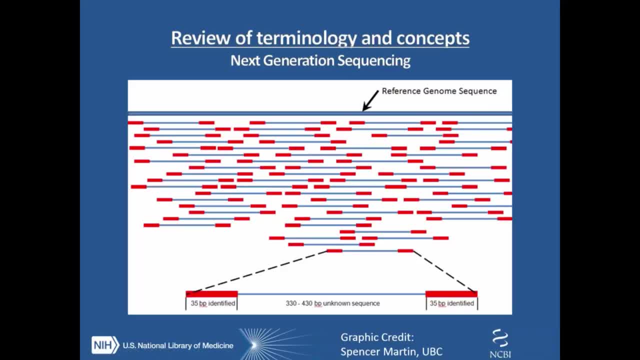 this now somewhere on the order of 100 to 150 nucleotides, with about a 400 base pair spacer and then another 100 to 150 nucleotides. We're taking these things and we're either assembling them or mapping them. 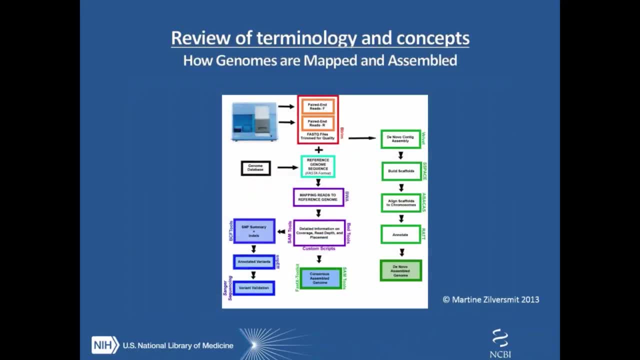 to a reference genome. So this is just a simple diagram of mapping and this shows basically that there are two paths for this. One is mapping to a known reference genome and then calling variants, And I'm going to show you how to do that with some of the stuff in our 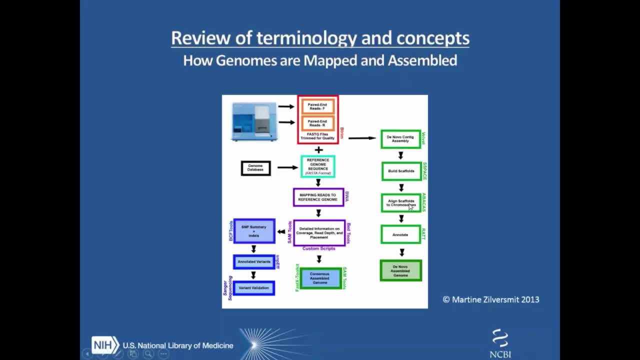 databases, And then also there's assembly. Some people have been asking me questions about what to do with their assemblies and how to submit them to NCBI, And if you're interested, what I would suggest starting with is submit ncbinlmnihgov. 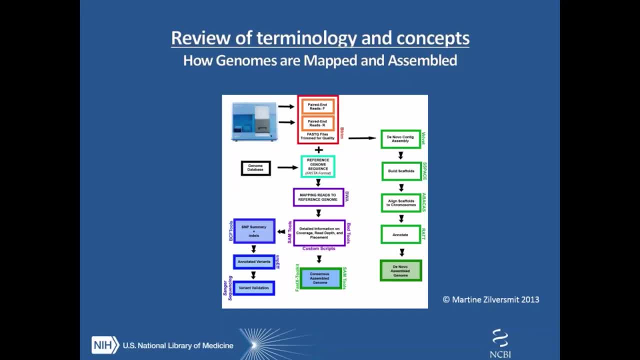 You can also check out previous webinars that we've given on sequence submissions. So if you go to our webinars page, click on the archive webinars tab, then you can actually just search for submissions And it'll pull all of those up. 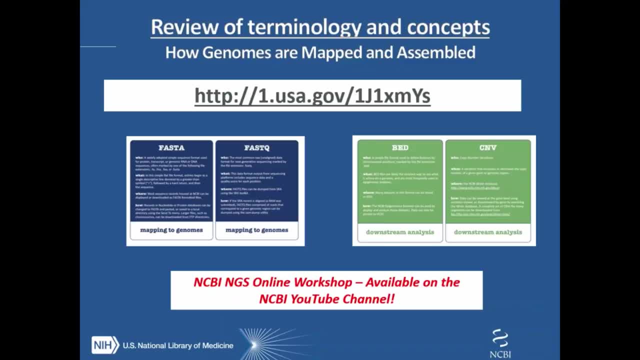 If you're interested more in genomics and you don't know what the names for the different kinds of files are, we have a glossary- It's available here, thanks to Shannon Green for her help with that- And also we have a basic next generation sequencing. 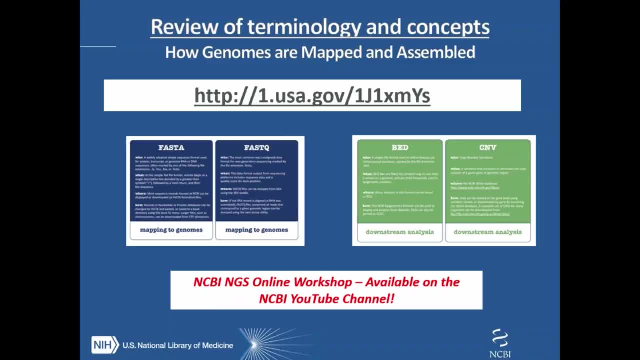 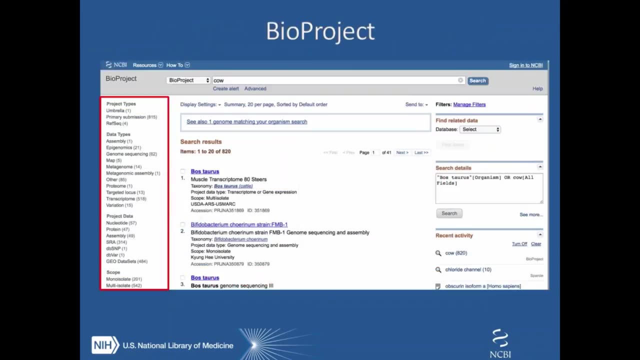 online workshop. It's really sort of easy to use and there's a basic Linux component in that. You can find that on the NCBI YouTube channel. Just go ahead and Google search for it. It should come up relatively easily. So I'm going to talk a little bit. 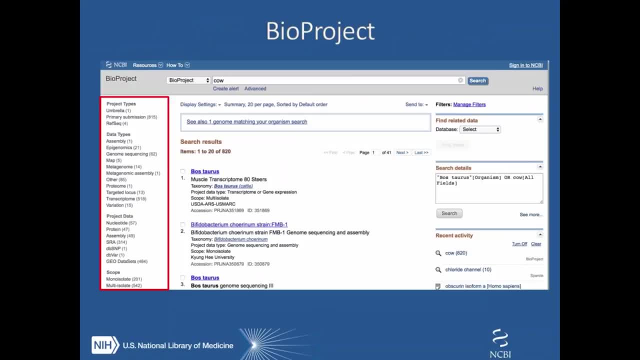 about where a lot of our genomic information lives. The first place I like to start if I'm looking for genomic information on a particular animal or plant is with BioProject. The really nice thing about BioProject- so you can search through a whole bunch of 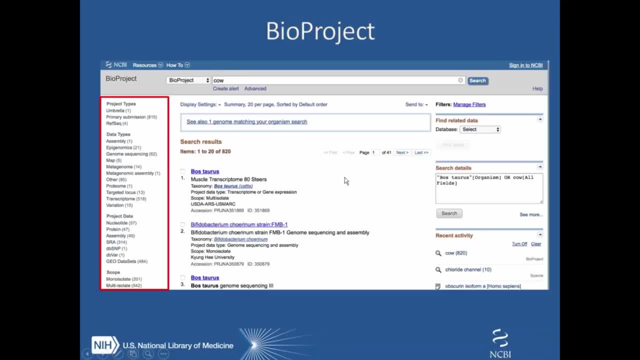 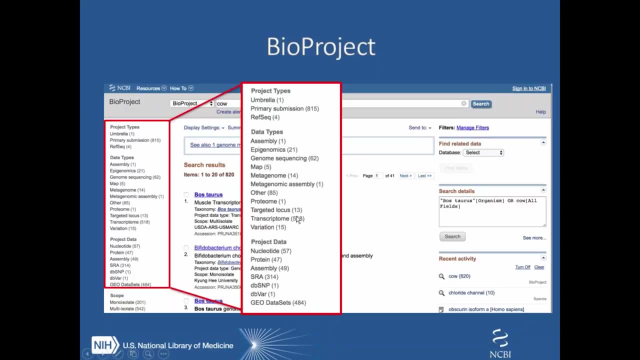 projects related to your subject of interest. In this case I picked cow, But then it'll also break it down by projects on different things. So, for example, we have 518 transcriptome projects on cow. So that's something particularly interesting. It may be interesting to you. 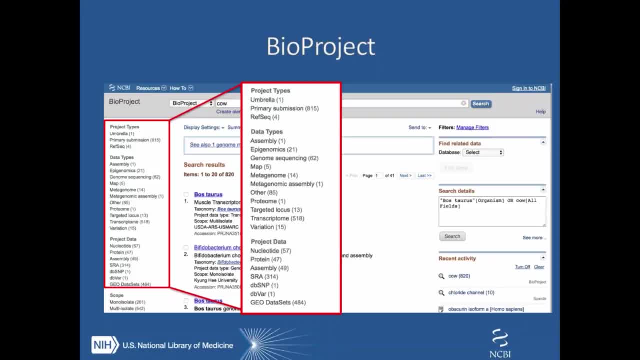 And those are divided between microarray and RNA-seq, And I'll show you how specifically to get into the RNA-seq data, in a couple of slides. We also have quite a few epigenomics projects, as well as sequencing projects, So things to check out. 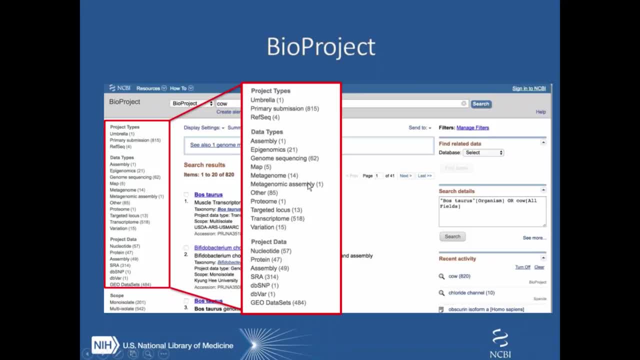 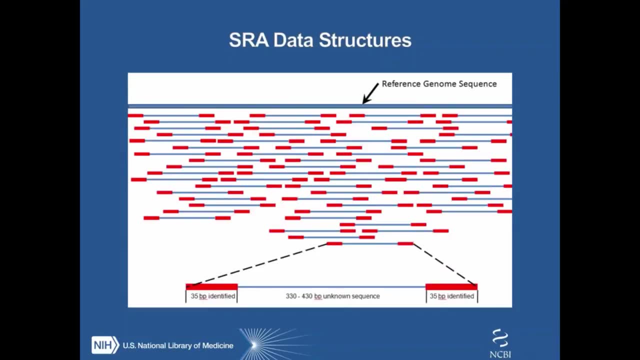 And then we have some metagenomic data sets for cow which I would imagine many of you are very interested in. So we keep our genomic data in a structure called SRA. SRA allows us to compress the data a great deal, But on the other end, for those of 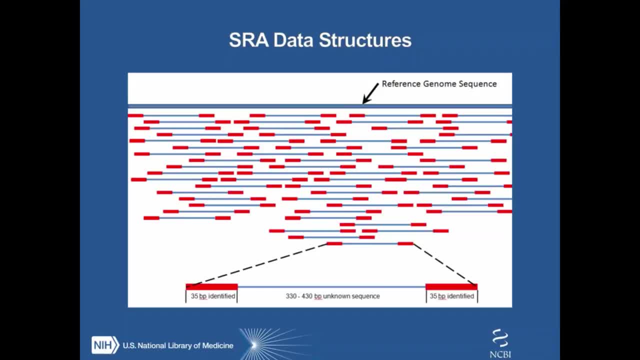 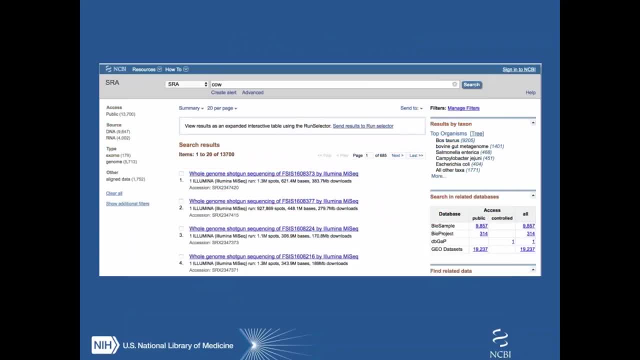 you who are pretty savvy. the nice thing is that you can stream the data to an endpoint And I'll show you what I mean just in the next couple of slides, Or, I'm sorry, in a few slides, when I show GATK. 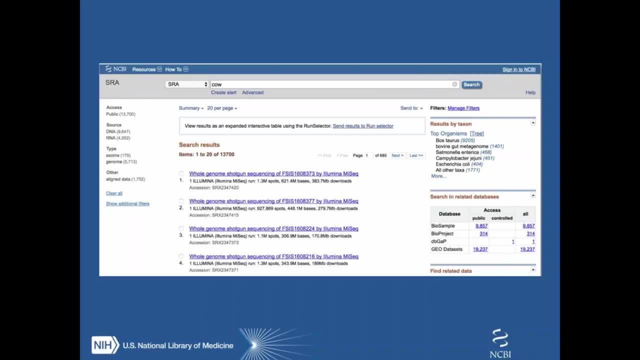 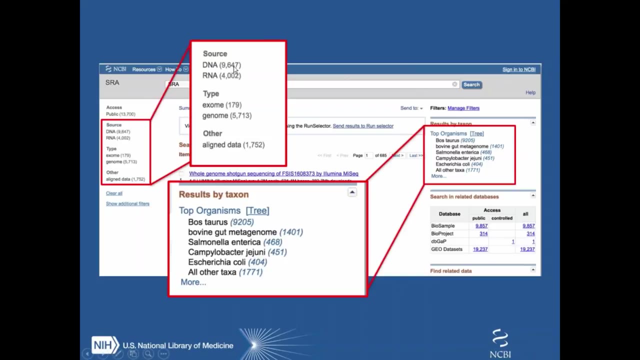 So say, I go to the public SRA and I search for cow, I get 13,700 results. So that means there have been 13,700 individual runs on the cow. Now I can see two things. One: about 10,000 of those are for DNA. 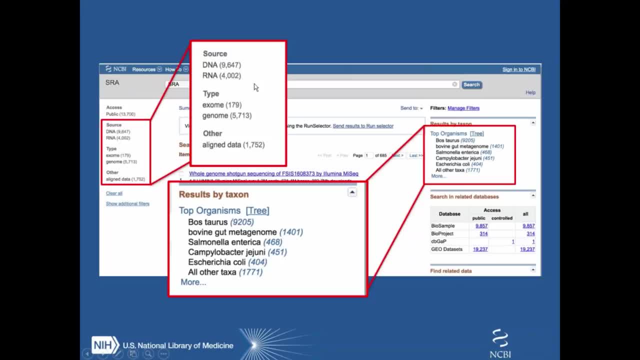 and about 4,000 of those are RNA-seq, So I think that's pretty exciting. There's a lot of data to go through for cow And in the next few minutes I'm going to show you how to go through that data. get into that. 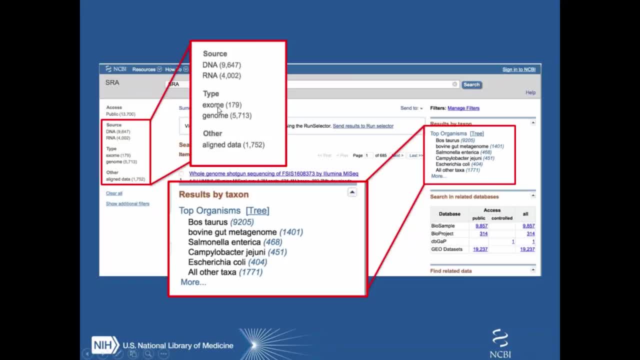 data relatively easily. Also, there's a lot of whole genome sequence for the cow. There's not a ton of exomes. Exomes tend to be used in sort of the human clinical genomics realm, but not necessarily as much, And this will be important as 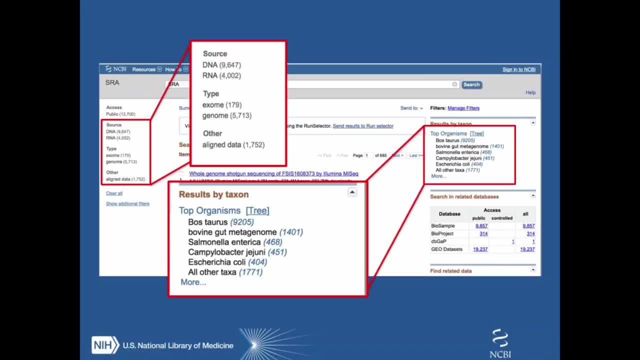 we get into it. Some of that data is aligned, probably much of the DNA-seq. So about somewhere on the order of 15% of the DNA-seq data is aligned. Most of the RNA-seq data and much of the DNA-seq data is not aligned. 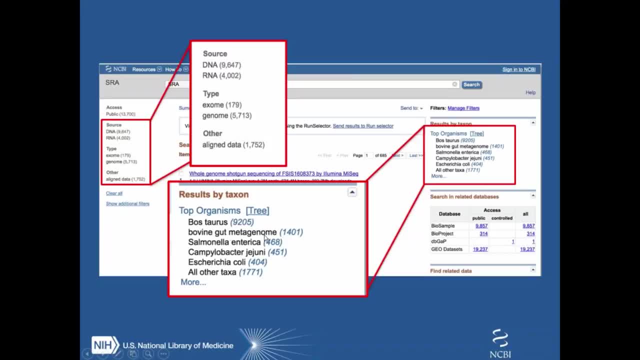 We can also see a breakdown by organisms. So of course there's bovine gut metagenome. We have about 1,400 sequencing runs from the gut metagenome and about 9,200 from the cow itself. Some of those are going to be. 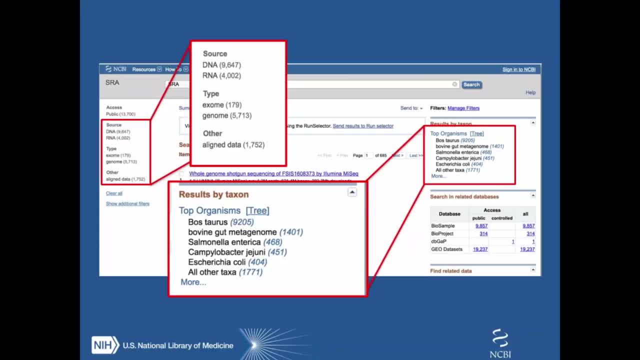 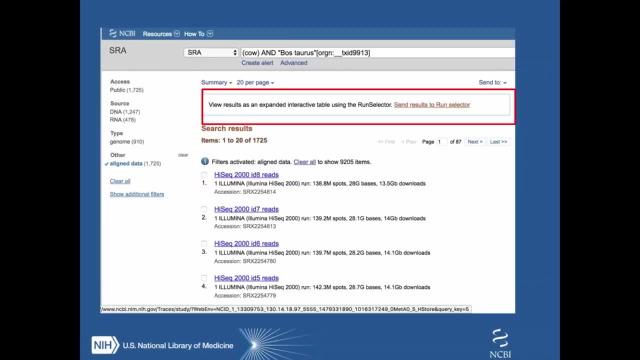 exomes. some of those are going to be targeted regions of the genome and some of those are going to be whole genome. But the really nice thing when we start to dig into this is, say I click on the cow as an organism per se, what I can then do. 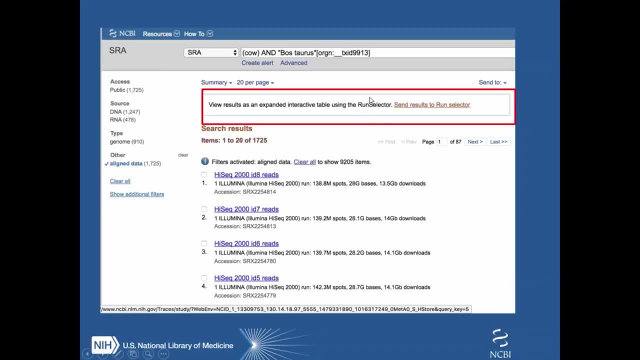 and I click on align data. so now I'm just looking at the aligned data. I can send the results to the NCBI run selector. The really nice thing is this gives me a very clear view of the metadata for these particular genomic data sets in SRA. 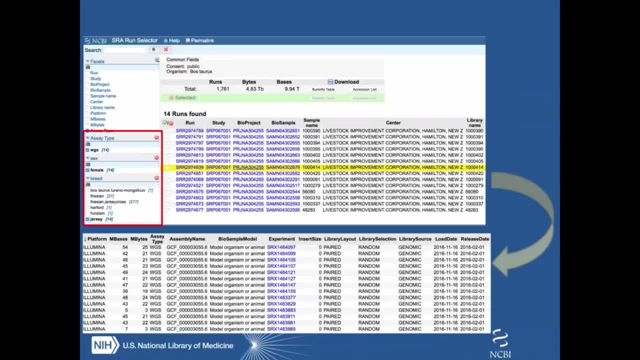 So here I can take a look at that and I can see I can narrow down on all of these facets. So here I know that there's 1,700 runs which I showed you before in the previous slide. so there's about. 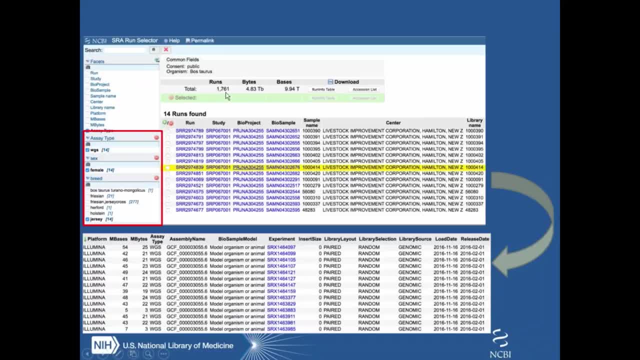 1,700 runs. Sometimes there's technical replicates. that's why there's a few more here than there are in the 1,725 number. But I can narrow them down relatively quickly. So for example, if I'm only interested in whole genome sequencing, 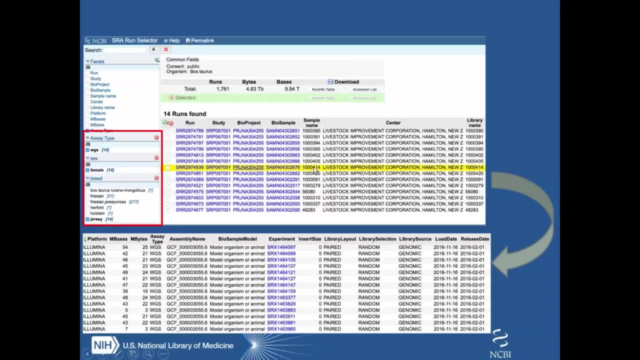 in female Jersey cows. I can look at that right away And I can see that here I have 14 aligned sequences from female Jersey cows And I can see by the bioprojects that all of these were done by the same group in New Zealand, which is not particularly. 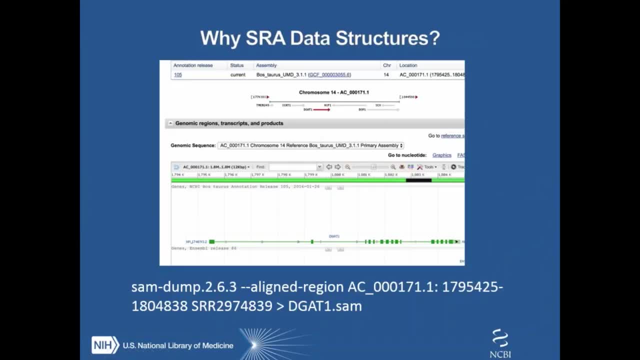 surprising. So why do we have SRA data structures? Well, one really nice thing is that if it is aligned, what I can do is I can just slice the things out. So here's the accession number for cow, chromosome 18 with the. I'm sorry. 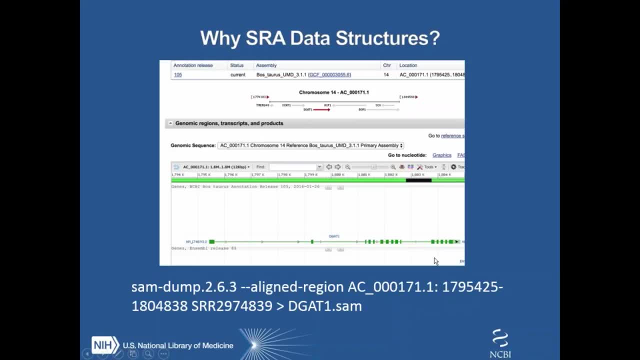 14, with the reference that Peter was talking about earlier. And here I have the region, and what this will do is simply slice out a SAM file from the region that I'm interested in in this aligned genomic data. The other thing I can do with aligned 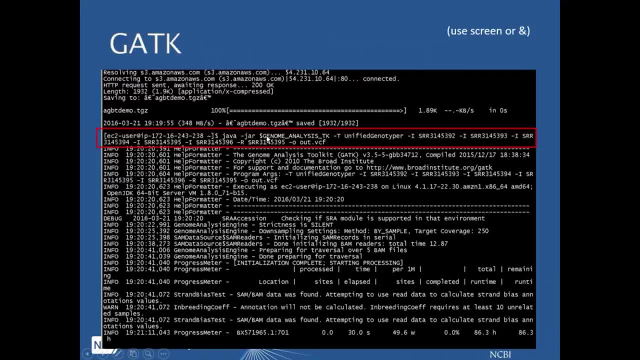 genomic data, and I'm very, very excited about this is that I can use GATK, which is the most popular variant caller in the world right now, And what I can do is I can tell it the SRRs These particular examples. 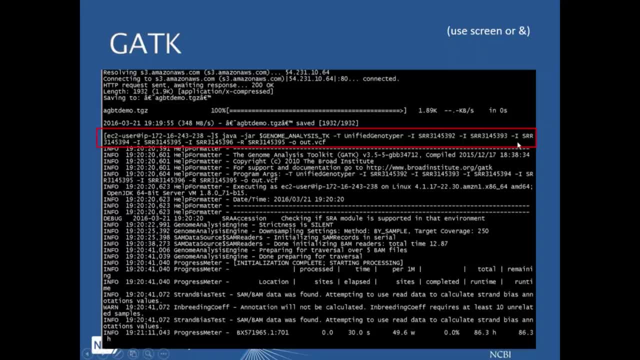 are humans, but they'll work for cow too. I can tell it the SRRs. I'm interested in put them with "-i" and then a space for the SRR. By the way, if you're confused, this is relatively. 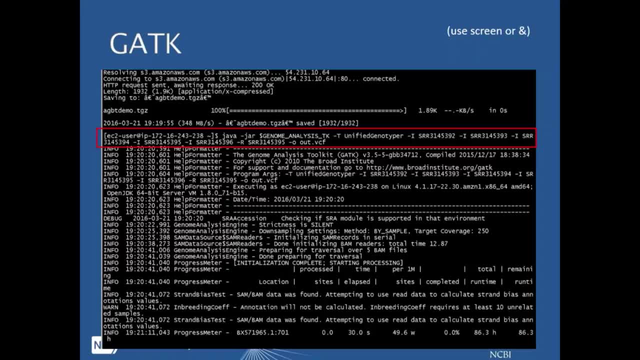 advanced. So don't worry, you're probably just at an earlier stage of your bioinformatics learning. I can also put the reference here and it will recapitulate the reference from that SRR that I give it And that's very exciting for any of you. 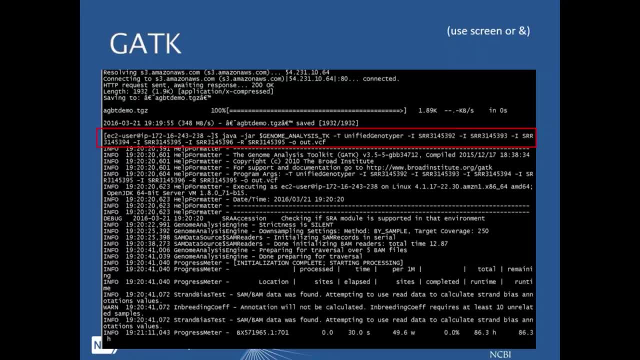 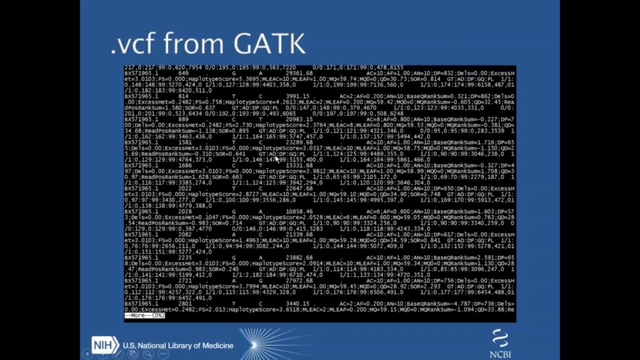 who have tried to use GATK with other people's data or public data. That's a new service we offer And, as you can see here, I get a regular VCF file. If you don't know what a VCF file is, that's okay. 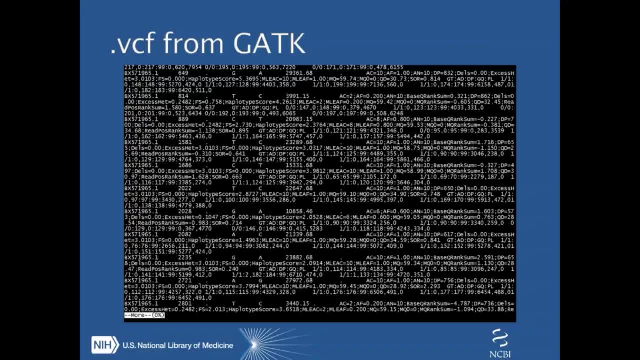 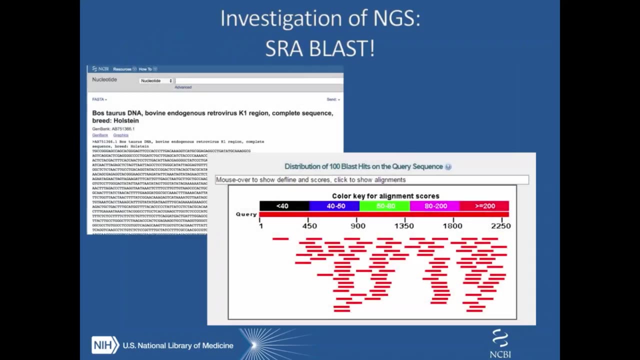 but please refer back to our glossary. It's very in call format and it tells you what the different variants are relative to the genome. It gives you a whole bunch of other information. However, what if that data is not aligned? You know, as we. 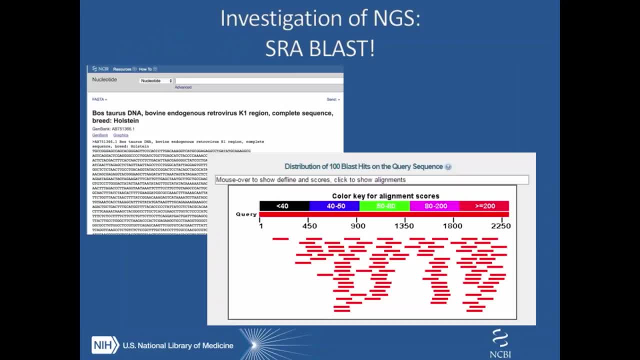 saw, 85% of the DNA data wasn't aligned. almost 100% of the RNA-seq data wasn't aligned. So what do we do then? Well, what I am proud to say is: now you can do BLAST, And this is. 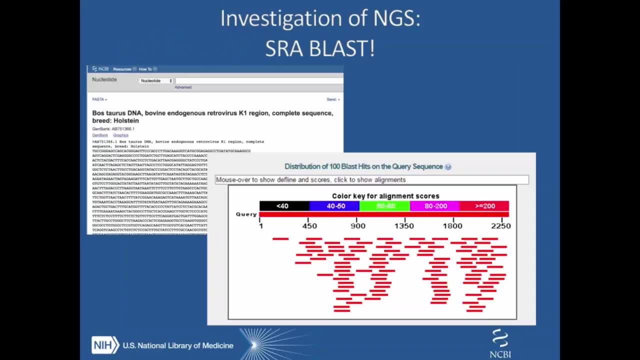 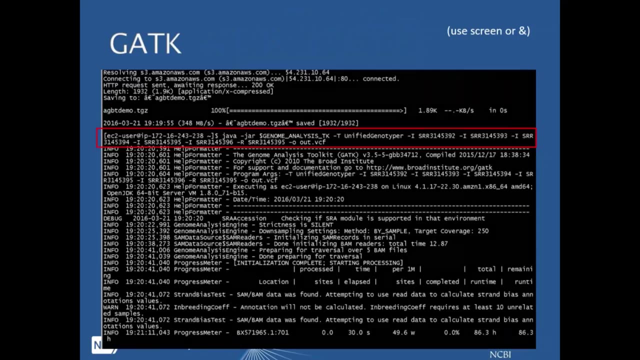 very exciting to me because SRA-BLAST works on both the. it works on both the graphic user interface or the web, as well as on the command line. if you're doing a lot of BLAST searches And when you're in SRA, 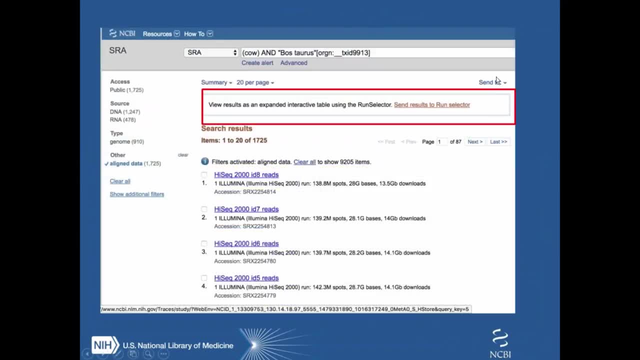 if you click this send to button, it will give an option to send these runs to BLAST. But please select particular runs if you're going to use that option. So if I were to select one and two here, open up the send to menu. I can send them. 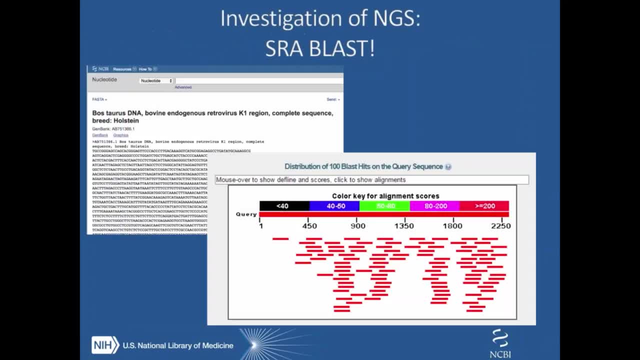 to BLAST. That's something that I think is very exciting and, frankly, sort of democratizes genomics, Because anybody- I believe any of you- are probably capable of doing a BLAST search today, And what this means is that you can do a BLAST. 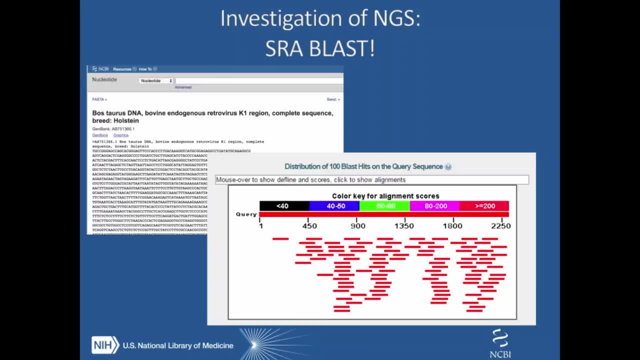 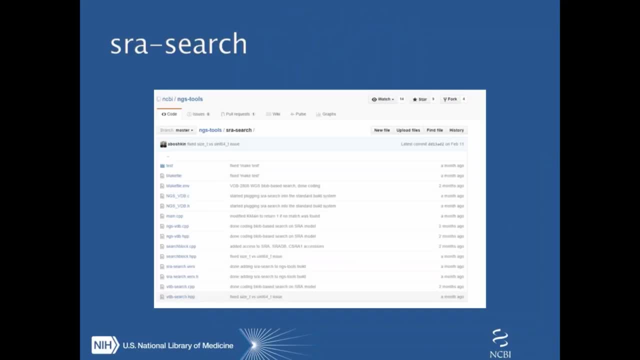 search into unaligned next generation sequencing reads today. So if you're fairly advanced, however, the other thing you can do is go to GitHub and clone the NGS tools repo. If you don't know what that means, don't worry about it. And if you do, 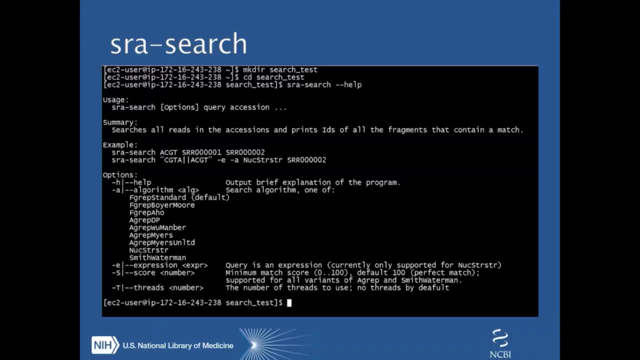 that then you can prepend your BLAST searches with SRA search. Basically, what this is is FB For SRA, And that's something that's very exciting to me because you can search very quickly. So if you had a virus and you were interested in, 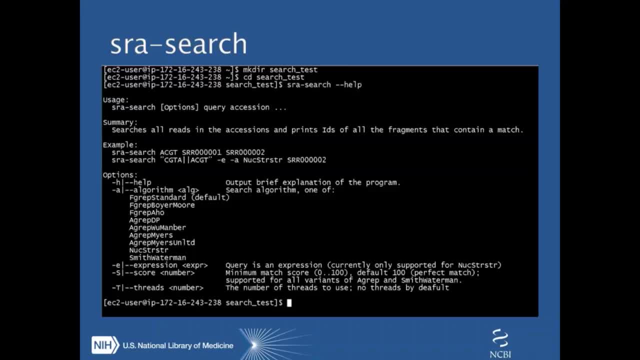 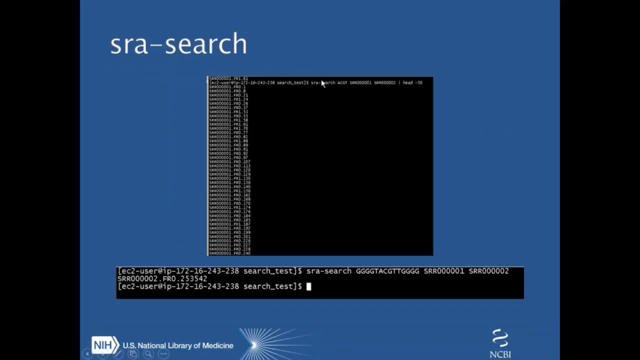 particular k-mers. you wanted to search into particular genomic projects. that's something you could do very, very quickly and very, very easily. This is just showing an example. This is just the very top of a search and these sort of initial. 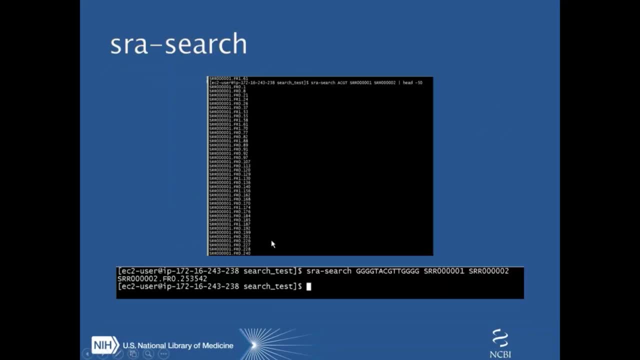 accession numbers for ACG, And here I can see that I have these things. I can make more specific searches and, as I'm sure any of you who are mathematically minded will intuit, that when I go out to something on the order of a, 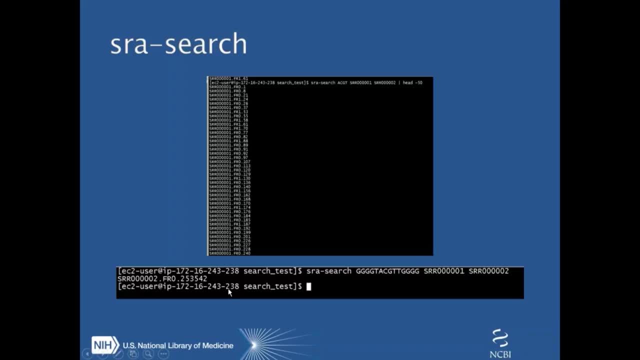 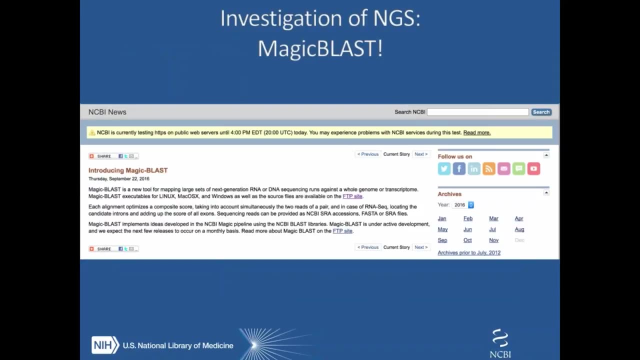 14-mer search string, I start to get to unique hits. So that's something that I hope is useful to you guys If you're interested in RNA-seq or DNA-seq. to some extent we have a new type of BLAST we call 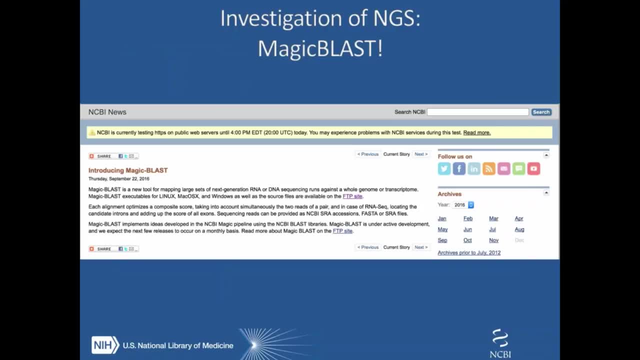 MagicBLAST. This is an NCBI optimized RNA-seq mapper. It works based on BLAST and the default output are SAM files. Once again, if you don't understand the last couple of sentences I said, try to go back through and work yourself through. 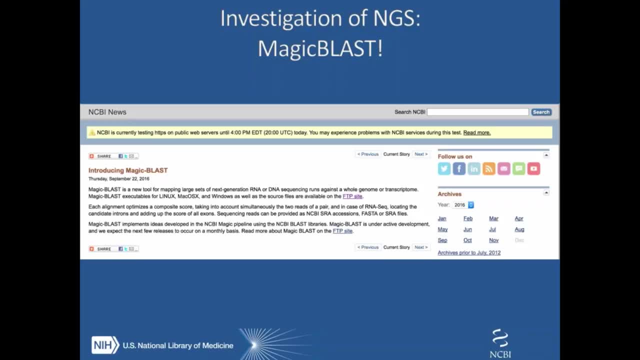 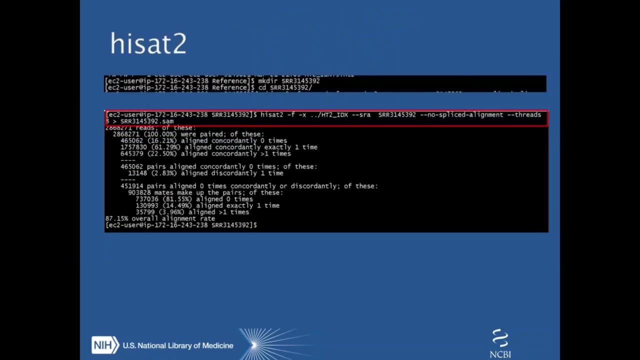 our Next Generation Sequencing Workshop or somebody else's Next Generation Sequencing Workshop, And you'll understand exactly what I mean when I say that You can grab this as a binary from our FTP site Also, HiSat, which is a very fast 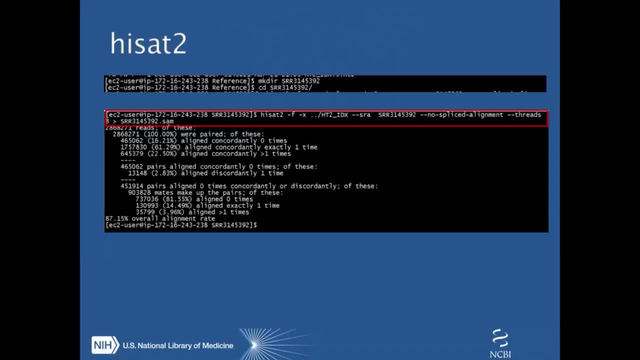 mapper, which happens to be written by the Salzburg group at Johns Hopkins University. Not an endorsement, but it does work natively with SRA. I'm excited to say that pretty soon. STAR, which is another very popular fast RNA-seq mapper. 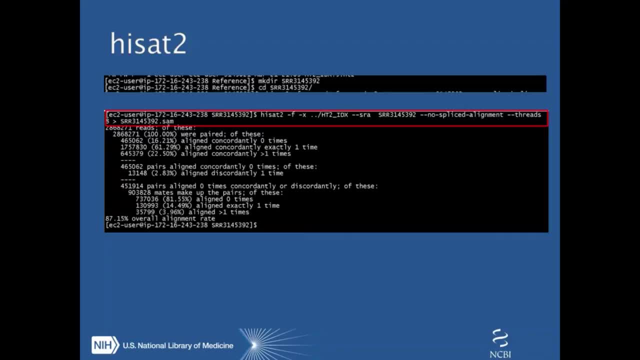 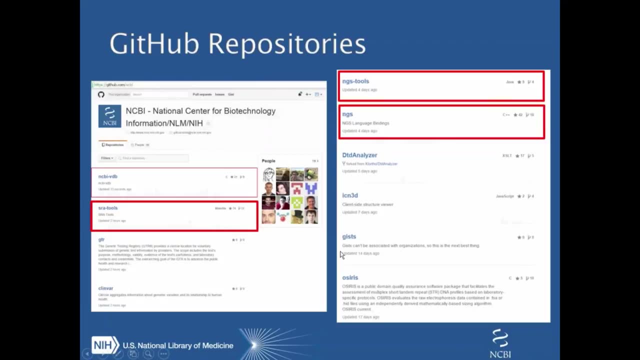 developed at Cold Spring Harbor Labs should also work natively with SRA. To find the SRA toolkit, you can grab it from GitHub. If you're not familiar with GitHub, that's okay. I'd encourage you. in my personal opinion, 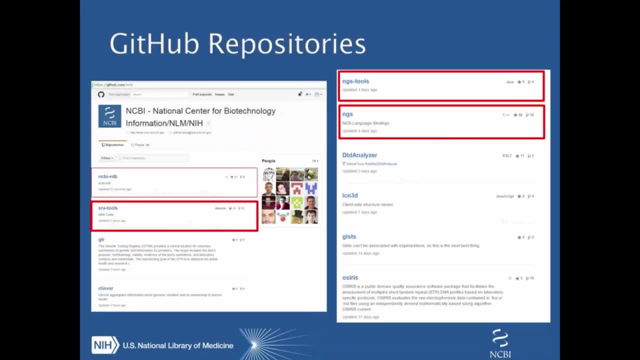 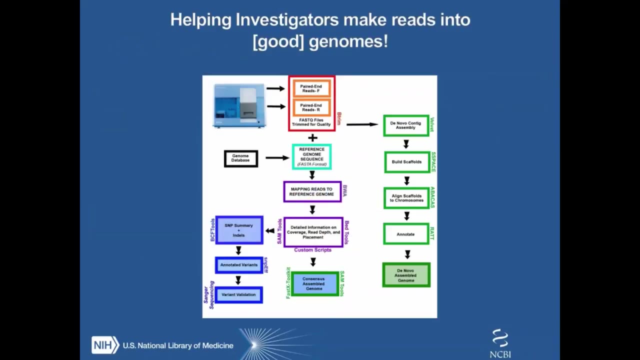 again, Software Carpentry is an excellent resource for checking these things out. If you are a tool developer, check out the NGS language bindings and you can make your tool work natively with the SRA datasets. So I had a lot of questions while Peter was. 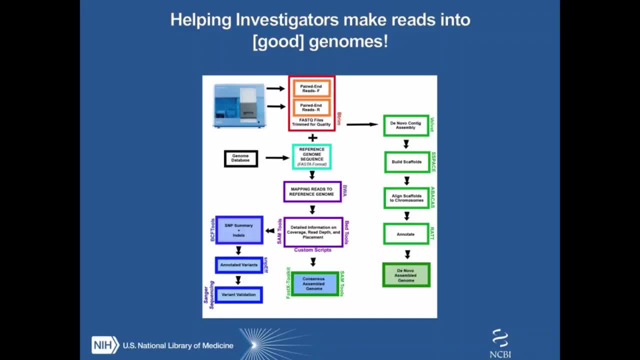 talking about genome annotation and so I actually want to talk about that a little bit. I think it segues well, I'm going to sort of switch off the genomics. Say you had an assembled sequence and you wanted annotation. Now, if you happen, 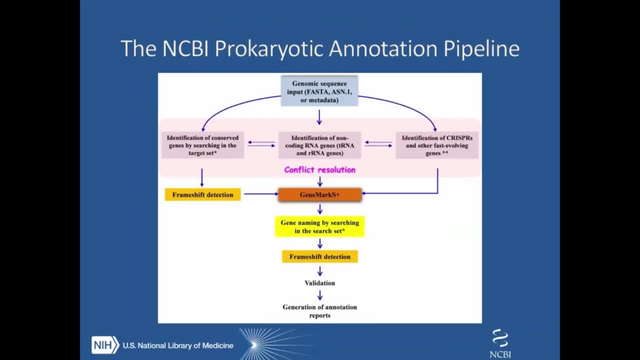 to work on bacteria. that is done automatically. So every bacterial sequence submitted to NCBI gets annotated by our prokaryotic annotation pipeline And you'll see if there are original submitters annotations. they're in the GenBank FTP file of the assembly database. 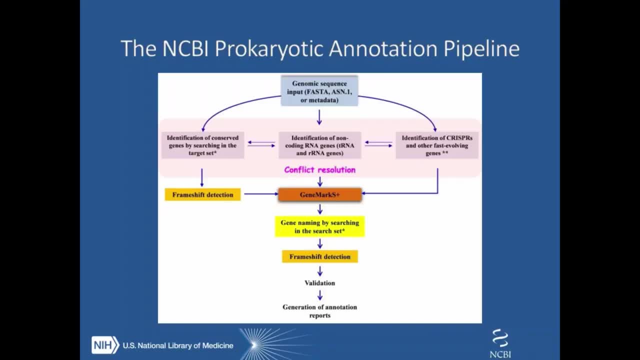 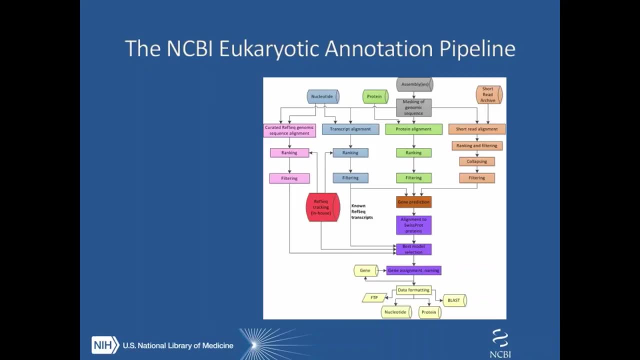 and our annotations will be in the RefSeq file For eukaryotes. not all organisms are automatically annotated by our pipeline but if you're interested in having your organism annotated, if you've done an assembly and you're submitting it. 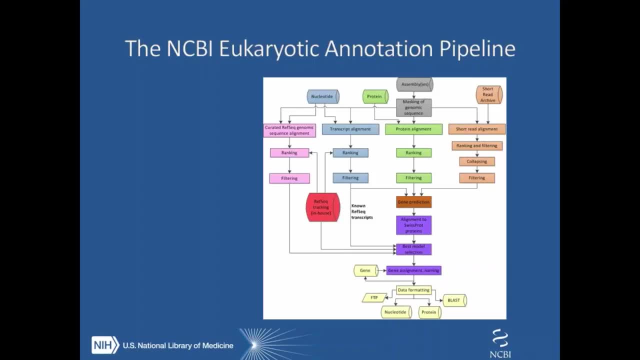 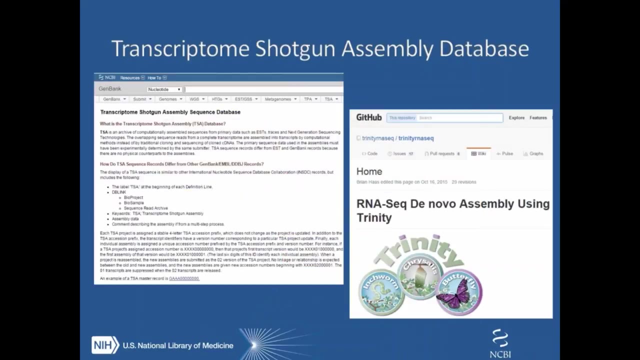 please write an email to genomes at ncbinlmnihgov If you need that information. again, you can go ahead and email us at webinars at ncbinlmnihgov. For organisms where there is not a good reference sequence- and I know this is true- 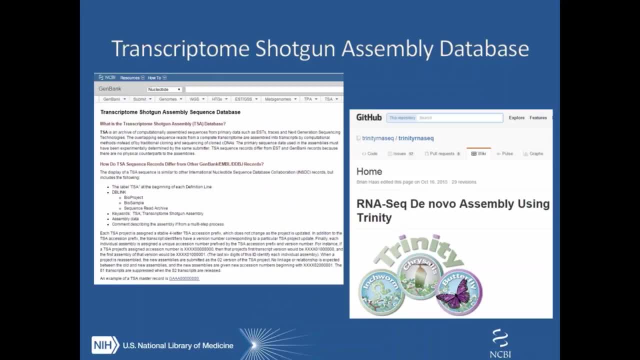 for quite a few agricultural organisms. you might check out the transcriptome shotgun assembly database. There are millions of assembled sequences in there at this point- And this is something that's very exciting to me- Maybe you have a strange organism which doesn't have a reference, or it has high GC. 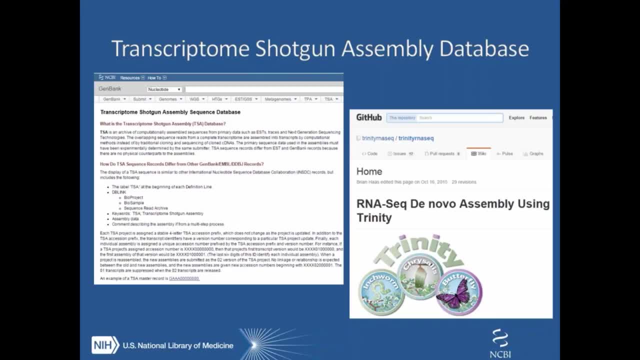 content or there's a lot of repeated elements, You can still most likely find assembled RNA in this database and do the work that you need to do. So I think that's something that's very helpful to the community, And if you're. 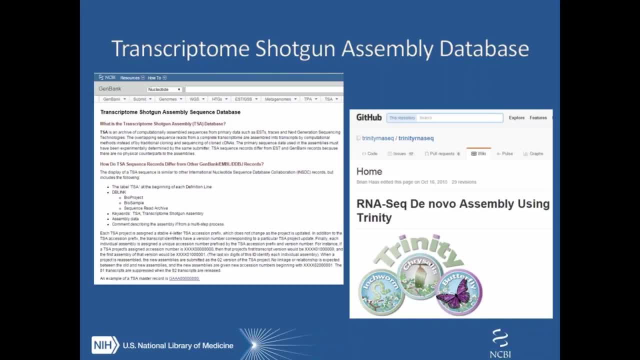 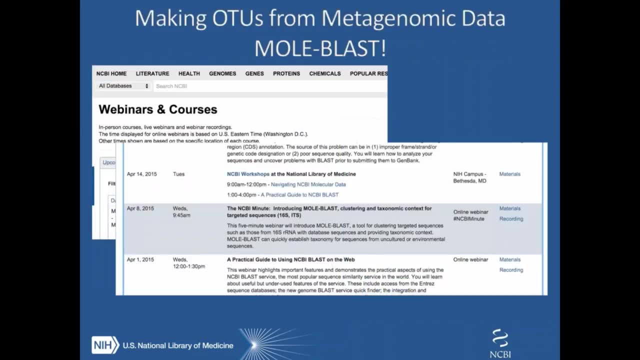 doing RNA assembly yourself, please consider submitting to this particular database. Once again, I think this database is very helpful to the community. Finally, we have a tool called Molblast. If you're just getting into the metagenomic space, you can use this. 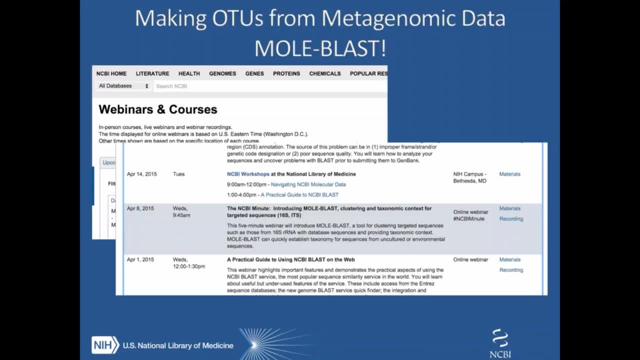 particularly for things like 16S, to go ahead and make operational taxonomic units, In other words, clusters of the sequences you're seeing in your metagenomic sample. That said, I want to caution you- and I've talked to community members about this- 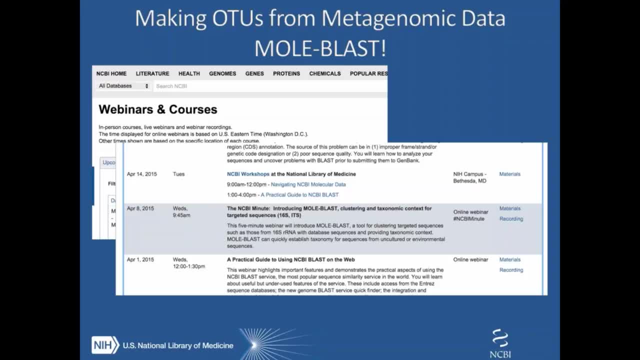 this is a very approximate tool, Really appropriate for first-pass analysis. If you need to do deeper analysis, please do some research on metagenomic tools that make more refined OTUs So to get more information. as I've mentioned a couple of, 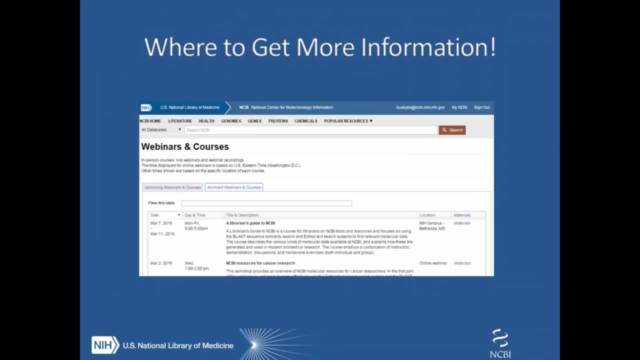 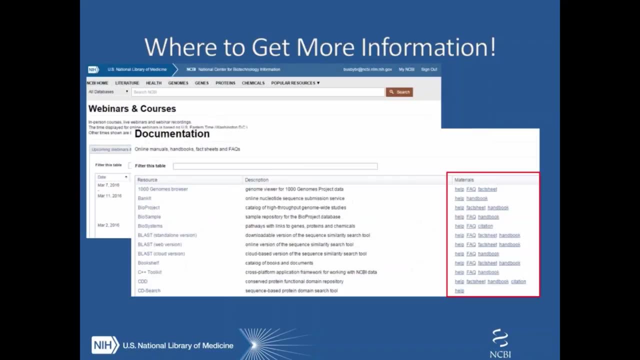 times. one quick way is to search webinars and courses and there's a very, very fast search very easy to use. search here on our webinars page And also if you go into our documentation from the NCBI Learn page, pretty much for. 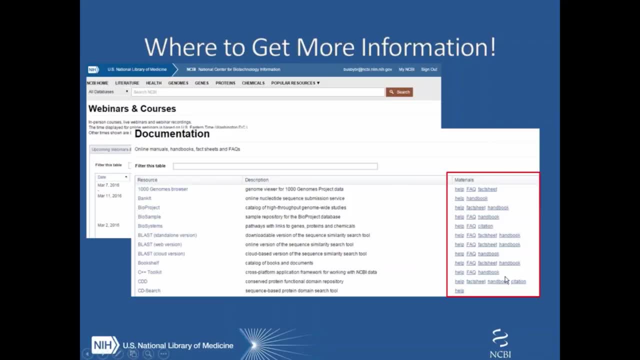 every single one of our resources. there is help and you can get to it. BankIt is our new submission system. It's something that the submission folks are very proud of. I encourage you to take a look at it. As you can see, this is in alphabetical order. 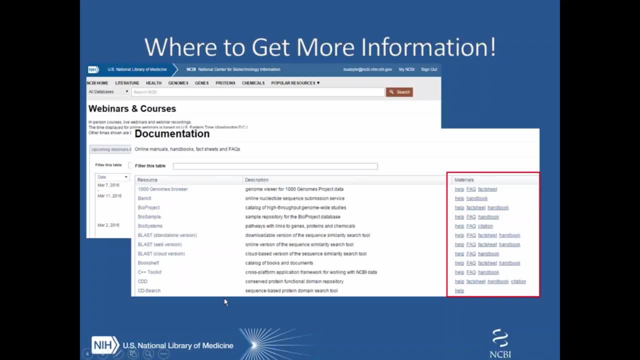 so you can go look in many, many other things. So, that said, I am sure there are a number of questions. I see Peter Cooper across the table from me typing relatively furiously. We have about five minutes to take questions and then we're going to have to go ahead and 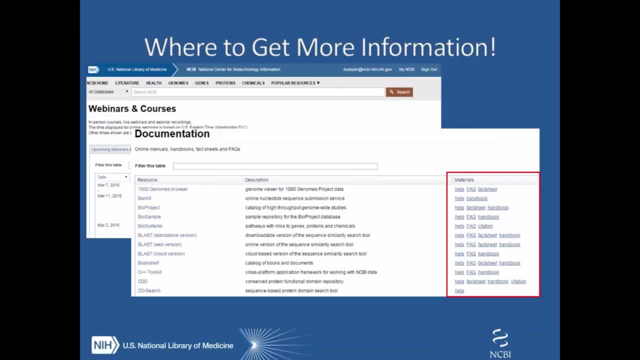 hang up the webinar. That said, if your question is not answered and you have a substantive question that's hanging out there- we'll try to get it up on the FTP site in the next couple of days. So check back here and we'll try to go ahead. 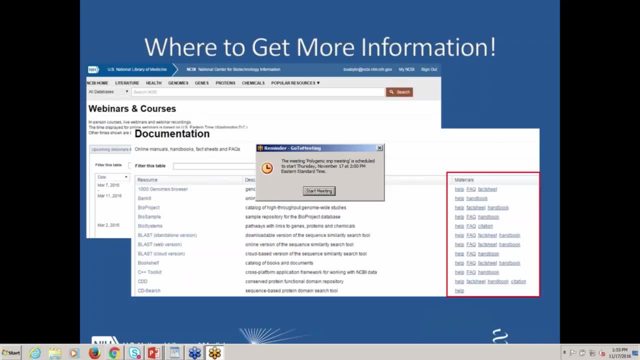 and answer your question. GoToMeeting is telling me it's time for the next meeting but, like I said, we're going to take questions for about five minutes. There will be a little bit of background noise. I'm going to hand this microphone to Peter. 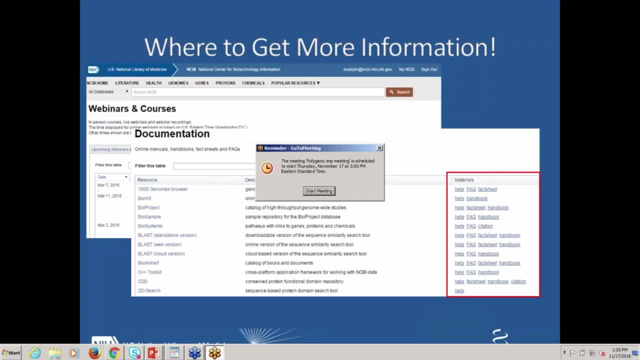 Cooper and for widely applicable substantive questions. he's going to ask the question and then either answer it himself or I'm going to go ahead and answer it. I think we have time for one or two questions, Alright, so I guess Peter has. 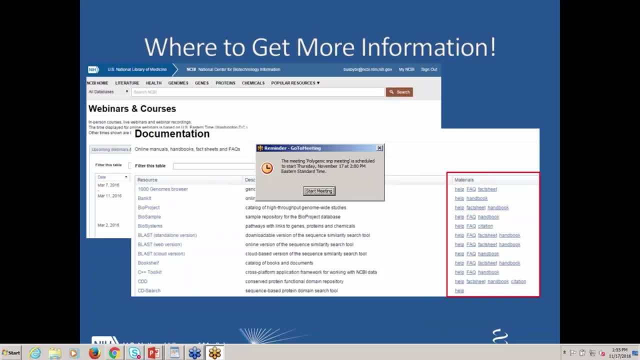 answered pretty much all of your questions, as far as I know. If you have more questions, if questions occur to you later on, no problem. Please just go ahead and ping webinars at ncbinlmnihgov or info, info, info at ncbinlmnihgov. 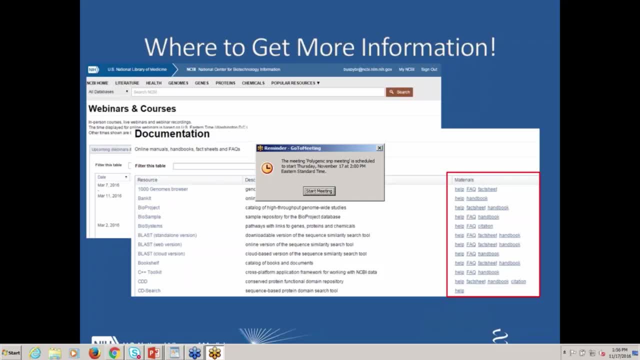 I really hope this has been an informative and worthwhile hour for you. Also, if you have ideas on other webinars or would like more explanation on any particular resources that we outlined in this webinar, please also send an email to webinars at ncbinlmnihgov. 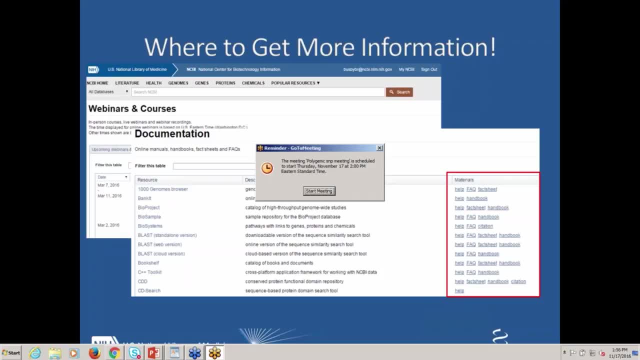 With that, I hope you all have a fantastic day. For those of you in the United States, Happy Thanksgiving and take care.